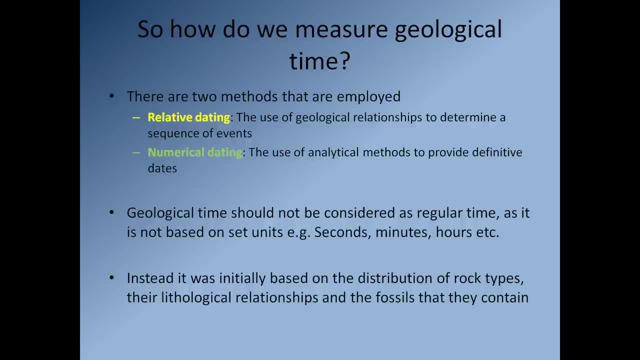 simply says this is the position of this layer of rock within a sequence of rocks. So geologic time should not be considered as regular time, as it's not based on seconds, minutes, hours, etc. Instead, it was initially based on the distribution of rock types. 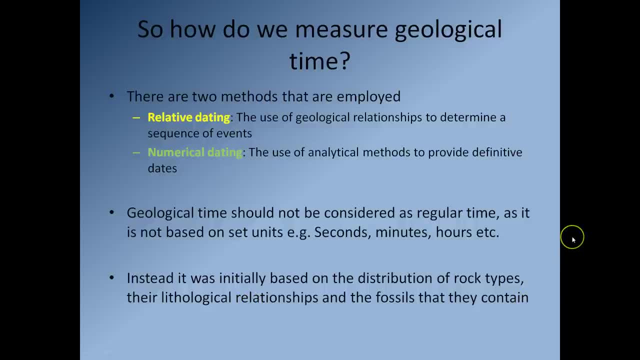 their lithological relationships and the fossils they contain. So when we look at the geologic time scale and you see the boundaries between the areas, the eons, the periods, the epochs and the ages, essentially what those boundaries represent is either, you know, the first or last appearance of certain fossils, or the first or last appearance. 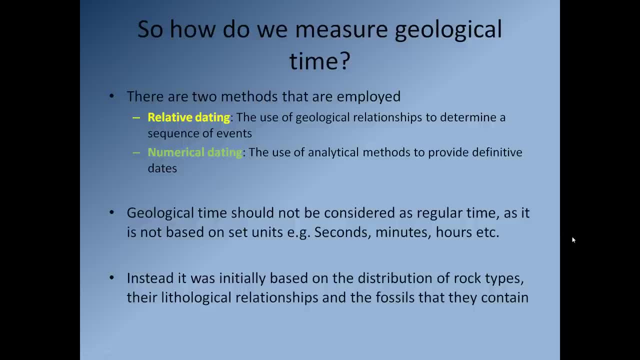 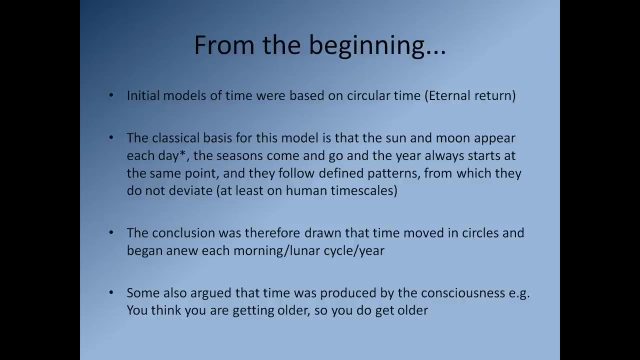 of certain rock types. So those boundaries aren't actually defined by a numerical value, and so that's why geologic time differs from, you know, time in the regular sense. Okay, so let's go all the way back to the beginning. let's think about you know how humans initially began to. 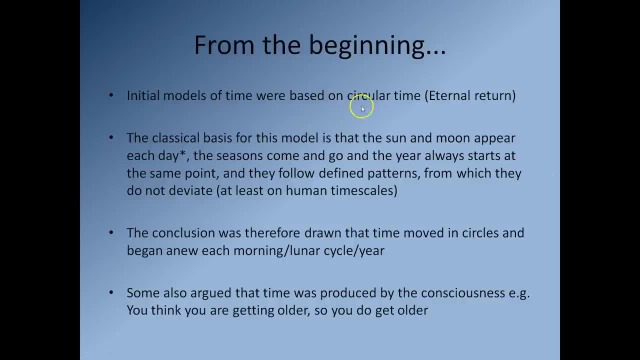 think about time. So initial models were based on what's called circular time, or also referred to as eternal return, and this is a classical model, and the basis for the model is that the sun and the moon appear each day, the seasons come and go, the year always starts at the same point, and so, essentially, 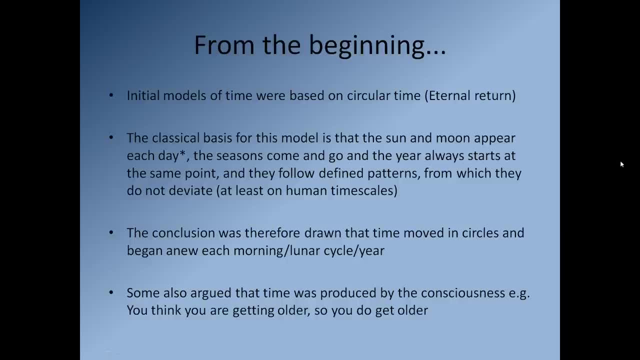 you know, time seems to follow these, you know, cyclical repeating patterns, and these patterns don't deviate, or at least they don't deviate, on a human time scale. So the conclusion was therefore drawn that time at the time moved in circles and it began anew each morning or the start of each lunar cycle. 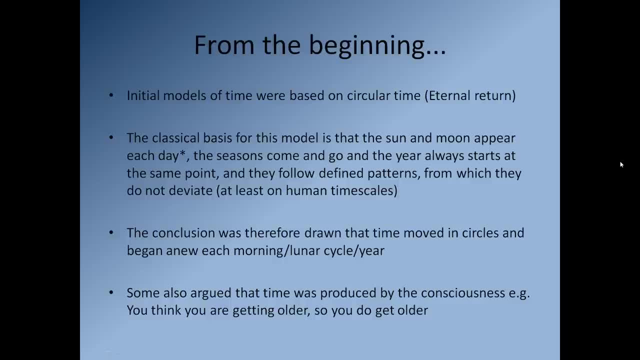 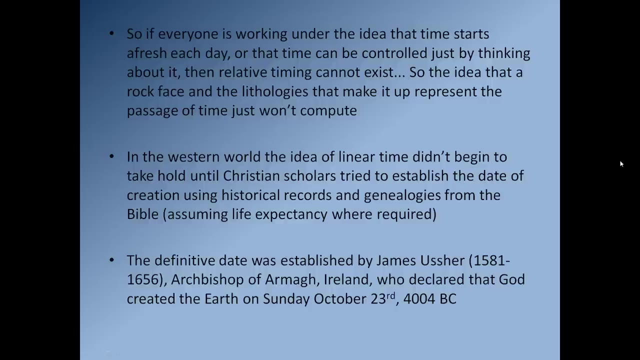 or at the start of each year. So some other people also argued that time was produced by the consciousness. so essentially, if you think you're getting older, you get older. if you think you're getting younger, in theory you should get younger. So if everyone is working under the idea that, 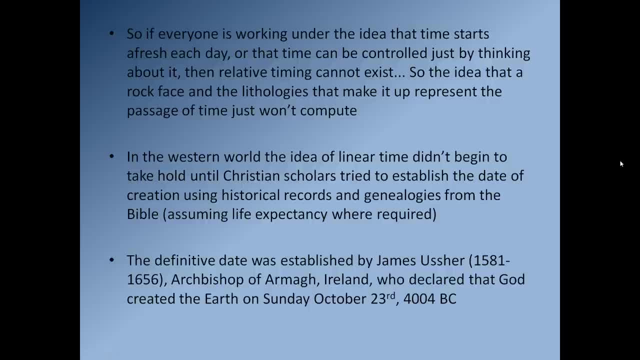 time starts afresh each day, or that time can be controlled by thinking about it, then relative timing cannot exist. So the idea that a rock face and the lithologies that make up that rock face represent the passage of time just doesn't compute, because you know if you're working. 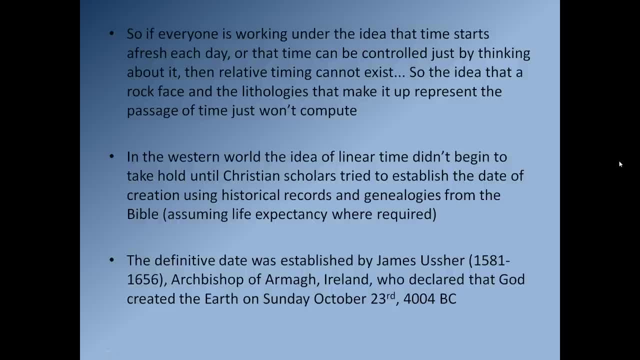 under the idea that the rock face is made afresh each day. it doesn't really matter what the rock face is made up from. So in the western world the idea of linear time didn't begin to take hold until the Christian scholars tried to establish the date of the creation using historical records. 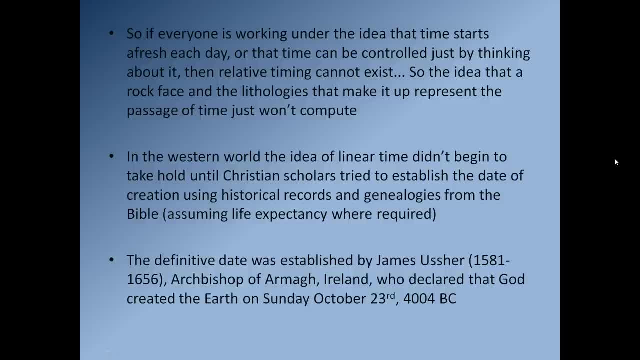 and genealogies from the bible. So in some places they had to assume life expectancies for some people who are in the biblical text. So the definitive date was established by James Usher, who was the Archbishop of Amarr in Ireland, and he declared that God created the earth on Sunday October 23,. 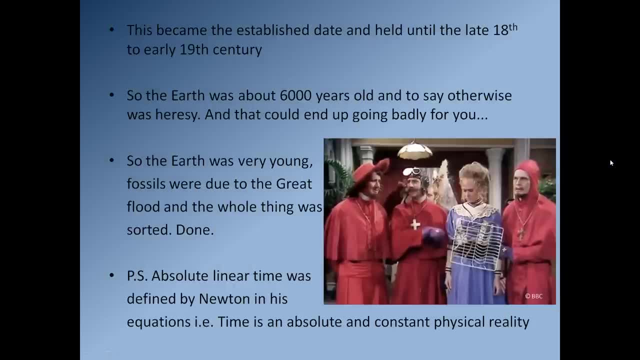 4004 BC. So this became the established date for the creation of the earth and it held until the late 18th century to early 19th century. So that means the earth was about six thousand years old and, and to say otherwise, it was heresy. and you know heresy could end. you, could you know if you uh. 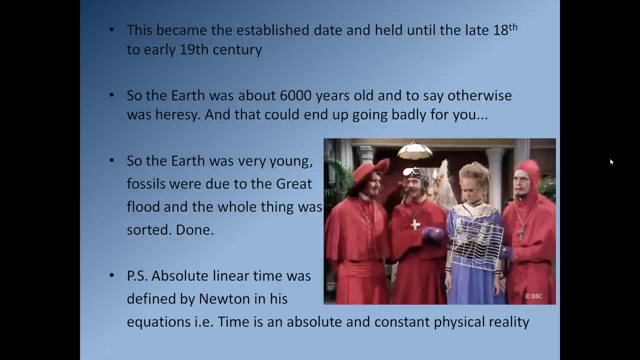 you know, committed a heretical act, you could end up in rather serious trouble. so the earth was very young, fossils were due to the great flood and the whole thing was sorted, done, finished over. a quick side note: uh, absolute linear time was was defined by newton in his 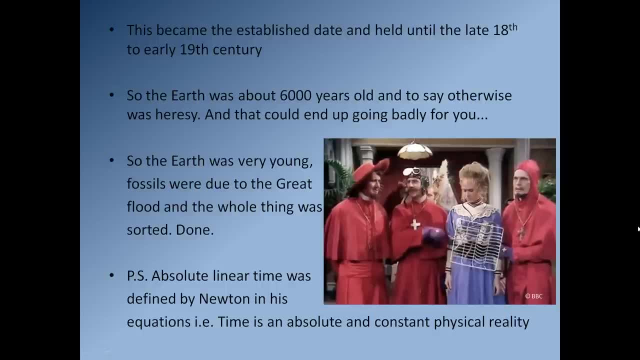 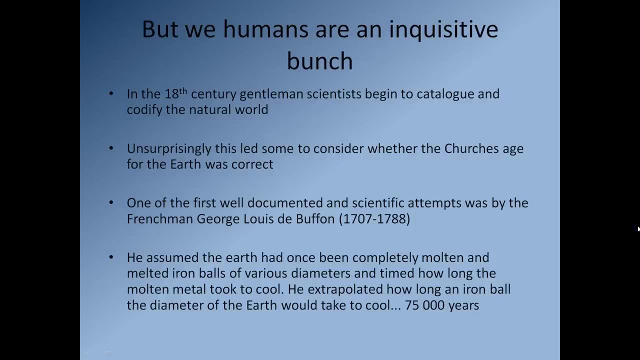 equations. so, uh, time. so he was saying that time is an absolute and constant physical reality. so up until isaac newton we didn't actually think of time in the way that we think of it now. so the problem is, humans are of our inquisitive bunch. so in the 18th century we had a group of 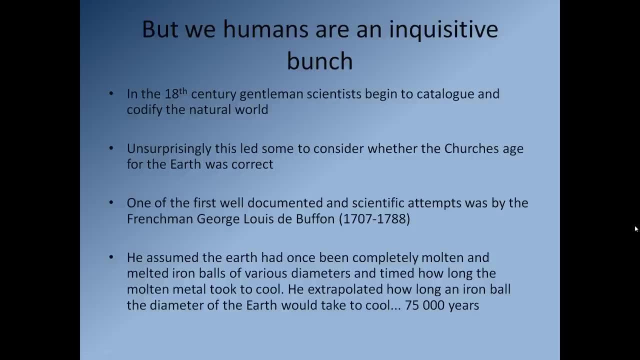 people, especially in western europe, who we generally refer to as gentlemen scientists, and they began to catalogue and codify the natural world. so gentlemen scientists were essentially typically men who were from relatively well-off families, so typically their families owned land and they had a steady income from that land, and so essentially it means they didn't have to, didn't? 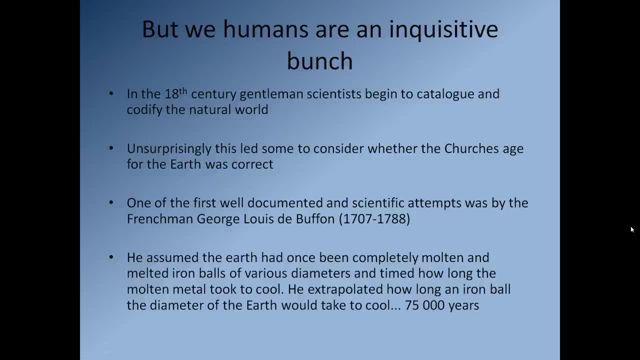 have to work, and so what you have is a lot of very well-educated individuals who need to fill all their free time, and so you know, some of them, you know, took to collecting butterflies, some of them took to collecting plant specimens, and some of them took to looking at rocks and fossils. 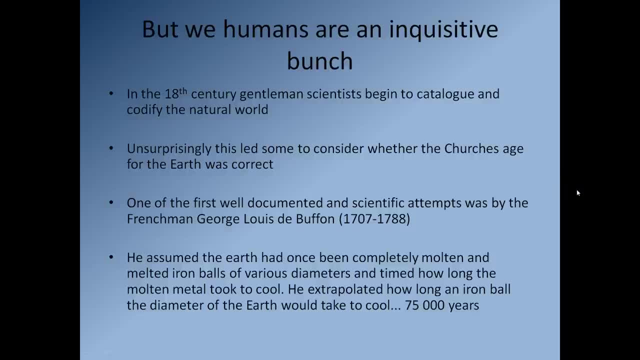 so all these uh, well-educated people began looking at rocks and fossils and they began to think: well, hold on a minute. these rocks and fossils seem to show indications of, you know, having been deposited over long periods of time. so maybe the church's age for the creation of the earth wasn't correct. so one of the first, 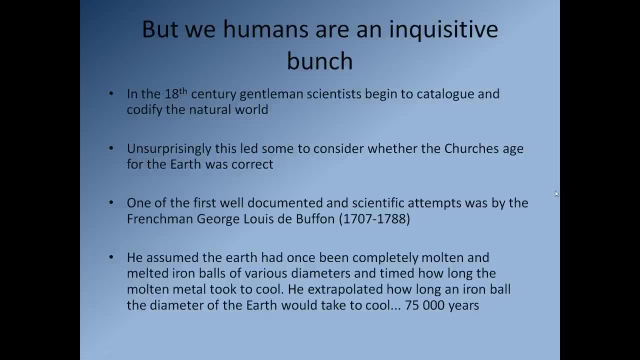 well-documented and scientific attempts to work out the age of the earth was by a gentleman called george louis de buffon, and he assumed the earth had once been completely molten, which he was correct about he did he's. he melted iron balls of various diameters and timed how long the molten metal. 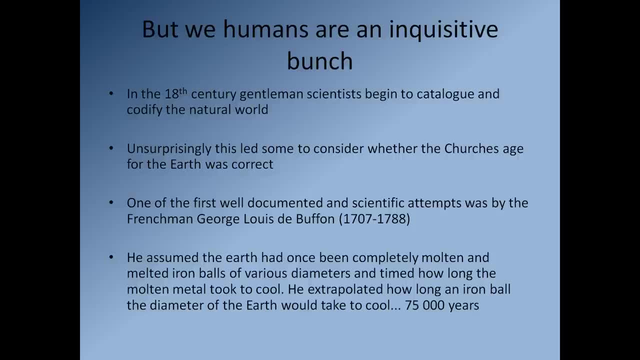 took to cool. so essentially, you know he would melt an iron ball. that's, you know, one inch, then two inches, then three inches, then five inches, then ten inches, and obviously, as the iron ball got larger, yeah, obviously, once he melted it it would take longer for that ball, you know. for the 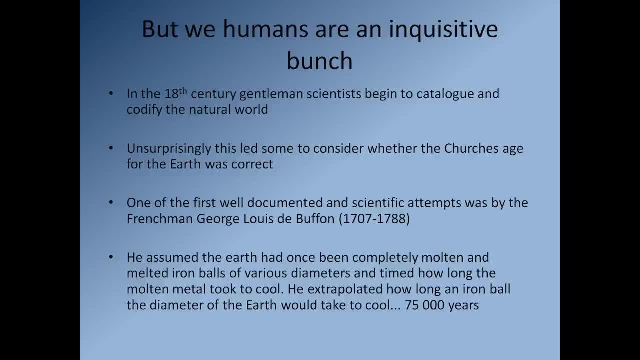 molten iron to cool down and solidify again. so essentially, once he'd done that, he could begin to extrapolate how long it would take an iron ball the diameter of the earth to cool from a completely, and so he came up with a number of a number of 75, 000 years. now we know that number is, you know. 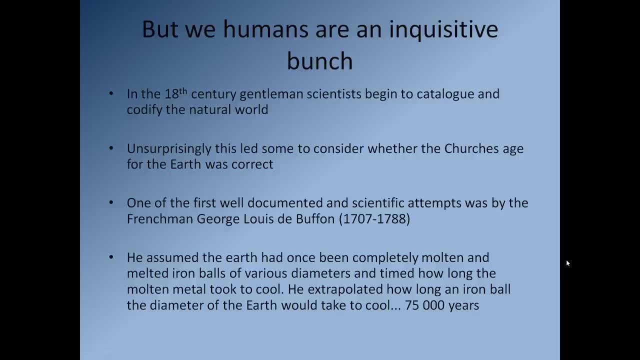 rather, rather wrong. it's a bit, you know, it's considerably too young, but he was trying to do it in a scientific fashion. so, although his result wasn't correct, he was trying to come up with a scientific mechanism that allowed him to try and work out the age of the earth. 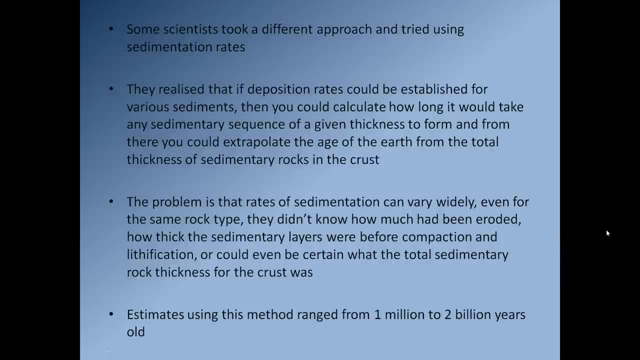 so some scientists took a different approach and tried using sedimentation rates. so some scientists realized that the sedimentary rocks that we see are actually being deposited by sedimentary processes like rivers, for instance. so they realized that if deposition rates could be established for various sediments, then you could calculate how long it would take any sedimentary 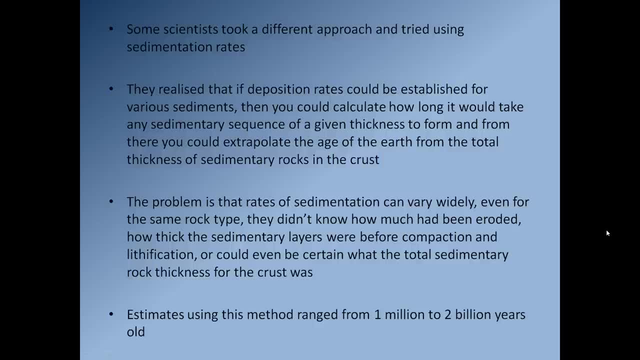 sequence of a given thickness to form, and from there you can extrapolate the age of the earth from the total thickness of sedimentary rocks in the crust. so if you can work out how long each layer of rock in the crust takes to form, well then you. all you have to do is add all those values together and if, voila, you have a value for. 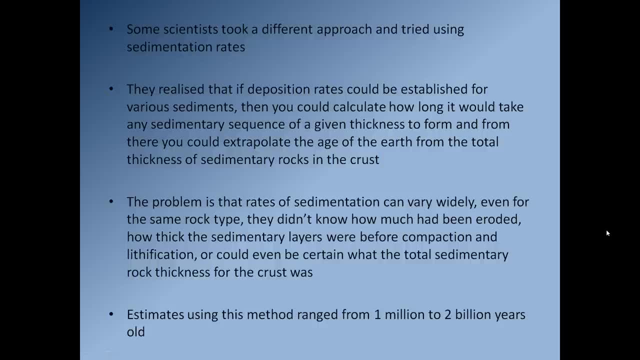 the age of the crust and you can then say that's the age of the earth, and once again, very logical argument. the problem is that rates of sedimentation can vary widely. so some rivers, for instance, will deposit sediment very, very slowly, and some rivers, like the ganges, will deposit sediment at 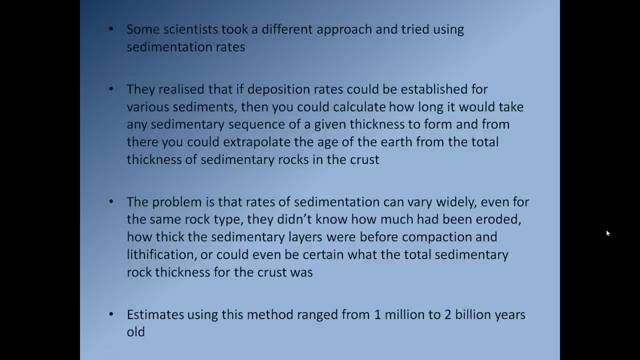 absolutely astronomically high rates. so the question becomes is: do you use a sedimentation rate for a relatively slow river like buffalo bayou, or do you use a sedimentation rate for a big, powerful river like um, like the ganges? so that's your first problem. 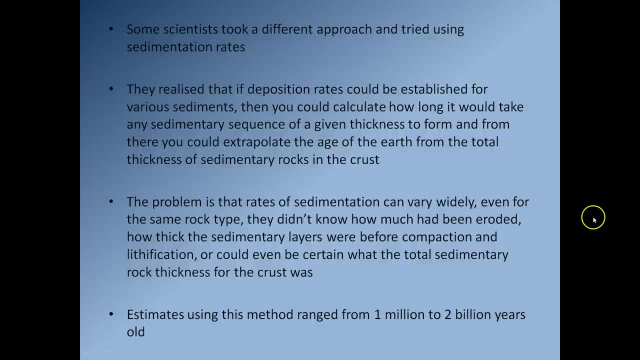 the other. the other problem is you don't know how much sediment has been eroded, so all those sediments being deposited, sediment is also lost, and so you don't know how much sediment has been lost. so you know, maybe you have a layer of sedimentary rock that's one meter thick. 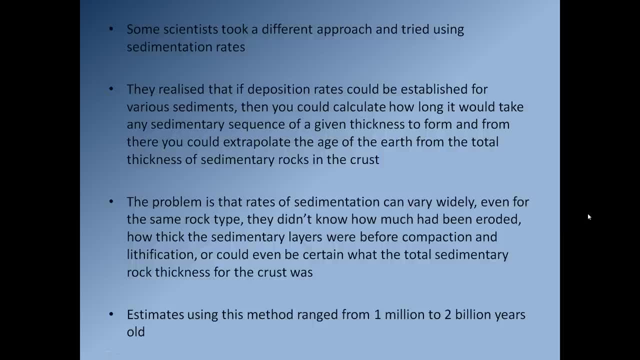 but in reality you know you actually lost two meters from that layer of rock. when it was lost was a sediment. so you know you don't have the original thickness of sediment represented by that layer. next problem is you don't know how thick the sedimentary layers were before they. 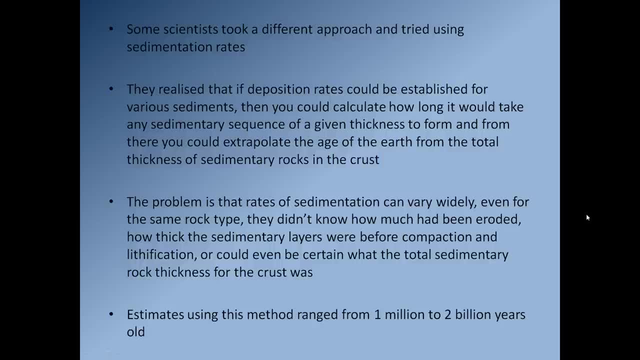 were compacted. in order to take a sediment and turn it into a sedimentary rock, you have to compress the rock, and so that means a sedimentary layer that was five meters thick will be squished and will turn into a sorry. a sediment layer that's five meters thick will be squished and will be. 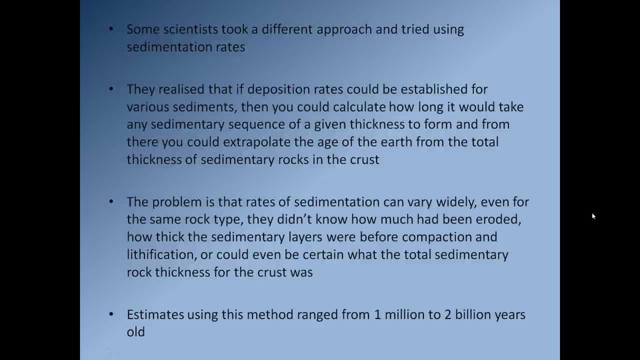 turned into a sedimentary rock that's one meter thick, and of course they didn't take that into. and then the other problem is you can't be certain about the total sedimentary rock thickness for the crust. you know all they could do was that. you know they only had the capacity to look at the 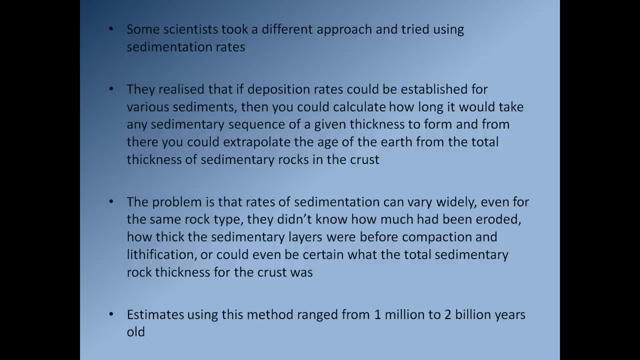 sedimentary rocks that were at the surface of the earth. now we know as geologists that sedimentary rocks go down hundreds of meters under this, under the earth's surface, but these scientists did not have the capacity to drill down and see those layers. so unfortunately it means that because 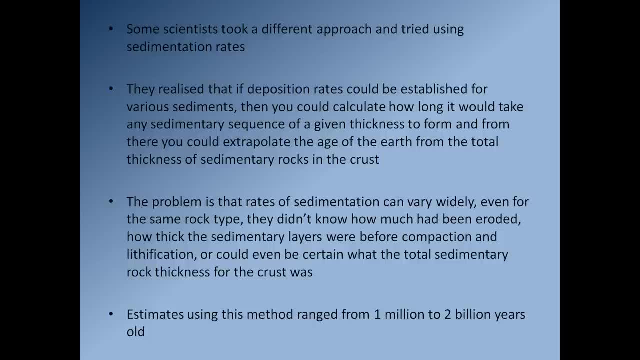 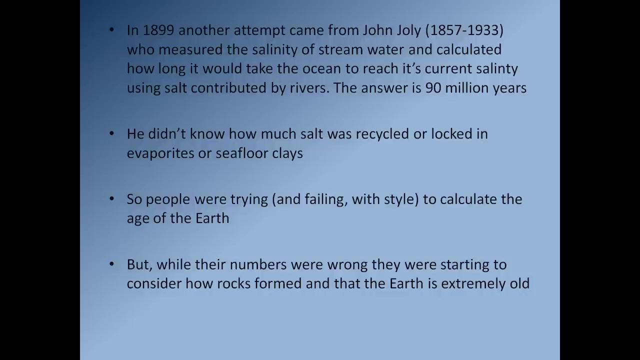 of the vast number of sedimentary rocks that have been formed by the fish we're talking about in the sky. most of them are in the upper reaches of the ocean, and some are in the deep williamson levels as well, and so, if you're looking for하기, 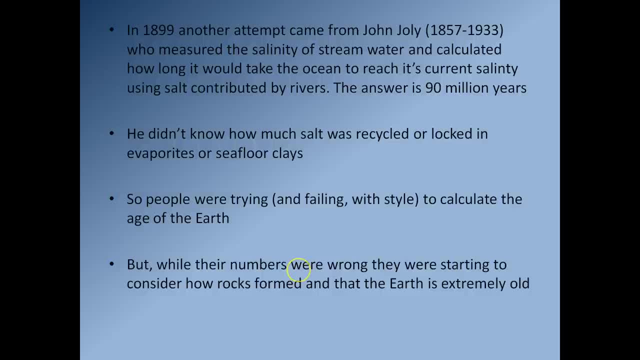 or a good piece of asbestos rock, to take into consideration that you're going to end up with quite a large range of numbers, and so estimates using this method range from about 1 million years to 2 billion years old. so, once again, the values they're coming up with aren't correct, but they are. 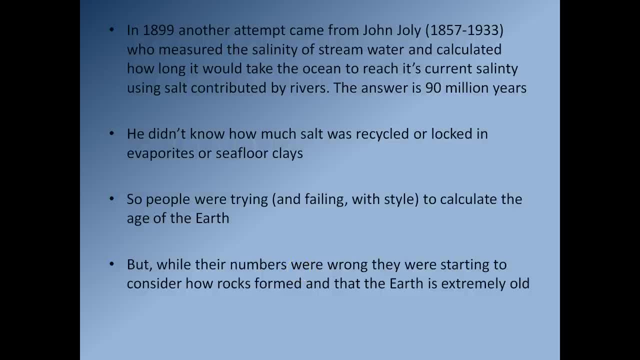 using scientific, logical methods to try and come up with a number. so in 1899 another attempt was made- the salinity of stream water- and calculated how long it would take the oceans to reach its current salinity using salt contributed by rivers. So if you measure the amount of salt there is in the Earth's oceans, 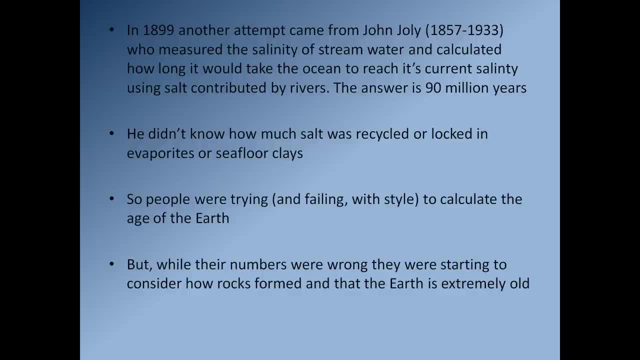 and you say right, this is the salinity of river water, and I know that the river water goes into the oceans. therefore, my assumption is that the salt that's in the oceans is being contributed by the rivers. Therefore, if I know the salinity of the rivers and I know the salinity of the oceans, how long? 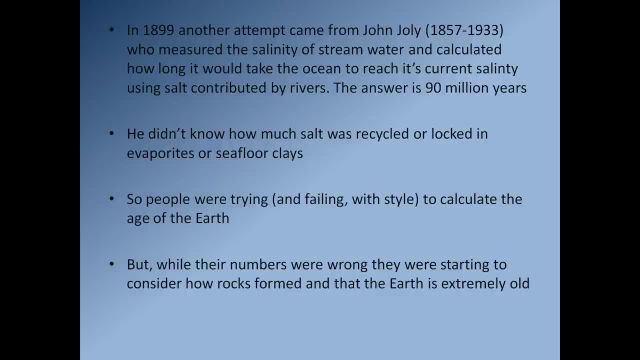 would it take me to reach that ocean salinity if I was just contributing salt from river water? and obviously, as I said, the answer for that is 90 million years. So the problem with John Jolly's attempt was that he didn't know how much salt was being recycled or how much salt was being locked in. 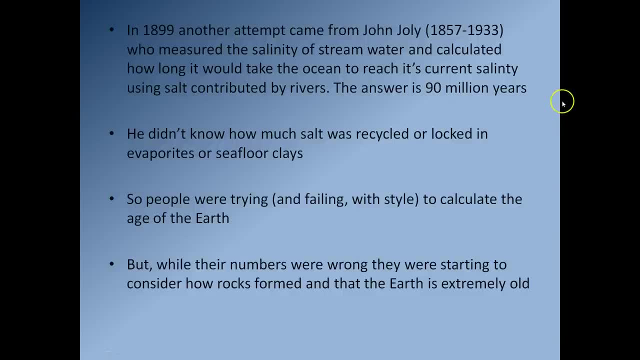 evaporites or in seafloor clays. So once again, his number is much, much smaller than the, the, than the true age of the earth, but nevertheless he was trying to come up with a scientific method to, you know, come up with a calculated age. so people were trying and they were failing with. 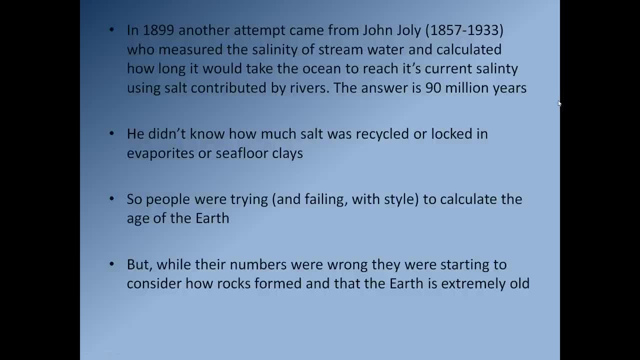 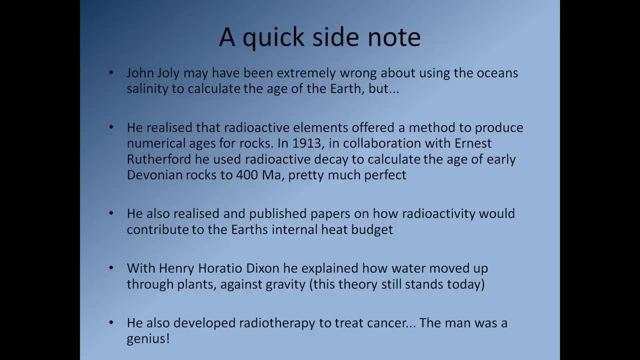 some style to calculate the age of the earth. but while their numbers were wrong, they were starting to consider how rocks formed and that the earth was extremely old. so just a quick side note about John Jolly: so he may have been extremely wrong about using the ocean's salinity to calculate. 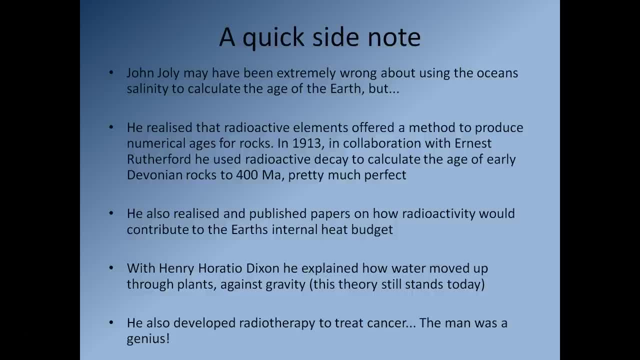 the age of the earth. but he did realize that radioactive elements offered a method to produce numerical ages for rocks. so in 1913, in collaboration with Ernest Rutherford, a well-known New Zealand scientist, he used radioactive decay to calculate the age of the early Devonian rocks. 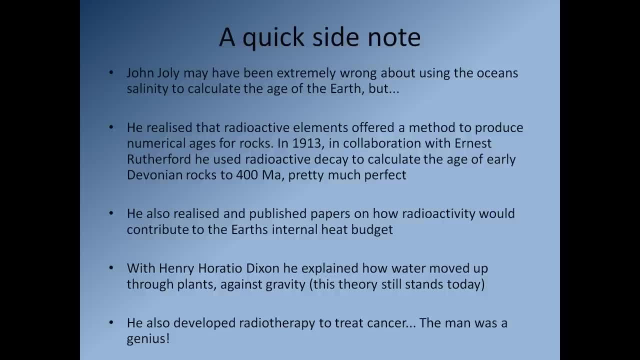 and the age they came up with was 400 million years, which is pretty much perfect. so that was the first time people had used radioactive isotopes within minerals to date- a rock- and we actually going to be discussing this later on when we talk about numerical dating- so he also. he also. 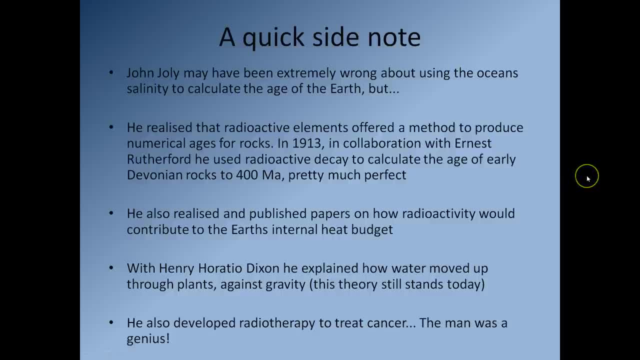 realized and published papers on how radioactivity would contribute to the earth's internal heat budget. so he was one of the first people to realize that these radioactive isotopes occurred inside the earth and that they would help to keep the earth's interior warm. and that's also going to. 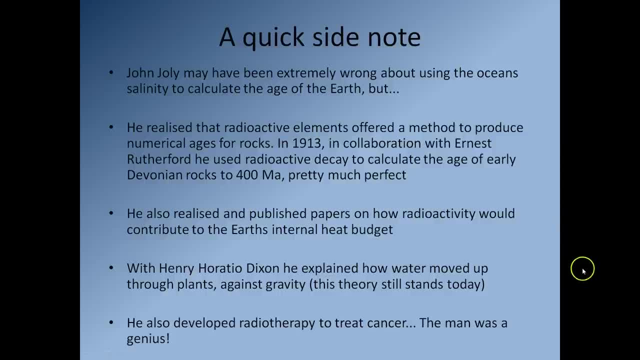 become important in a few slides time. so, with Henry Horatio Dixon, he helped to explain how water moved up from the earth to the earth, and how it moved up from the earth to the earth and how it moved up through plants against gravity. and that theory still stands today. so you might remember. 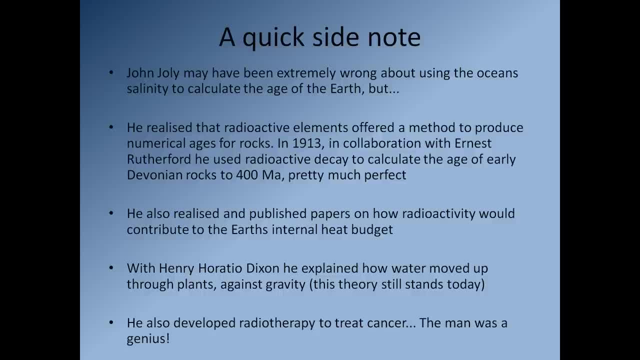 from when you did high school biology, chances are, when you looked at plants, you spoke about xylem and phloem. those are the two types of cells that move water and nutrients up and down the plant. well, that was, you know partially uh come. you know partially uh uh. came up with by, uh, John Jolly. 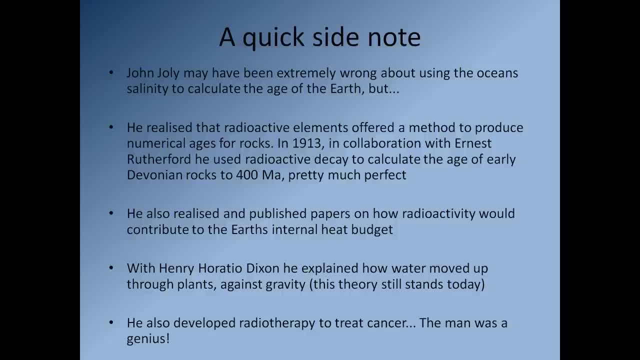 and he also developed radiotherapy to treat cancer. so he would insert little capsules containing radioactive material into cancer cells and he would insert little capsules into cancer cells and into cancerous tumors and the radioactivity would destroy the cancerous cells. so you know, the man was, you know, obviously very, very intelligent. so you know he might have been wrong about the. 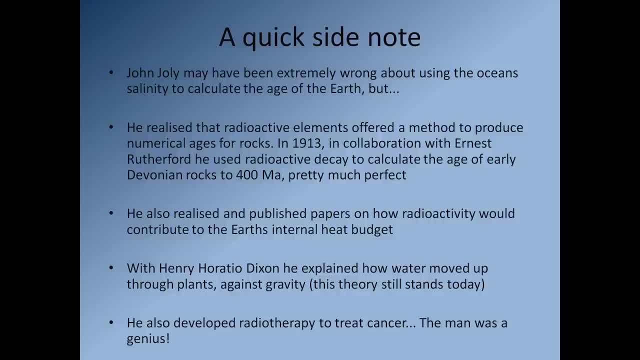 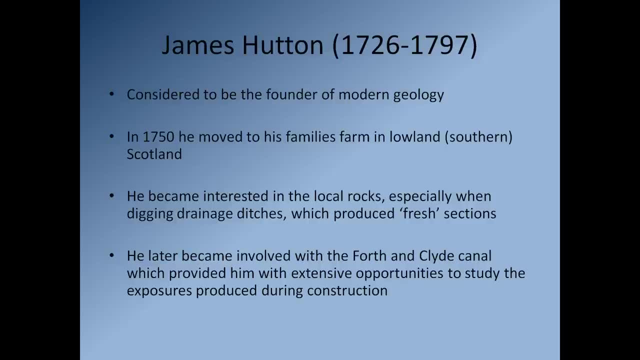 salinity of the oceans, but in in other, you know, parts of his life, the man was a complete genius. so this brings us on to James Hutton. so James Hutton is considered to be the founder of modern geology. so in 1750 he moved to his family's farm in Lowlands, that's southern Scotland. and once again, 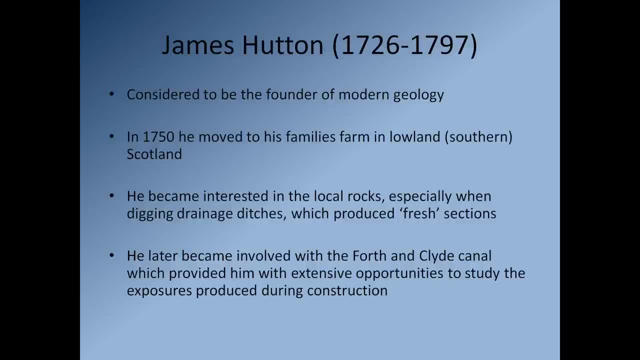 he was one of these gentlemen who was a very important person to him, and he was a very important gentleman, scientist. they had some land there, the family got their income from the land, and so essentially he didn't really have to work and so he had lots and lots of free time to fill. 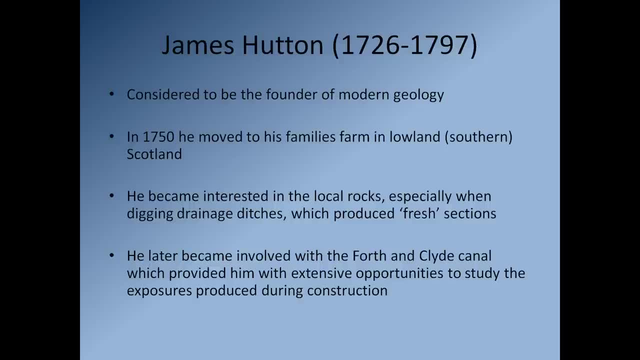 so what he did is he became interested in the local rocks and especially, uh, he became ultra interested when he when he got people to dig drainage ditches. so one of the things he did was he realized that his family's farmland could be improved if they were to drain the land more. 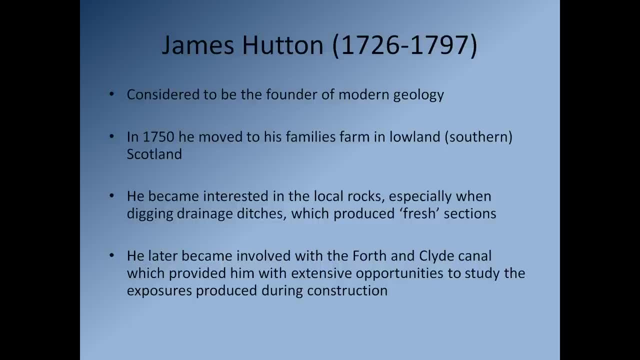 efficiently, and so he had workmen dig some very large ditches for him to help, you know, move the water away. now, in the process of digging these ditches, they obviously had to cut through rocks, and as they cut through rocks, essentially what they did is they produce what we refer to as 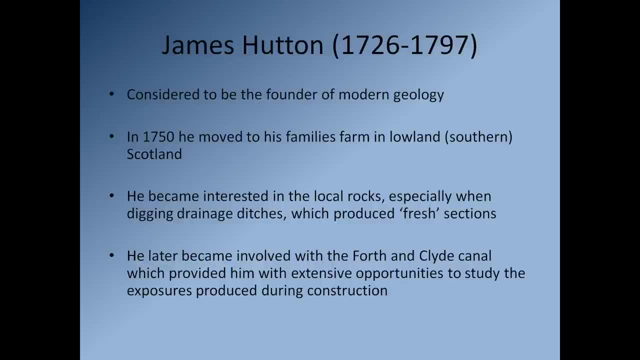 fresh sections. those are areas of completely new, clean, exposed rock where you can really see the relationships between the layers of rock. you know, in the face you've just cut and so, uh, you know that offered him a way of viewing, you know, the rock relationships in very, very high levels of. 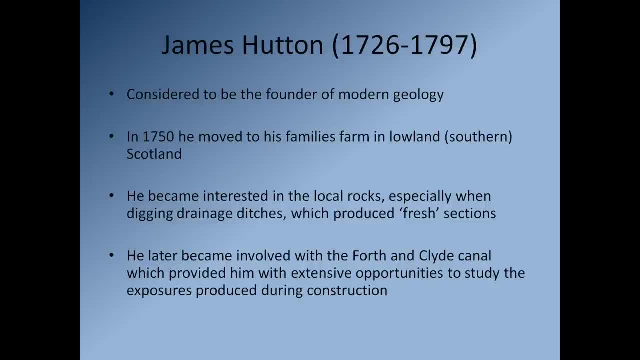 detail. he later became involved with the work of James Hutton who was the founder of the Forth and Clyde canal and that was up in western Scotland and once again, you know, you might or might not know- canals were a method of. essentially, canals are artificial rivers and they were used. 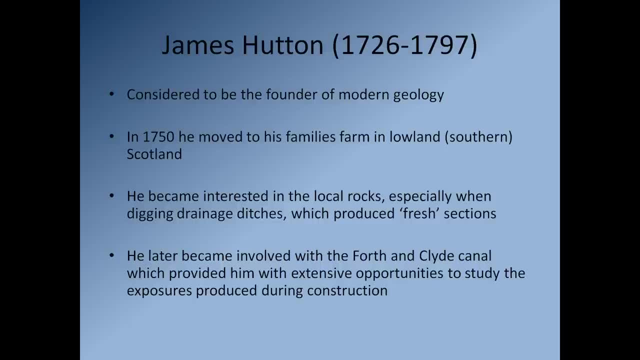 to move coal from, you know, one city to another. and, uh, because obviously you know, movement by road at that point was, you know, impossible for very, very large quantities of coal. so it can only be moved by water, and so canals, as you will obviously expect, obviously have to be quite big, and they're 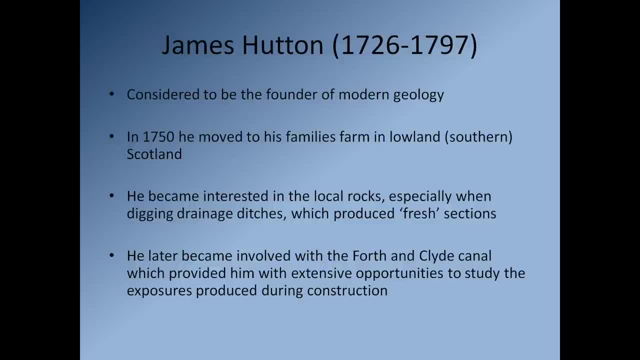 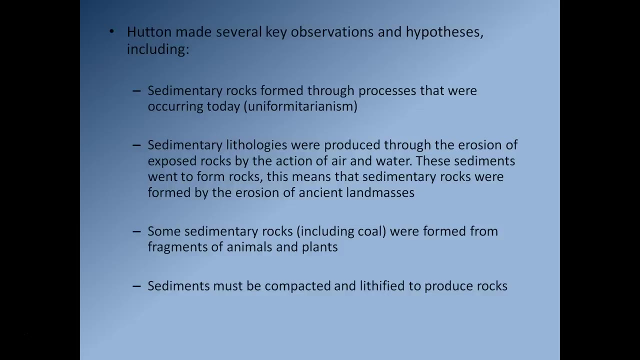 quite deep and so once again, when they're- you know, making this canal, they're going to have to cut through large quantities of rock, and once again that meant they produced extensive and large fresh sections where Hutton could look at the rocks. so Hutton made several key observations. 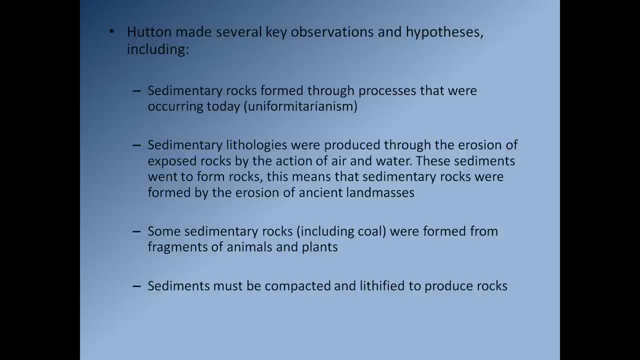 and hypotheses, including number one: sedimentary rocks formed through the pros. sorry, let me try that one again. sedimentary rocks formed through processes that were occurring today. so that's the principle of uniformitarianism: if it's happening now, it's happening in the future, it's happening in the past. so what he realized was, when he looked at some sedimentary rocks, he 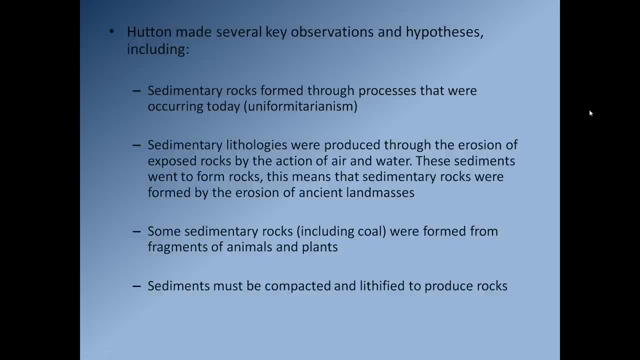 would see structures in those sedimentary rocks that were forming in modern environments. so he'd see things like ripples and burrows and mud cracks. he also realized that sedimentary lithologies were produced through the erosion of exposed rocks by the action of air and water. so he realized that. 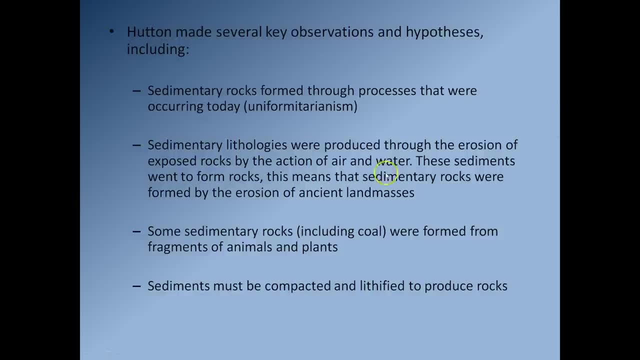 when a rock comes above sea level, it gets exposed to, you know, the action of air and water, and that causes the rock to weather to break down. bits of it will fall off. those bits will get transported and as they're transported they'll be, they'll be eroded and they'll move. you know, they'll change from big class into small. 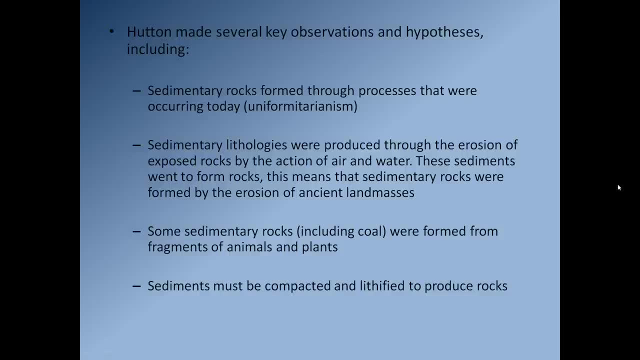 class and those pieces will get incorporated into sedimentary rocks. so what this means is is that the sedimentary rocks he looks at when he goes up to a cliff face were formed by the erosion of ancient land masses. he also realized that some sedimentary rocks, including coal, were formed from fragments of 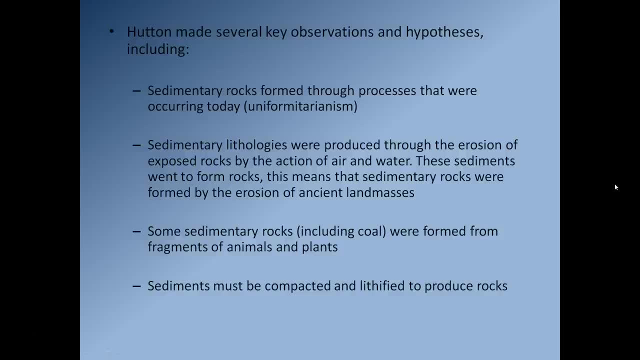 animals and plants. so, once again, that's extremely important, you know. so, in order to build up a very, very thick layer of coal, it obviously takes a lot of organic material. so you know, a coal bed takes a very, very long time to build up. so he realized that the sediments must be compacted and lithified. 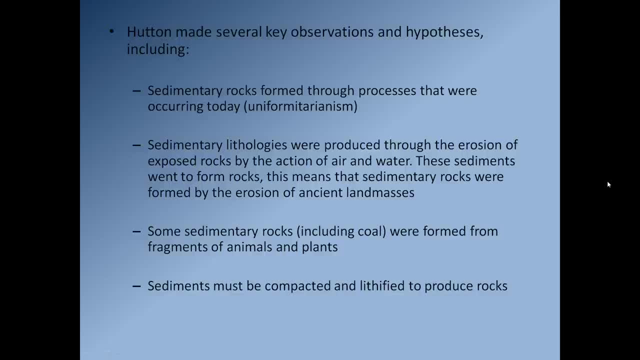 to produce rocks. so he realized that those people that have been trying to calculate the age of the earth using the thickness of sedimentary layers had a bit of a problem because they had no idea of how thick the original layer of sediment would have been before they could make a sedimentary rock. 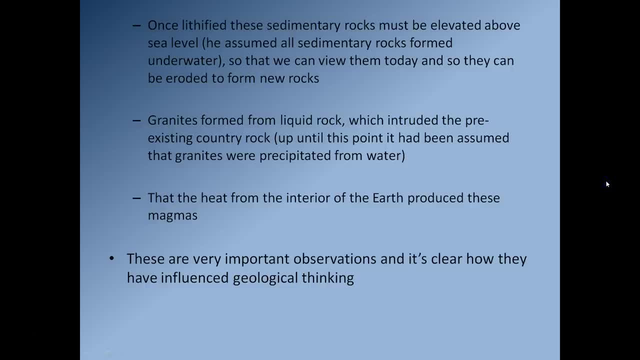 it was compacted to form a sedimentary rock. Here he also realised that once lithified, these sedimentary rocks must be elevated above sea level so that they can be viewed today and so they can be eroded to form new rocks. So in his model, 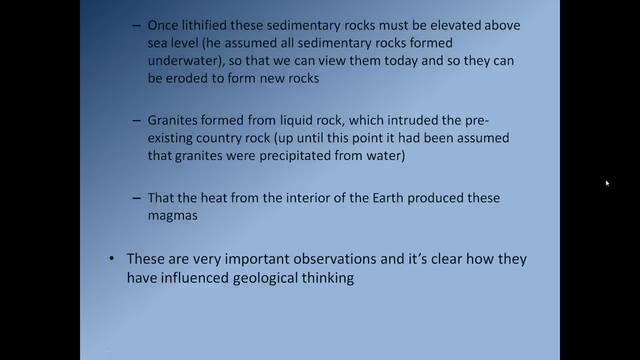 he assumed that all sedimentary rocks were created underwater, so therefore they had to form below sea level and therefore, for all those rocks to be exposed, they had to be lifted above sea level. So, essentially, he's realised that, you know, layers of rock are deposited and then they have to be. 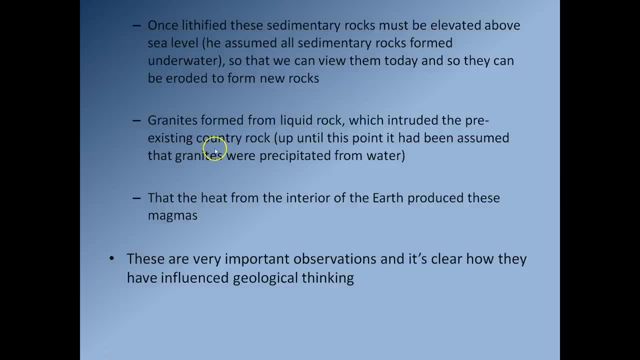 tectonically moved to get them above sea level. He realised that granites form from liquid rock. so he realised that granites form from magma, and he realised that this magma intruded pre-existing what referred to as country rocks, the rocks that were there originally and up until that point it had been assumed. 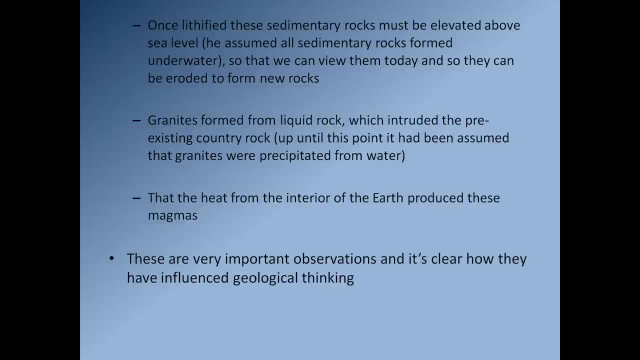 that granites were actually the result of minerals precipitated from water underground. So you know quite a big leap there. And he realised that the heat from the interior of the earth produced these magma. so he realised that the only way to really melt large quantities of rock 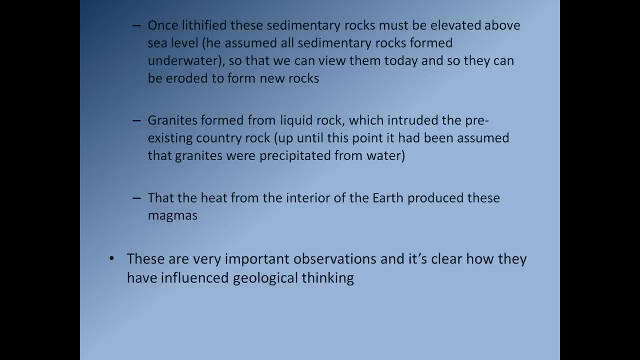 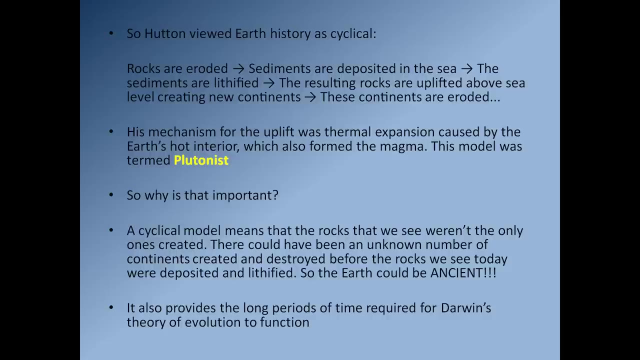 was due to know the heat of the interior of the earth. So these are very important observations and it's clear how they've influenced geologic thinking all the way through to the present day. So these are some of the basic founding principles of modern geology. So what Hutton did is he viewed the earth as cyclical. 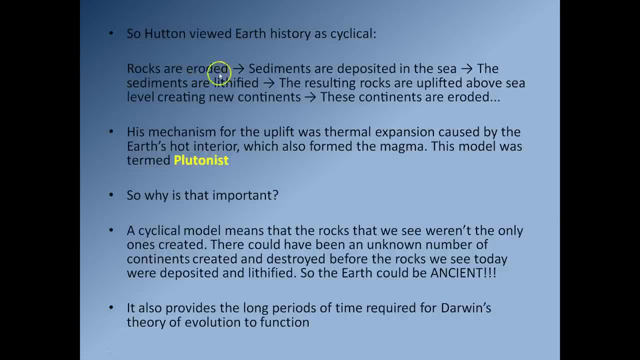 So essentially, his model says that rocks are eroded. from those eroded rocks you get sediments that deposited in the sea. The sediments are then lithithed and turn into a sedimentary rock. the resulting rocks are uplifted above sea level, creating new continents. And these continents were eroded, producing new. 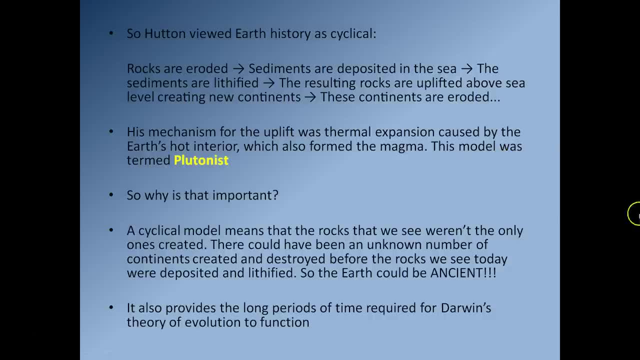 sediments that then go into the sea to produce new layers of rock etc. So essentially you have this rock cycle And his method for uplift was thermal expansion caused by the earth's hot interior. So he said that in some places in the earth the mantle underneath the crust got very, very hot. 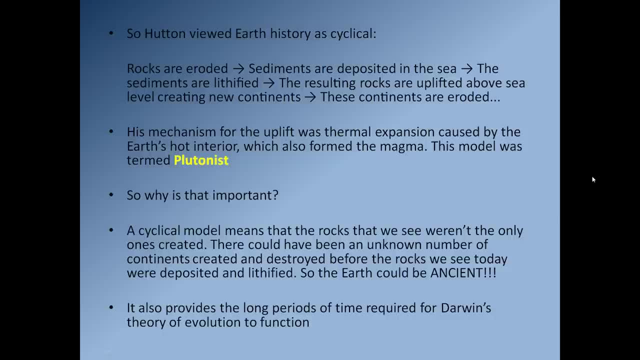 and because it got very, very hot, it became less dense and that area of mantle would rise and so it would push up the area of crust directly above it, pushing it above sea level, And that model was referred to as Plutonist. So why is this important? What's so important about this? 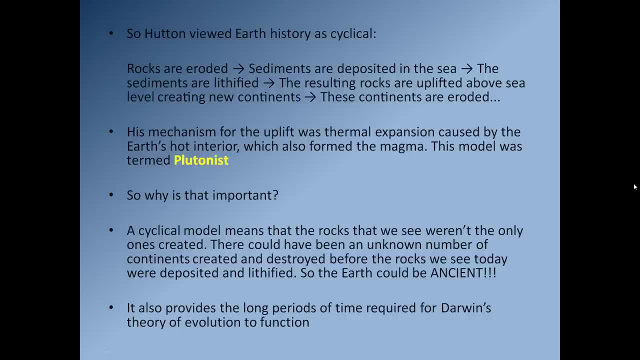 Well, a cyclical model means that the rocks we see weren't the only ones created, So there could have been an unknown number of continents created and destroyed before the rocks we see today were deposited and lithified. So if you use Hutton's model, it suddenly means the earth could be absolutely ancient. 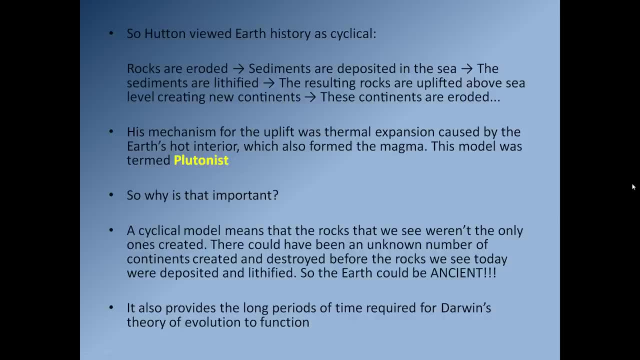 You know, not a few million years, it could be billions of years old. So the other thing it did is it also provided the long periods of time required for Darwin's theory of evolution to function, because evolution does not happen quickly, It's a relatively gradual process. so you need the earth to have existed for very, very long periods of time. 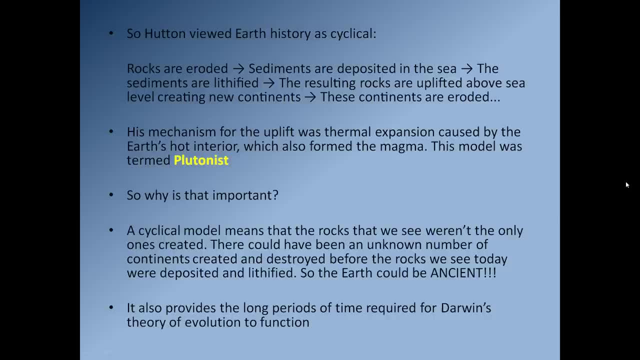 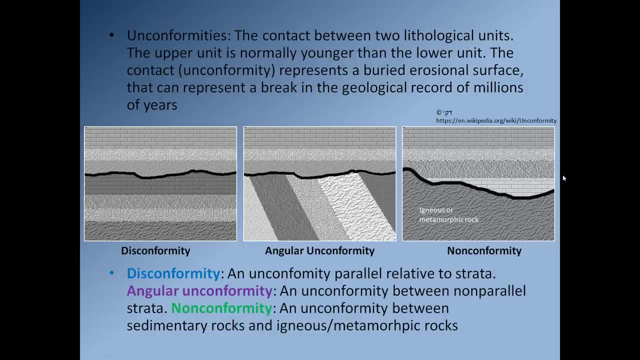 for evolution to be permissible. So the model that Hutton came up with here was very, very useful when Charles Darwin and Wallace came up with the theory of evolution. Okay, so that's been 20 minutes, so this would be a good time to take a minute. 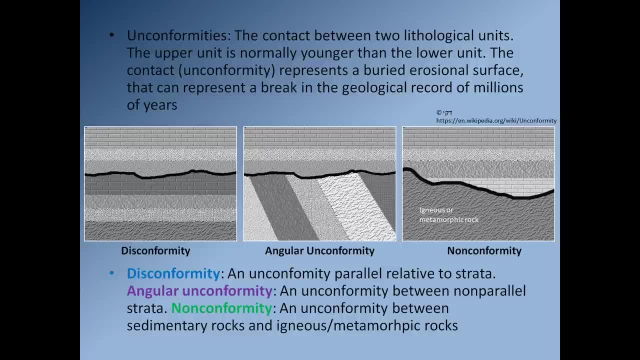 So pause the presentation, get up, have a walk around, get a glass of water And then come back once you've had a few minutes to relax. Okay, so when we look at a sequence of sedimentary rocks or sequence of rocks in general, 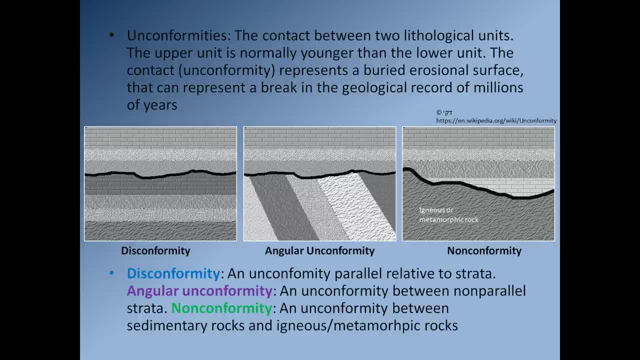 it begins to become clear that some portions of the sequence are missing. So there is nowhere to be found. There is nowhere on the surface of the earth where you have a complete sequence of rocks. Okay, wherever you go on the earth, you may have a- you know, a pretty complete sequence of rocks. 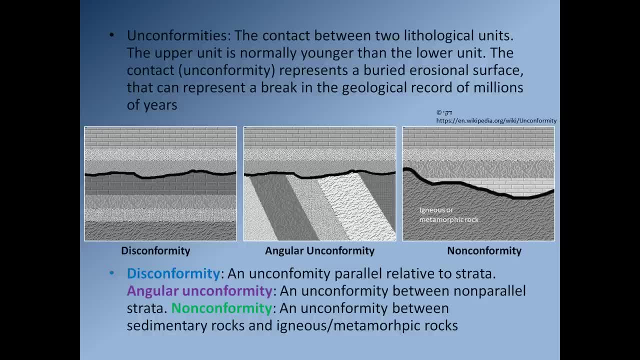 but there will always be portions of the rock sequence that aren't there because they've been eroded. So this process of losing rock. now, as I said, geologic time is based on rocks and fossils, so if you lose rock from the record, that essentially means you've lost time. 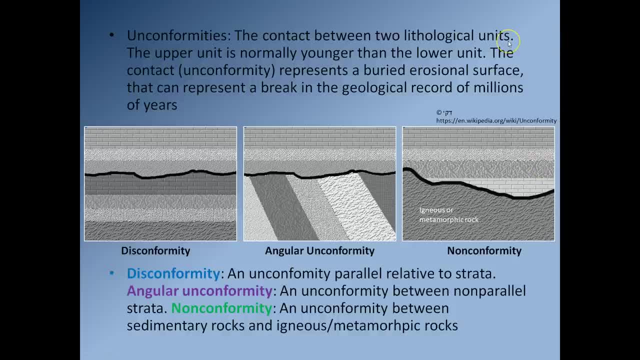 So unconformities are the contact between two lithological units. The upper unit is normally younger than the lower unit and the contact- that's the unconformity- represents a buried erosional surface. Essentially, that can represent a break in the geologic record of millions of years. 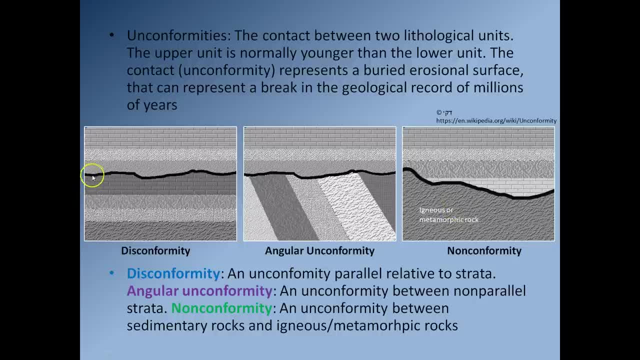 So in these three diagrams here you can see the unconformity is marked out by this emboldened line here, And so in most unconformities the older rocks will be below the unconformity and the younger rocks will be above the unconformity in most cases. 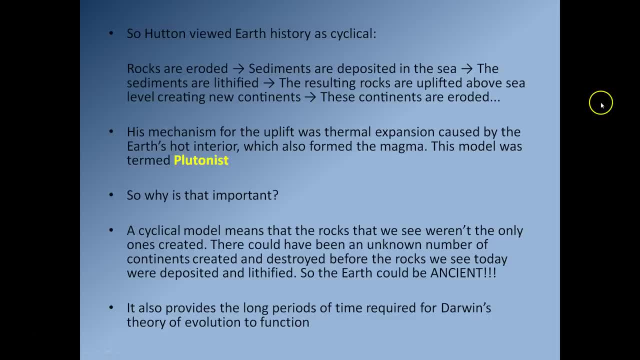 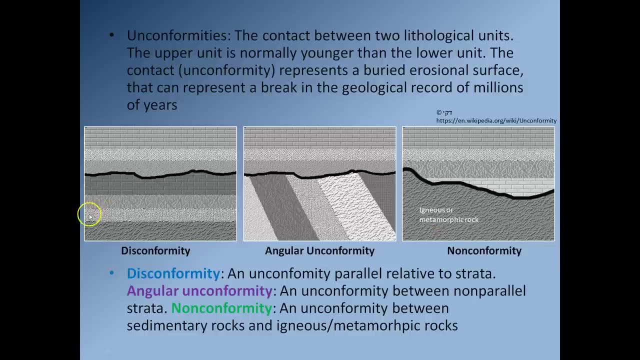 So when it comes to unconformities, there are three main types. The first one is a disconformity. So in a disconformity the rocks below the unconformity are horizontally bedded to the horizontal. Above the unconformity the rocks are also horizontal. 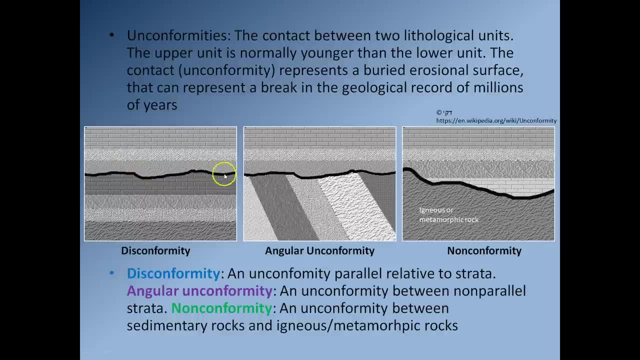 The unconformity itself, however, undulates, it has topography. Okay, in the case of an angular unconformity, the rocks below the unconformity are topographic, They're tilted, so they're not horizontal. they're not horizontal, they are at some kind of angle. 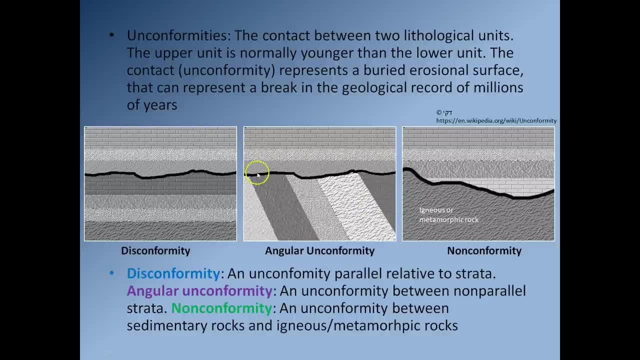 Above the unconformity, the rocks are horizontally bedded and, once again, the contact between the two, the unconformity is this undulating surface. Now, in both of these two cases here- disconformities and angular unconformities- what we're looking at is we're looking at a situation like we have now. 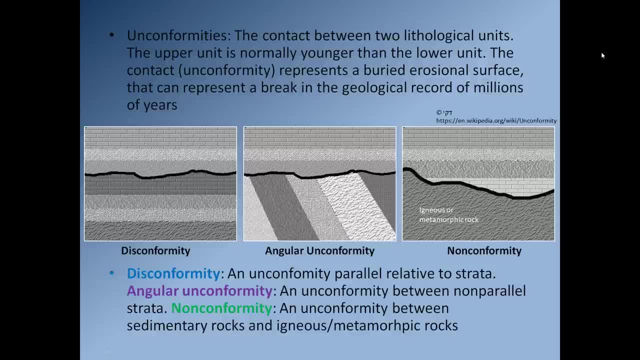 So at the moment, the United States is pretty much as exposed as it can possibly be. Okay, so the vast majority of the continental crust that makes up the United States is currently above sea level, And so that means at this moment in time, the United States is one massive factory for making sediments through erosion. 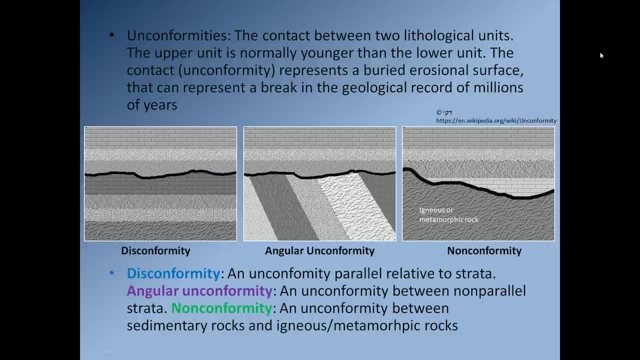 And as all the rocks on the surface are eroded, we are losing time from geologic point of view. So, if you imagine, this is the modern surface of the United States, going all the way from the west coast, all the way from Seattle over here, all the way over to Boston, over here. 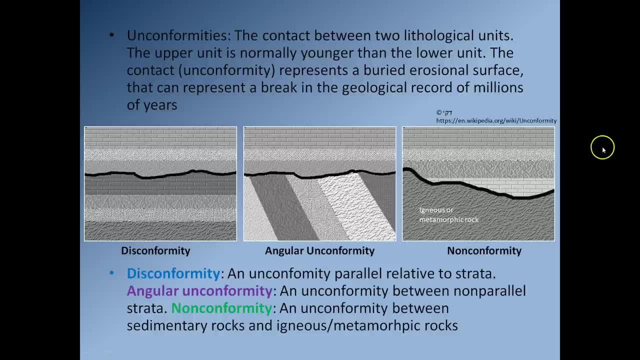 And so we have this giant unconformity Going from one side of the United States to the other, where erosion is actively going on and so we're losing rock, And so at some point, let's say, the United States goes back below sea level and we have sediments deposited over the top. 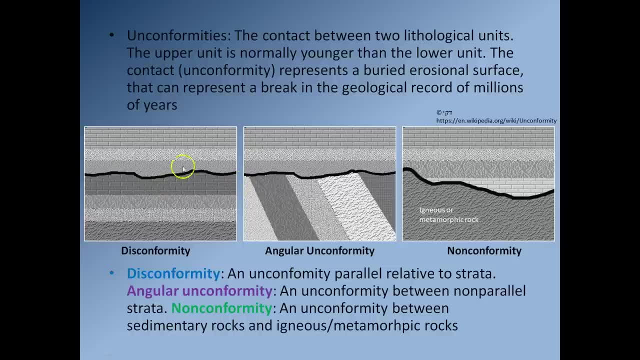 Well, clearly, between this layer of rock here and this layer of rock here, we're going to have a period of lost time, aren't we? And so that goes for disconformities and angular unconformities. Now, non-conformities are slightly different. 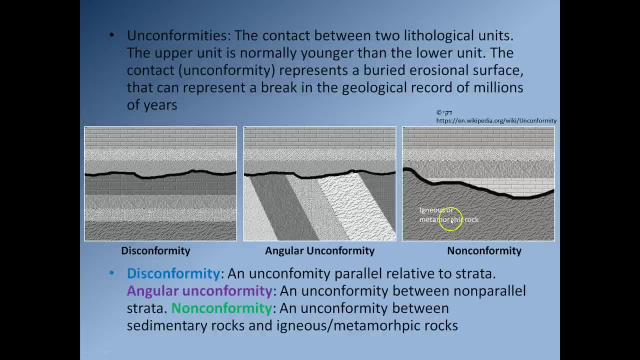 A non-conformity is when we have a the contact between a body of igneous or metamorphic rock and sedimentary rocks. So essentially, the contact between the igneous or metamorphic rock and the sedimentary rocks, that interface between the two, is considered to be the non-conformity. 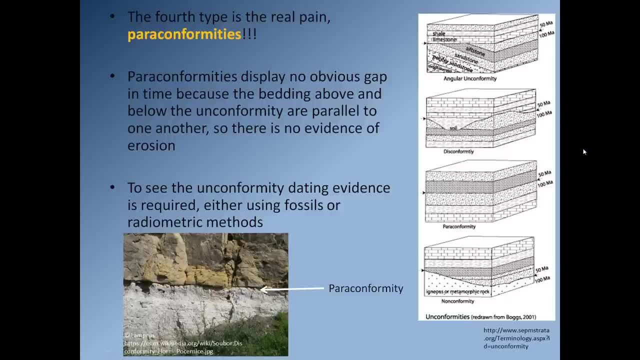 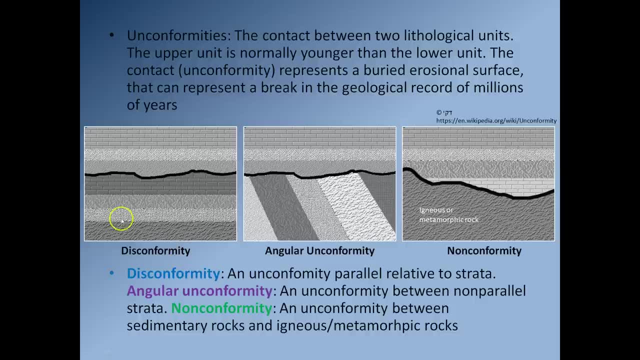 Now there is a fourth type of unconformity which is referred to as a paraconformity. Now paraconformities are rather difficult to see. So in a paraconformity there are two types of non-conformities. In paraconformity, the rocks below the unconformity are horizontally bedded. 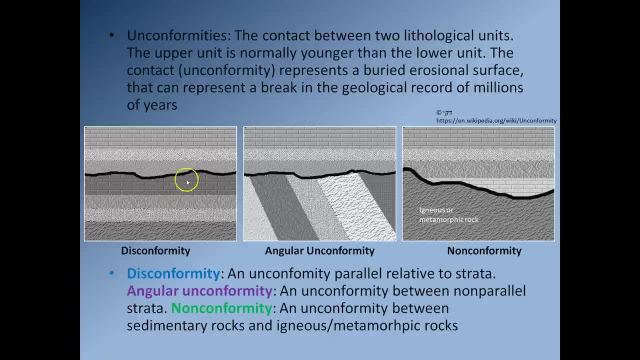 Above the unconformity, the rocks are horizontally bedded. Now you can see it here I'm pointing to a disconformity. Now, in a disconformity, the unconformity itself is undulating. it has topography. 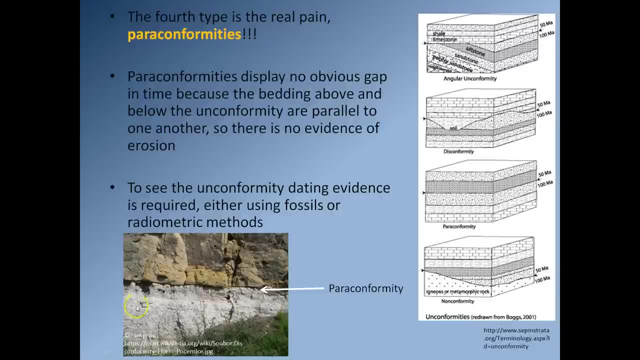 In the case of paraconformity, the rocks below are horizontally bedded, The rocks above are horizontally bedded. The unconformity itself is also horizontal. it's completely flat, And so that means that paraconformities are extremely difficult to see, because it looks like that's. you know that looks just like a bedding plane between two layers of rock. 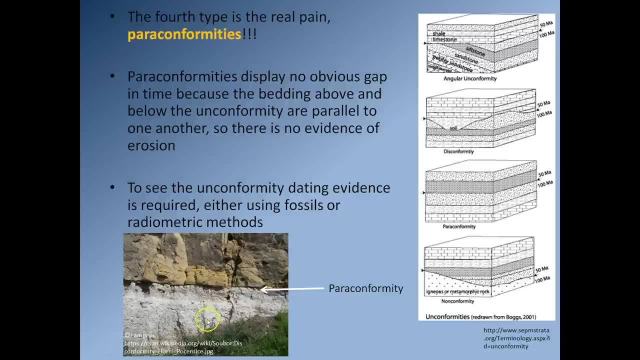 So the only way you can tell, you know, you can tell there's a paraconformity there is if you can date this layer of rock here, this layer of rock here, And then when you date them, you'll suddenly realize that maybe, let's say, you've got two million years missing, at which point you realize that this contact here must be an unconformity. 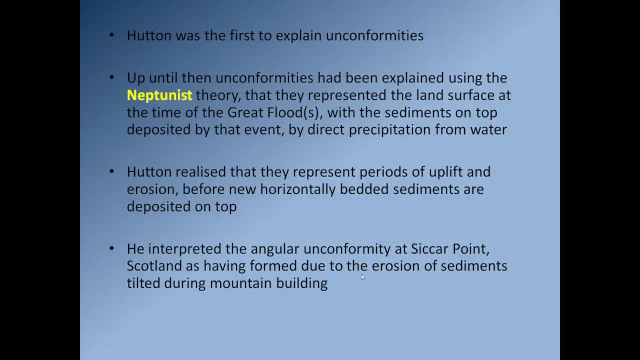 Unconformities. So Hutton realized that these unconformities actually represented periods of uplift and erosion before new horizontally bedded sediments were deposited on top. So he interpreted the angular unconformity at Sick Air Point in Scotland as having formed due to the erosion of sediments tilted during mountain building. 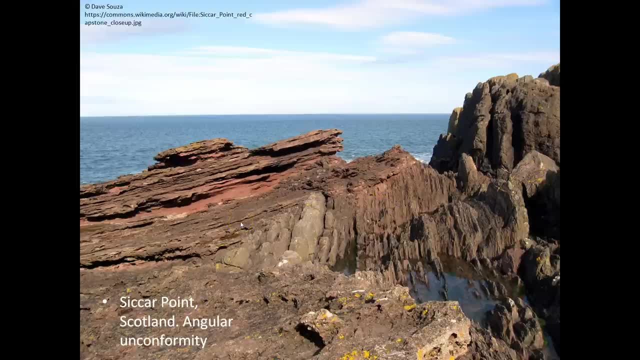 So here is Sick Air Point. It's in northeastern Scotland. If you ever get the opportunity to go there, dress warm, because it's a very exposed area and the wind comes whipping off the sea with quite a bit of force. But nevertheless, here we go. 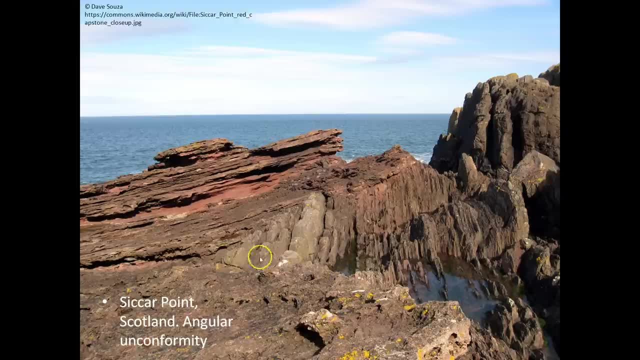 So if we look at the Sick Air Point unconformity- I didn't draw a line there, but the Sick Air Point unconformity is coming up through here. OK, so that's the approximate path of it, And so what you'll notice is below the unconformity, we have these rocks here and you can see that these rocks are vertically bedded. 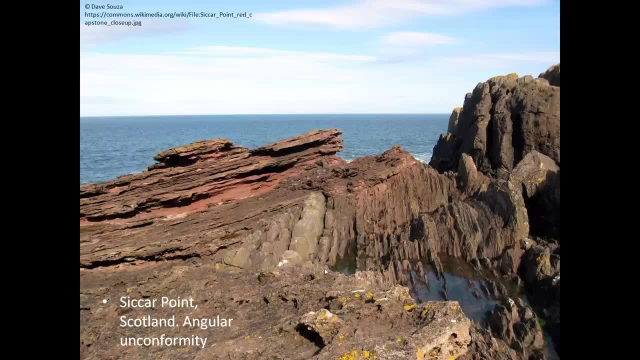 So the layers, the layering in the rock is pointing all the way up, Almost straight up Now, above the unconformity. remember, the unconformity is coming along here. The rocks above the unconformity are horizontally bedded. 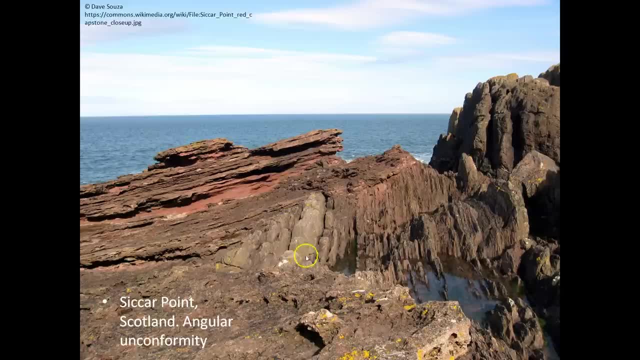 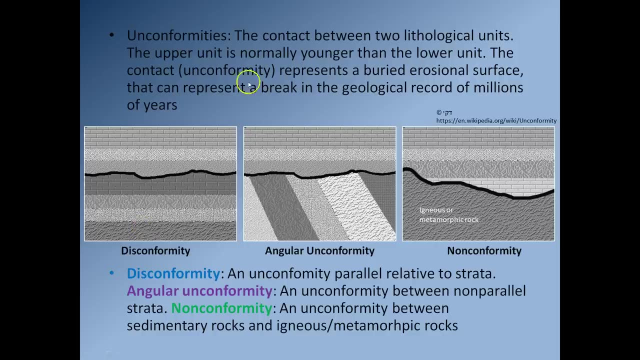 So you can see these layers of these. you know, the portion of rocks below the unconformity and the portion of rocks above the unconformity are angled significantly differently. So what we have here is a angular unconformity. So what does this actually mean? 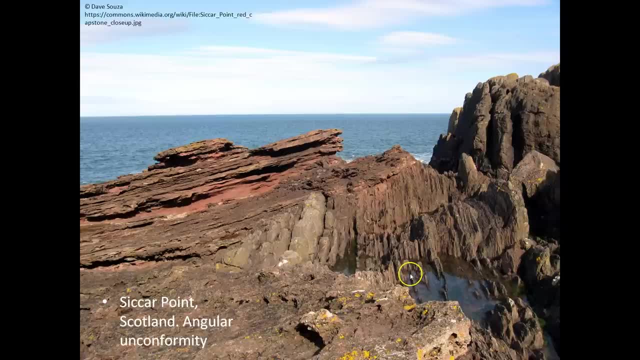 Well, what Hutton realized was that these layers of sediments here- Well they were, They were- They would have initially been deposited as nice horizontal sheets, And so that means that obviously these rocks have to have been tilted after they were lithothied. 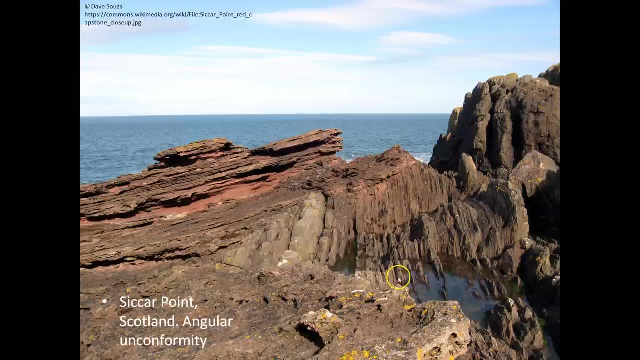 And so he realized that the process of actually tilting these rocks was likely to have occurred when the rocks were being pushed up above sea level so that they could be eroded. Now, once he realized the rocks had been pushed above sea level, he realized that this surface here has to have represented the surface of the Earth at some point in the past. 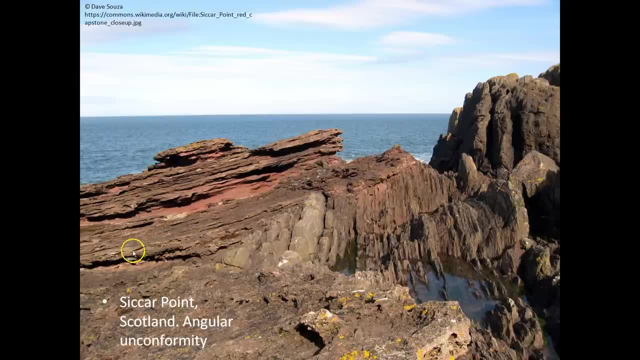 And any rock, The rock that was above this unconformity, has been eroded away and lost. Then he realized that clearly this area, with these vertical sequence, vertical sequence rocks, must have probably dropped down below sea level and it's had sediment deposited over the top in the form of nice horizontal layers. 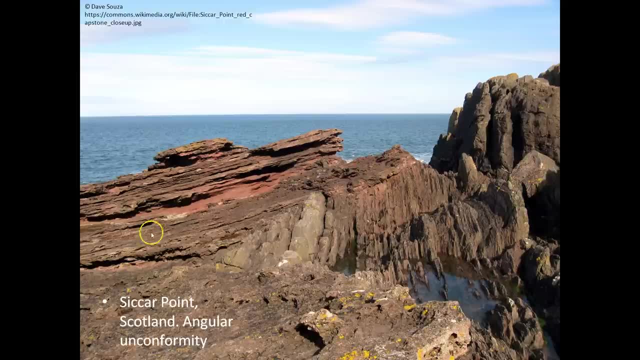 So by looking just at this one point- he's not location, Sorry, he's not only you know- begun to define what unconformity actually is, he's also been able to show that rocks have to be uplifted and tilted in order to get them. 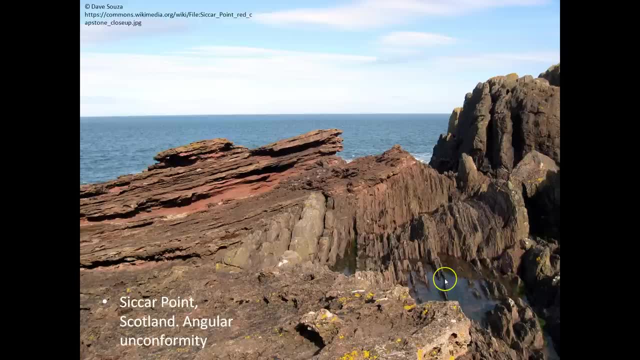 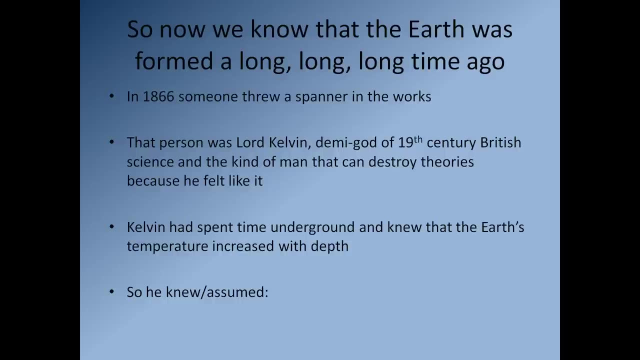 So above sea level, so they can be eroded. So it's a very important location for geology. So now we have some idea. The Earth was formed a long, long time ago. So in 1866, someone threw a spanner in the works and that person was a gentleman called Lord Kelvin, who you'll know from the Kelvin temperature scale. 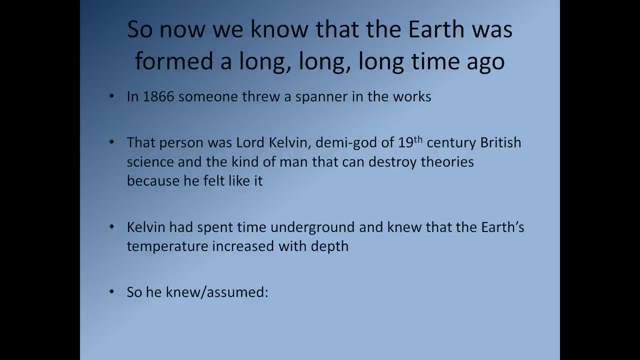 And he was a demigod of 19th century British science And he was the kind of man that could destroy a theory because he felt like it. So you know, Lord Kelvin, And said no, I don't agree with your idea. Pretty much everyone in the scientific community at that time would go. yes, I agree with Lord Kelvin, You're clearly wrong. So Kelvin had spent some time underground and he knew the Earth's temperature increased with depth. So this is what he knew and what he assumed. 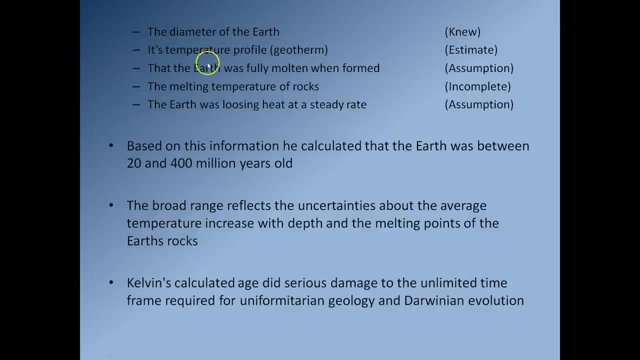 So the first thing is he knew the diameter of the Earth and knew how big the Earth was. He also knew to some degree the Earth's temperature profile, So we knew the Earth was getting hotter as you went down into it. Now Most of his temperature profile was an estimate with a bit close to the surface. he got from actual measurements. 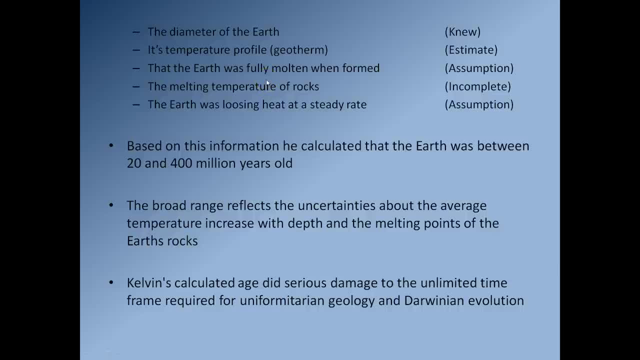 So he also assumed the Earth was fully molten when it formed, which was a assumption, But once again it was correct. He knew the melting temperatures for certain rocks And he knew that the Earth was losing heat at a steady rate. Apparently, it was losing heat at a steady rate. 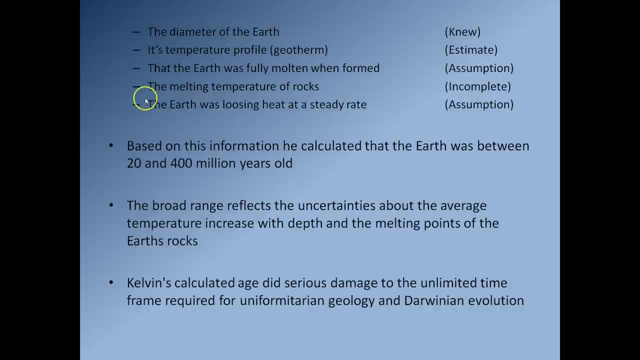 So what was going on? So essentially what he said was the Earth started at as a molten ball and because he knew how hot that molten the molten ball had to be to have liquid rock from these melting points, here he had a starting temperature. 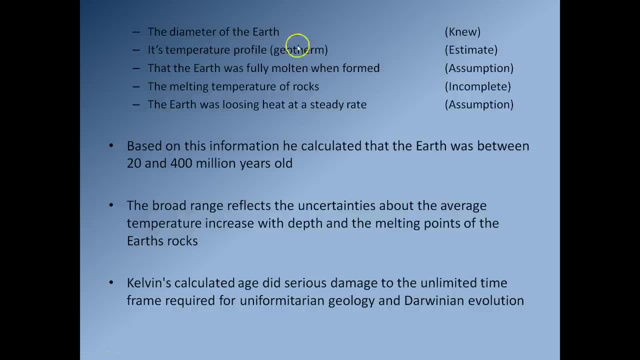 Well, he knew the current temperature of the Earth. He can also look at the Earth's profile, and so he could calculate how long it would take the Earth to go from essentially a sphere of molten rock the size of the Earth- So it shows a sphere of molten magma the size of the Earth- to the present day solid- well, mostly solid- planet that we have now. 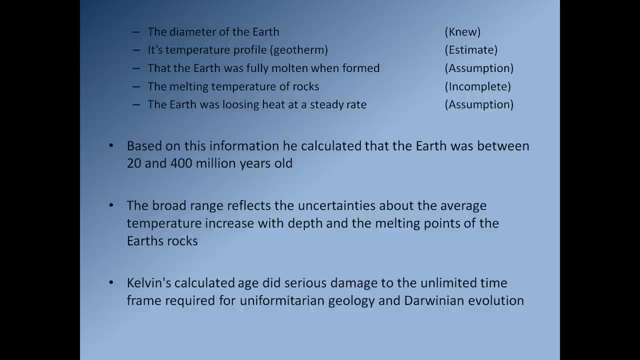 And so when he did that calculation, he calculated the Earth was between 20 and 400 million years old, So you know still pretty old. but Well, that's, you know, not really that old in the grand scale of things. 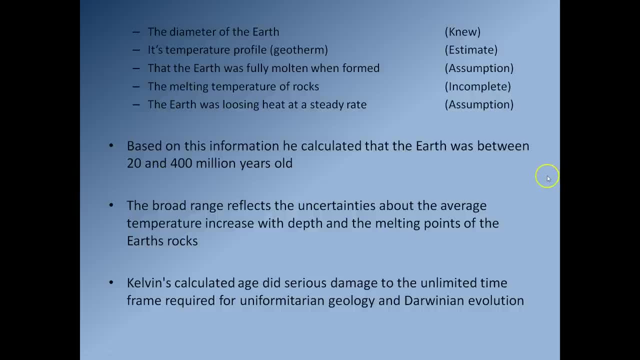 So this broad range here represents the uncertainties about the average temperature, increase in depth and the melting points of certain rock. So he had to make several assumptions. and because he had to make several assumptions it means he had quite a broad spread when it came to calculation. 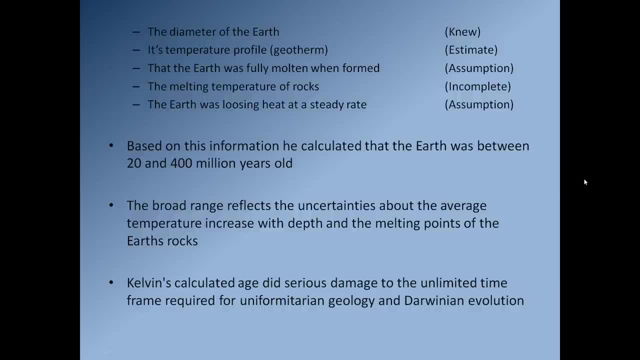 calculating the answers. So Kelvin's calculated age did serious damage to the unlimited time frame required for uniformitarian geology and Darwinian evolution. so essentially he was saying no, the earth is only you know, and he tended to try and stick to the lower end of the scale. this 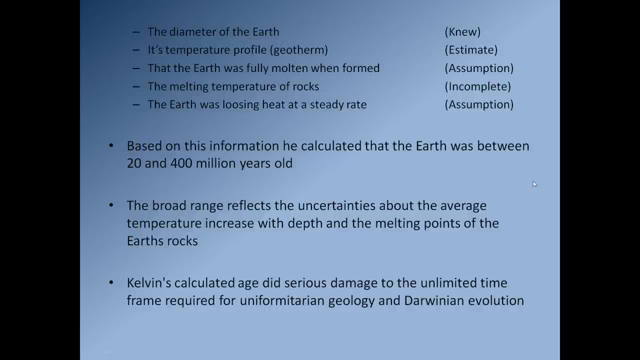 20 million year age here. so he was saying, well, no, the earth isn't actually that old. you know Hutton's ideas of continents rising, being eroded, sediments being deposited, producing new continents, you know, and there being several cycles of this process, not enough time for that to happen. so 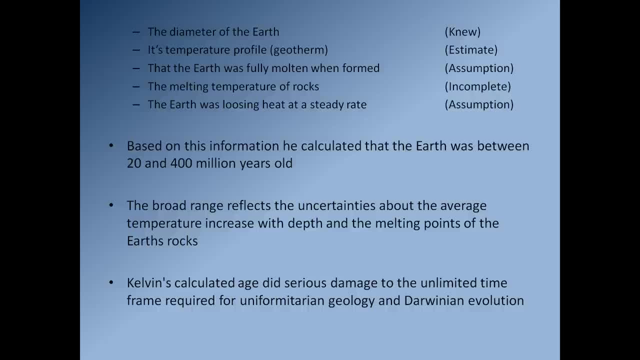 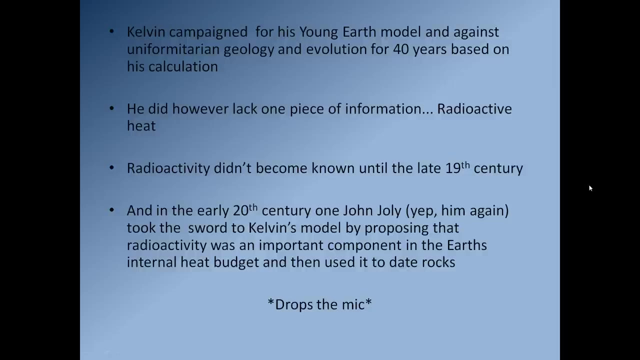 Hutton's wrong. and if Hutton's wrong, well that means that Darwinian evolution is also not going to function correctly. so all of a sudden you know we have a real problem. So Kelvin campaigned for what he referred to as his young earth model and against uniformitarian geology and evolution. for 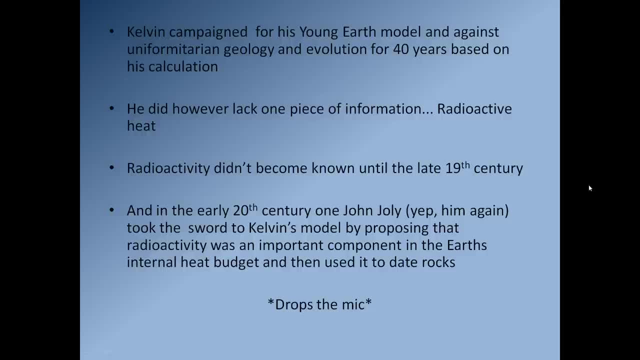 40 years, based on these calculations that he did. So he did, however, lack one piece of information, and that's radioactive heat. so he didn't realize that inside the earth there are all these radioactive isotopes. that's helping to keep the interior of the earth warm Now: radioactivity. 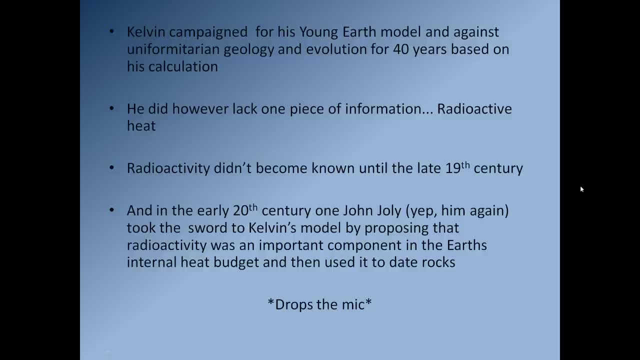 didn't really become known and fully understood until the late 19th century and in the early 20th century. one- John Jolly- here he is again- took the sword to Lord Kelvin's model by proposing that the radioactivity from the radioactive isotopes inside the earth 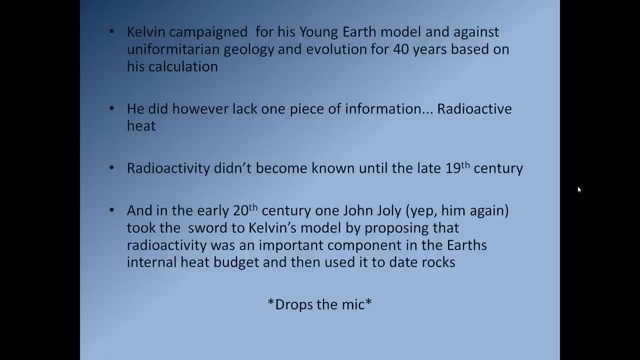 was actually keeping the earth's internal heat budget up, and so they helped to keep the interior of the earth warm, and so this meant the earth could be a lot older than Lord Kelvin had calculated, And so essentially, that's it. once John Jolly puts that forward, radioactivity saves a day. 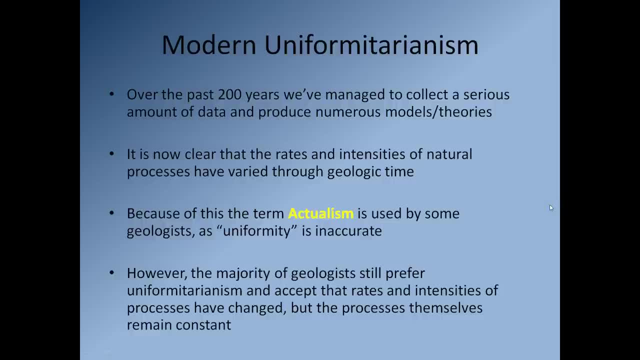 John Jolly walks off stage, drops the mic. So modern uniformitarianism. So, over the past 200 years, we've managed to collect a series of data that shows that the Earth's internal heat budget is a serious amount of data, and produced numerous models and theories when it comes to geologic 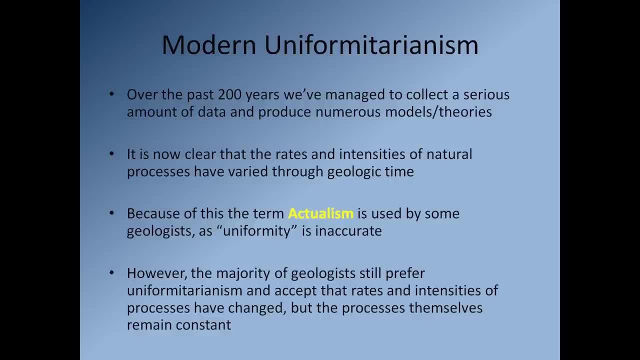 processes. So it's now clear that the rates and intensities of natural processes have varied through geologic time. So the initial idea of uniformitarianism was that things were happening at a constant rate and they've happened through that constant rate throughout geologic time. 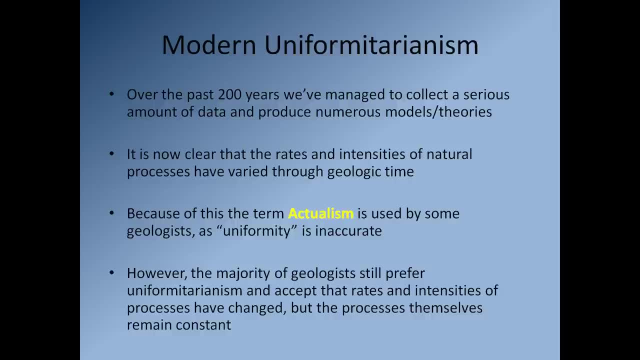 What we've realized now is that the rates will have actually changed in some cases. So we know, for instance, you know, spreading ridges in the middle of the ocean. well, that's where new oceanic crust is made. Now, at the moment, we know that. 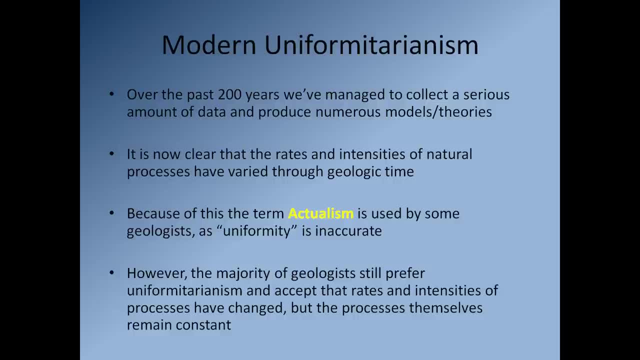 spreading ridges will operate. you know they'll will create new oceanic crust somewhere in the region of about three to nine centimeters per year, depending on which which spreading ridge you're at. In the past, however, so during the Cretaceous, we know that spreading ridges were 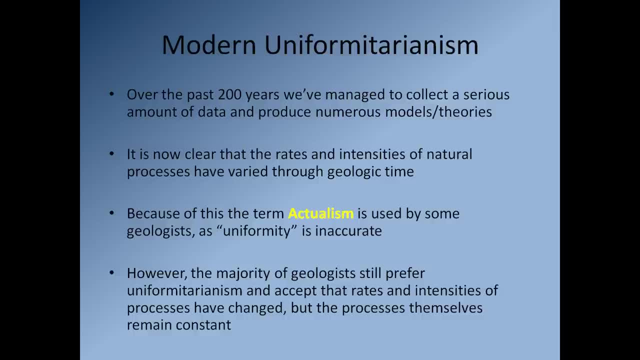 churning out oceanic crust at absolutely astronomical rates. So, although the process is the same, we actually know from the geologic record that the rates of geologic crust are different, and so this has led to the term actualism, and that's used because some geologists 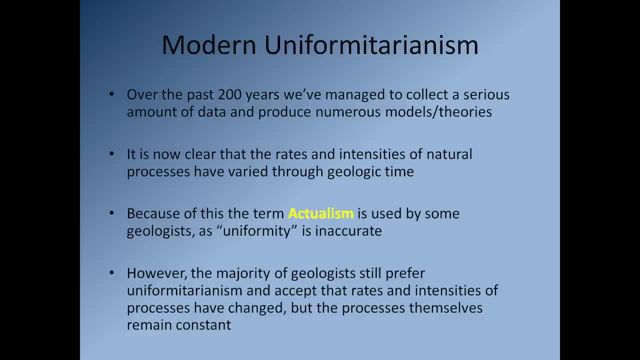 you know, view uniformity as an inaccurate term. So things weren't always happening at the same rate. the rates at which the processes occur were able to change. So, however, the majority of geologists still prefer to use the term uniformitarianism, and we use it with the understanding that the 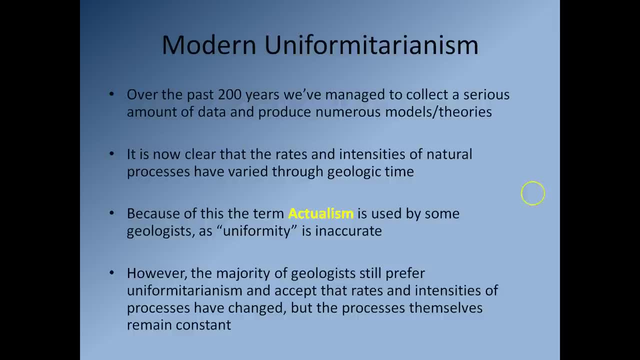 rates and intensities of certain processes will have changed through geologic time, but the processes themselves remain constant. So even though the rate of new oceanic crust being made at spreading ridges will change, the actual process of forming that oceanic crust remains the same. 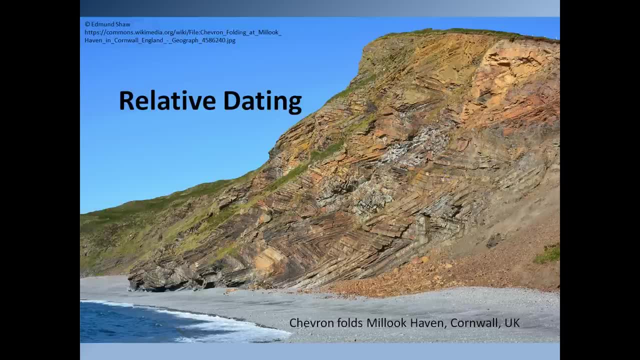 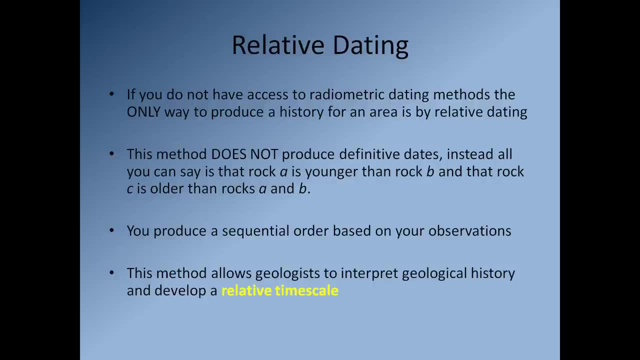 Okay, so this brings us on to relative dating. So if you, if you're interested in understanding the rate of new oceanic crust being made at spreading ridges, you do not have access to radiometric dating methods, so you can't, you know, get a numerical. 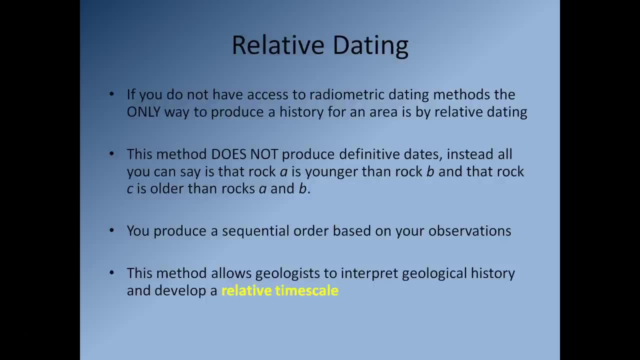 value for your, for your rock. the only way to produce a history for an area is by relative dating, so the method does not produce definitive dates. instead, all you can say is that rock a is younger than rock b and that rock c is older than rocks a and b, so you're essentially producing a. 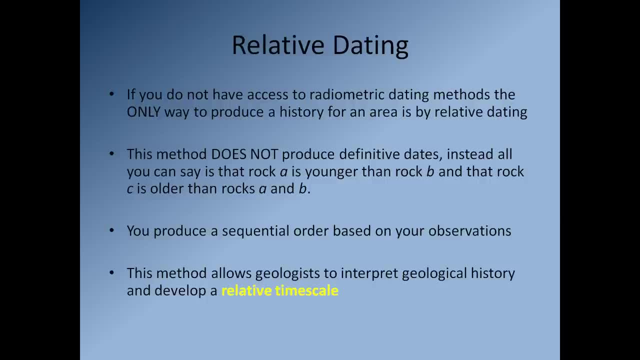 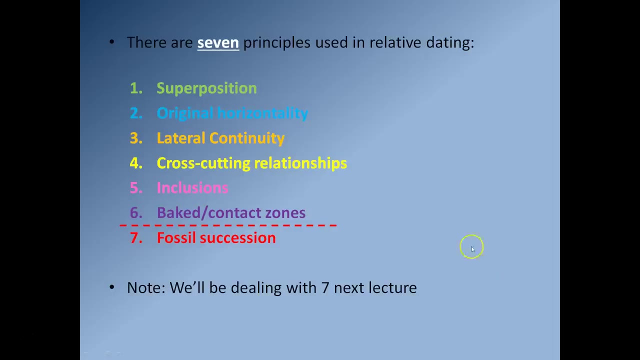 sequence, you know, of rocks, which you put in order based on their age, and this method allowed geologists to interpret geological history and develop what's referred to as the relative time scale. so there are seven principles used in relative dating: superposition, original horizontality, lateral continuity, cross-cutting relationships, inclusions, baked contacts and zones and fossil. 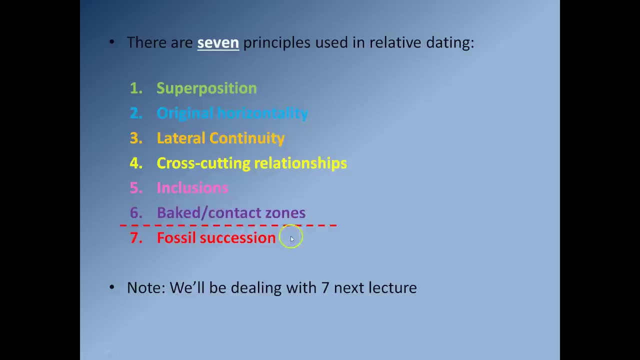 succession, also superposition, sometimes referred to as faunal succession. now, point number seven isn't going to be dealt with until next week, so we're not going to worry about that. so today you're going to be looking at superposition. original horizontality, lateral continuity, cross-cutting relationships, inclusions. 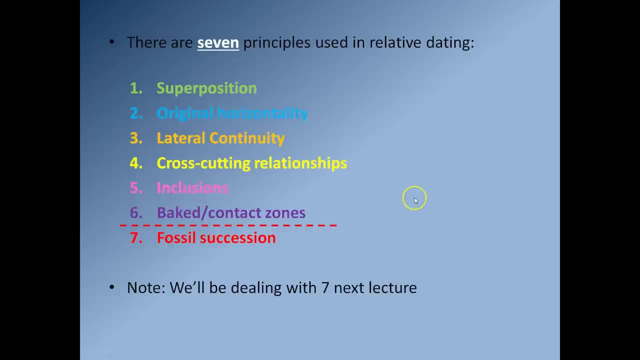 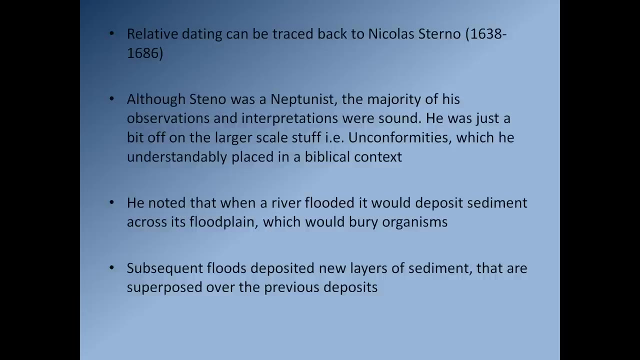 and baked contacts and zones- sorry, baked zones, baked contacts. so relative dating can be traced back to nicholas sterno. so sterno was a neptunist, so the majority of his observations were essentially based on the idea of a great flood. however, the observations he actually came up with and the vast majority of his interpretations, 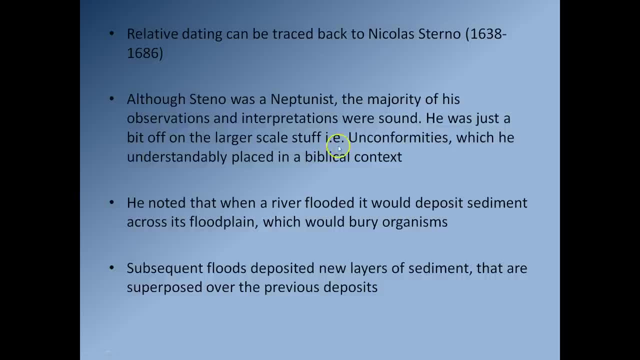 were actually sound. so he was just a bit off on the larger scale stuff. so he noted that when a river floods, it would deposit sediment across a floodplain in horizontal layers, and those horizontal layers would bury organisms. so he realized that as a result of that he was able to. 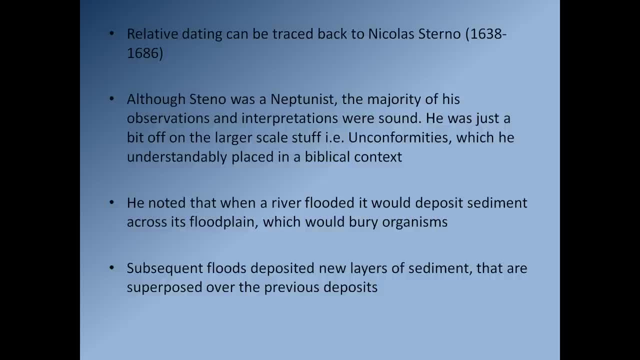 essentially that could be where fossils came from. he also realized that because you're producing these nice horizontal layers, he suddenly came to the realization that sediments were deposited as horizontal sheets. he then realized that subsequent floods would deposit new layers of sediment over the top of older layers of sediment, so they would essentially superimpose. 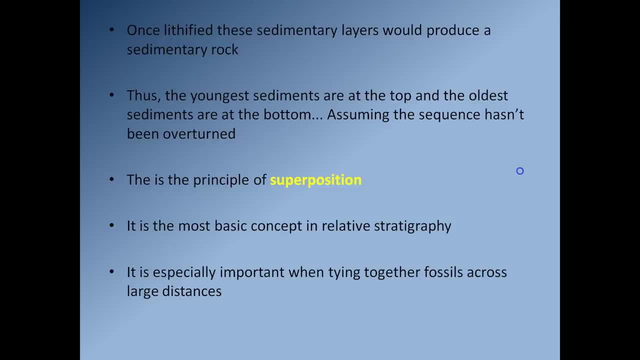 themselves over the top of the older layers of sediment. so he then realized that if you went to lift, if you then lithified this, this stack of sediments, they, essentially you would retain the sedimentary layers in the rocks that formed. so he then, he therefore realized that 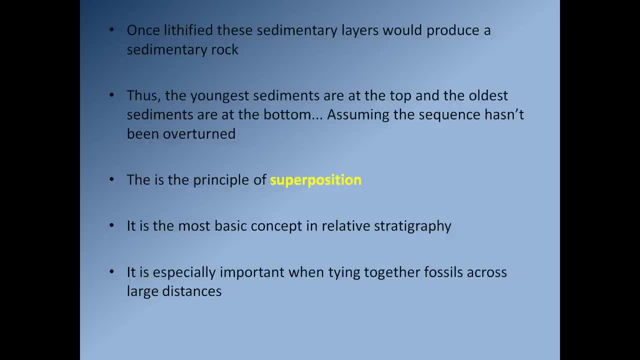 when, when you see a sequence of sedimentary rocks, in 90 percent of cases the sedimentary rock at the base of the sequence will be the oldest and the sedimentary rock at the top of the sequence will be the youngest. so essentially that is the principle of superposition. if you see a sequence, 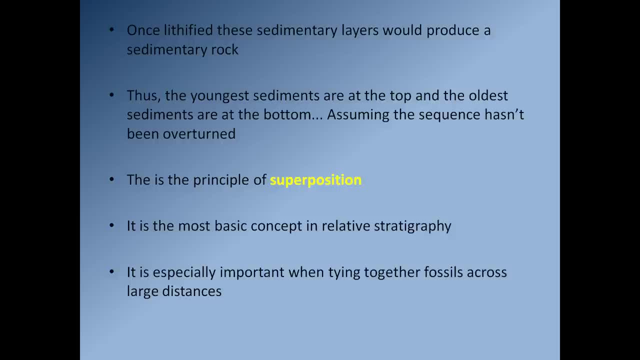 of sedimentary rocks. chances are the rock at the bottom of the sequence is the oldest, the rock at the top of the sequence is the youngest and it's the most basic concept of relative stratigraphy. so it's especially important when you, when you are tying fossils together across large 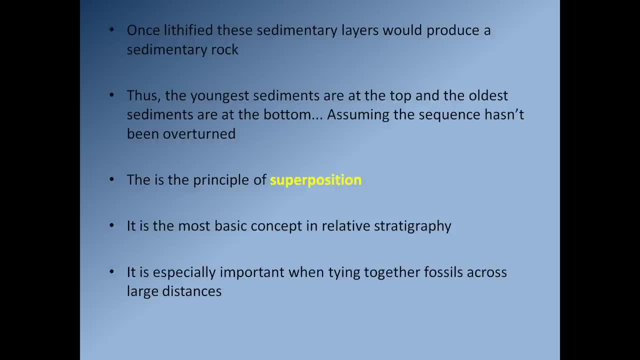 distances, because that means if you have a rock at the bottom, so let's say rock a and that has a fossil in it. well, you know, rock a is probably the oldest, because at the bottom of the sequence, that means any fossils in rock a must also be the oldest. and at the 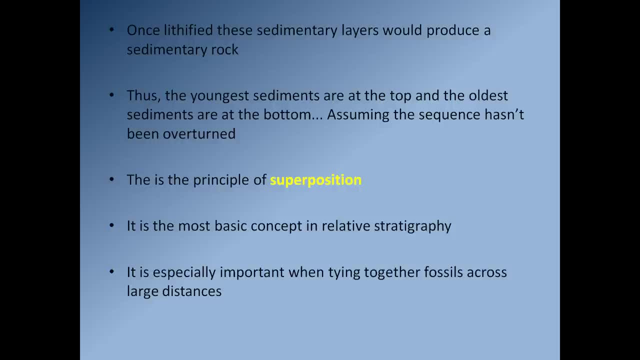 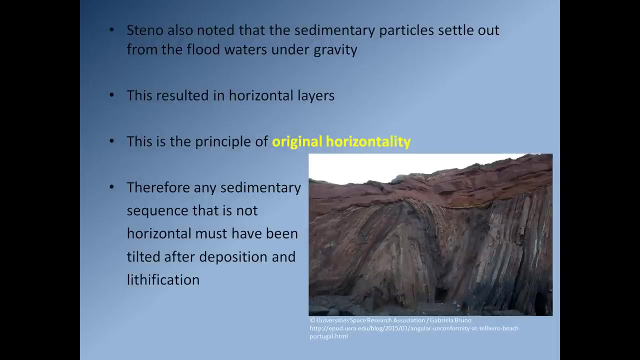 top of the sequence you have rock z. well, rock z is the top of the sequence, therefore superposition says it must be the youngest. therefore, any fossils in layer z must therefore also be the youngest fossils. so sterno also noted that sedimentary particles settle out from flood waters under gravity. 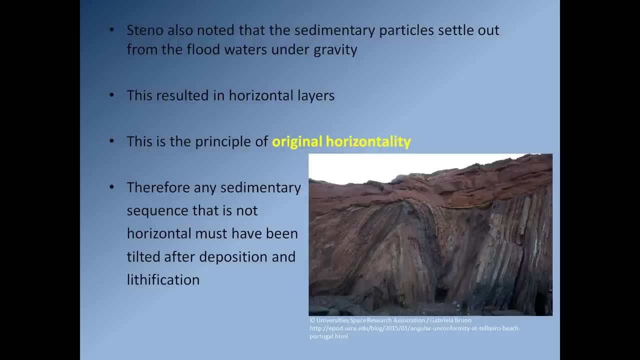 and he realized that sediments were deposited as horizontal layers. so this is the next observation he made: this is the principle of original horizontality. sedimentary rocks were well the, so to say, the sediments that make sedimentary rocks were initially deposited as horizontal layers. it therefore means that if you see a sequence of rocks, 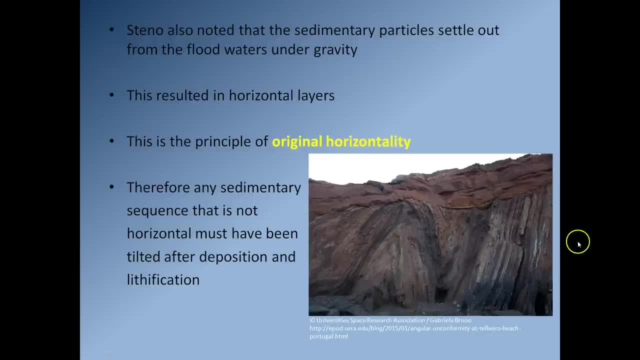 like this one down here, which are not nice horizontal sheets, then it means they must have been tilted after the sediment has been turned into a rock. so initially these layers of sediment here were nice horizontal layers like these layers above at the top. but once the horizontal layers have been turned into rock, that sequence of rocks was then was then folded and 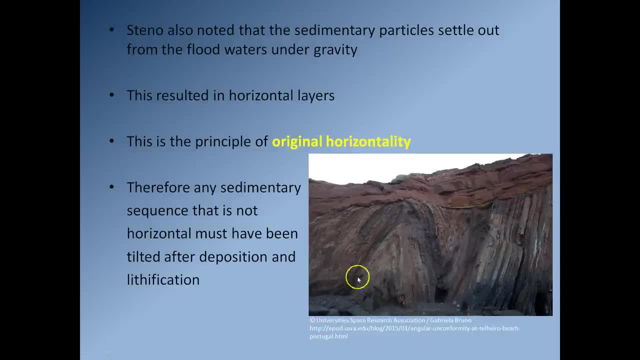 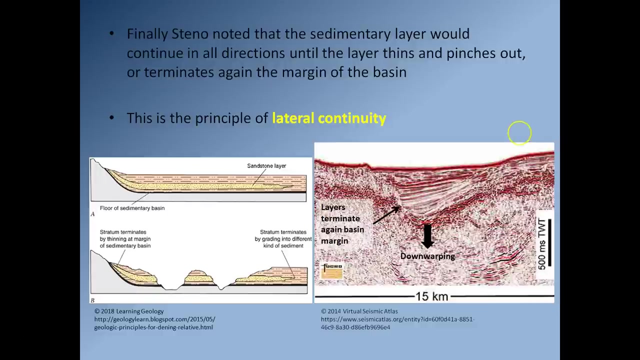 deformed, as you can see there. so that means any tilting must have occurred after lithification, after the rock, after the sediment was turned into a rock. the final thing that sterno noted was that sedimentary layers would continue in all directions until the layer thins and pinches out or terminates. 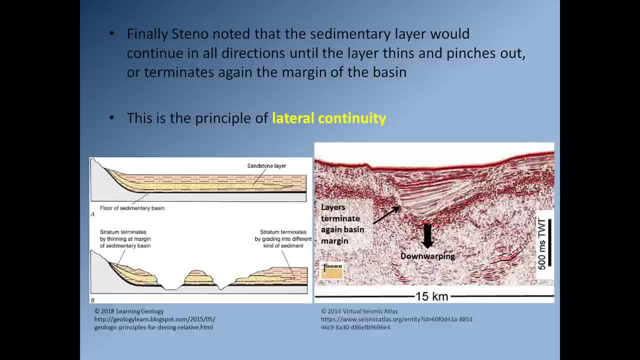 against the margin of a basin. so, once again, if you imagine a river flooding, well, the flood water leaves the river and obviously the water continues for a long distance as it, you know, as it moves across the surface of the earth, it will deposit sediment as it goes. 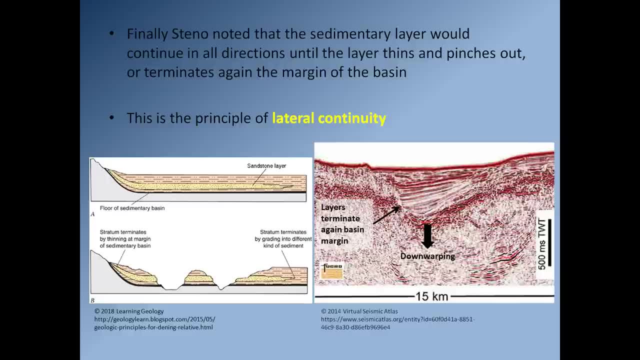 now, eventually, the, the, the river, water is going to run out, of sediment to deposit. so what you'll notice as you move, as you follow a layer of sediment deposited by something like a flood, the layer will steadily get thinner and thinner and thinner and then eventually it will just disappear. and in geology, this process of a layer getting thinner and thinner. 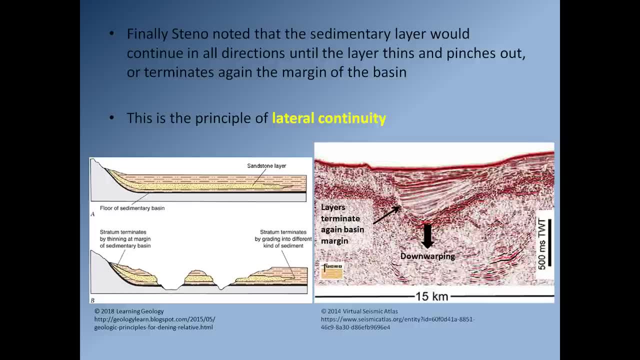 and thinner and then eventually disappearing, is referred to as pinching out. so if we look at this diagram here, we can see here's a layer of sedimentary rock and we can see it's continuing laterally until eventually the layer gets thinner, thinner, thinner and then it eventually pinches out. 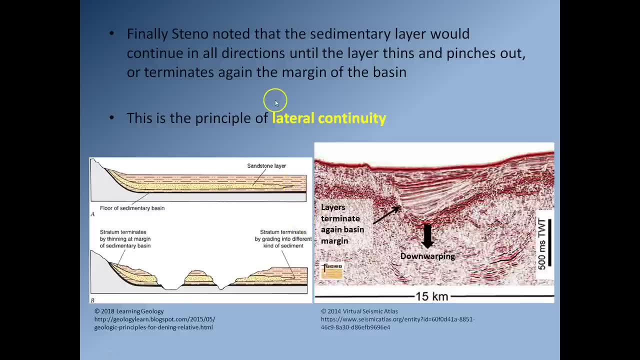 and disappears. the other thing a layer of sediment can do is that it could continue horizontally until it terminates against the edge of a basin, some kind of vertical surface like, let's say, you know, a levee along the levee along the bank of a river, or maybe a um, oh, i can't. 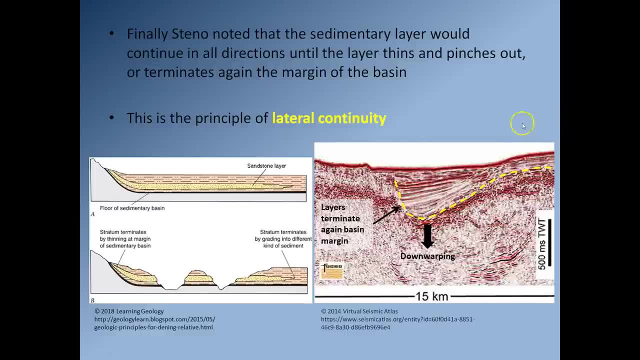 write term there, or maybe let's say some kind of hill, something like that. so in this case, we can see, here's our basin. so this is a depression that's filled with water and, you know, filled with sediment, and you can see the layers of sedimentary rock within it here and you can see. 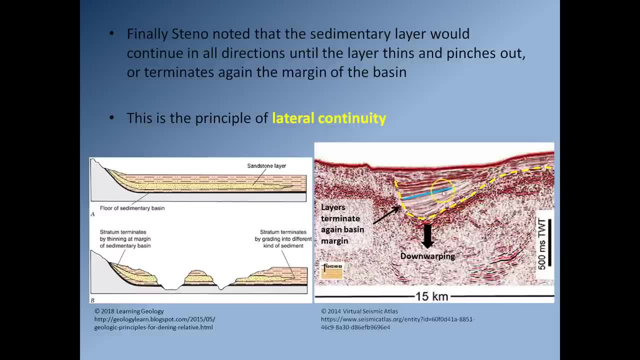 the layers of sedimentary rock. they're marked out as blue line, while they continue all the way across the basin until they hit the basin edge, at which point they obviously can't go any further. so what sterno said was that sedimentary rocks would, uh, continue, so sorry, should i say a layer of 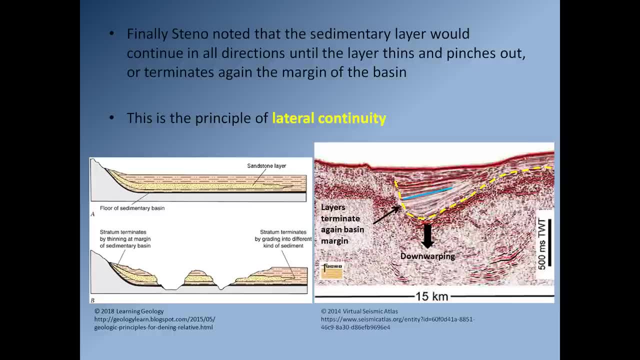 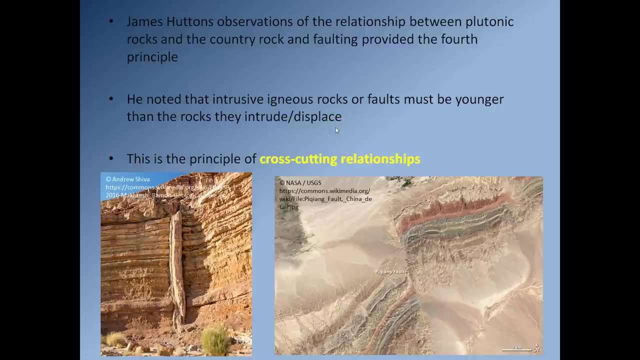 sediment will be deposited in all directions until the layer thins and pinches out or terminates against a basin margin, and that's referred to as the principle of lateral continuity. okay, so that's been 40 minutes, so once again, time to pause the video. get up, have a walk around, get. 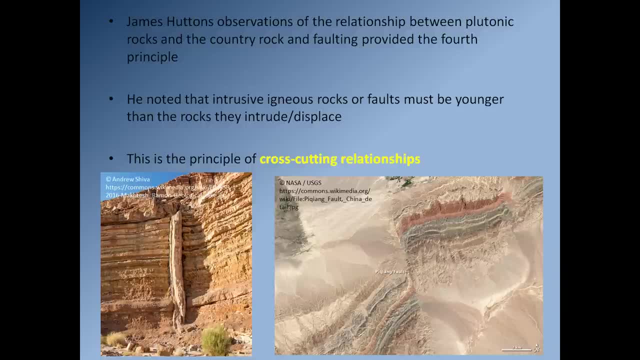 a glass of water, take a couple of minutes to get your head straight and then come back and we'll be right back, okay? so what's the next principle of relative dating? well, that was produced by james hutton, and james hutton, and using his observations, realized that the relationship 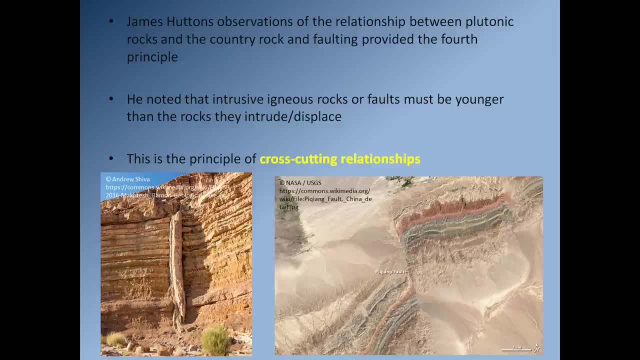 between plutonic rocks, that's igneous rocks, and the country rocks, and faults and faulting in the country rocks provided the fourth principle. so he noted that intrusive igneous rocks or faults are younger than the rocks they intrude or displace. so here we have two pictures. so on this side we 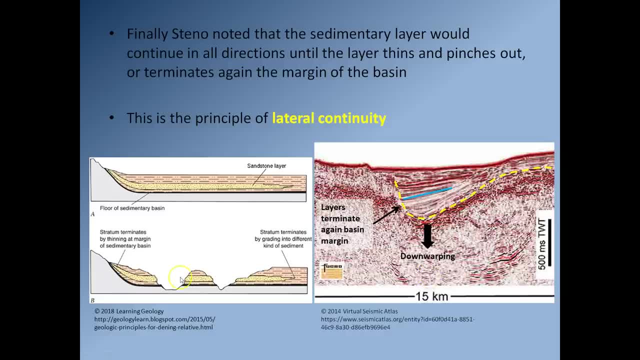 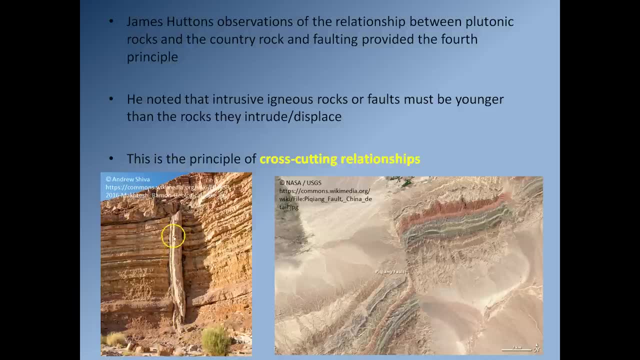 have a sedimentary dike on this side. we have a fault. so what we're seeing over here is: here's a nice sequence of horizontally bedded rocks and here's this sedimentary dike smashing through it vertically. now obviously for this sedimentary dike to cut this sequence of rocks. 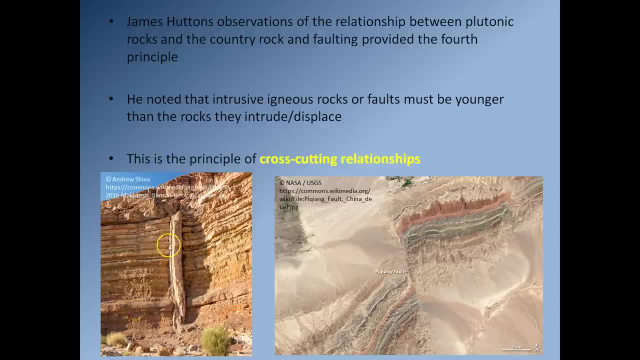 well, clearly, the sequence of rocks has to have been there first, doesn't it? so it means that this dike here must therefore be younger than the sequence of rocks. that the dike is cross-cutting makes sense. same thing goes for this sequence of rocks here. okay, so here we have a sequence of rocks. these ones are very nice and easily. 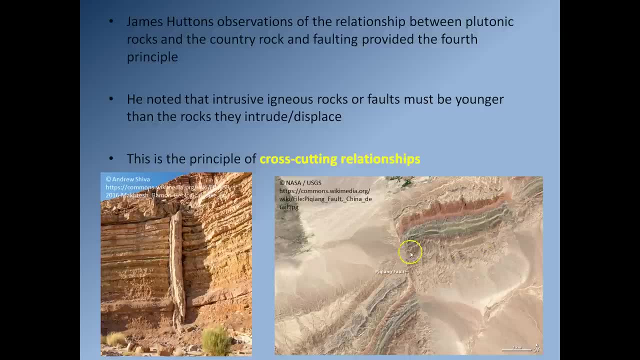 picked out because they have these distinct colors to them, and so the only way you can cut the rocks with a fault is, once again, if the rocks were there first. so that means that if you're trying to fault something you know, essentially crack it and put a, put a large. 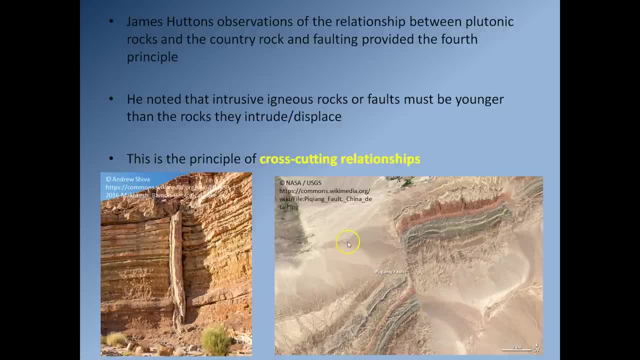 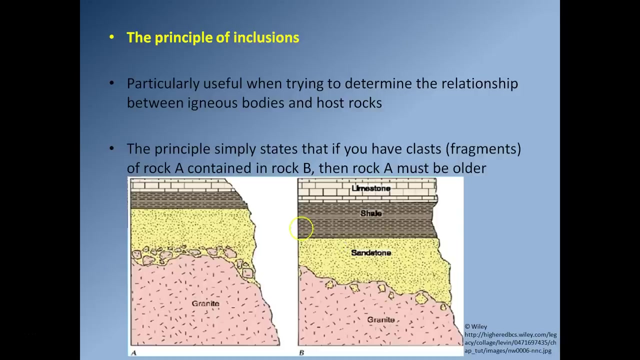 break in it. essentially, the rocks have to have been there to begin earlier or before the fault. So that's the principle of cross-cutting relationships: Dykes and faults must be younger than the rocks which they cross-cut. So then we have the principle of inclusions. 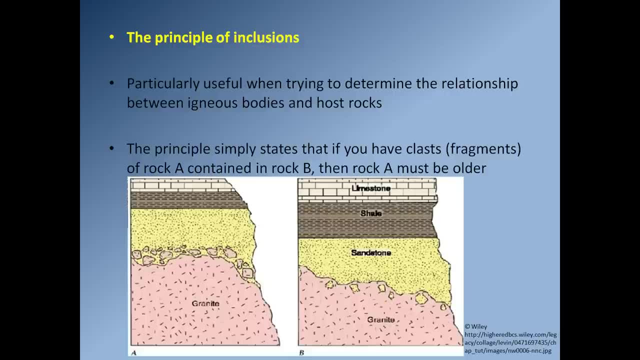 So this is particularly useful when trying to determine the relationship between igneous bodies and host rocks. So the principle simply states that if you have clasts, that's fragments of a rock- let's say rock A contained in rock B- then rock A must be older. 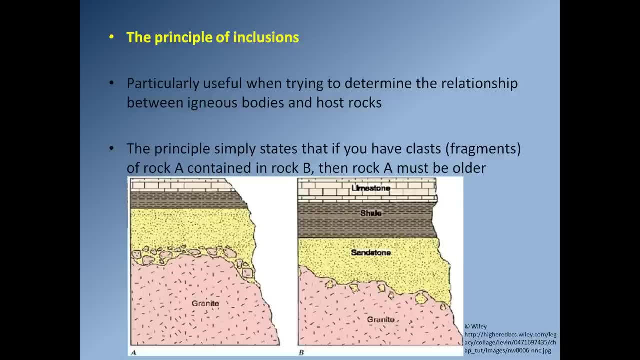 Obviously, if you've got pieces of rock A and rock B, well clearly rock A has to have been there to be eroded so it can be turned into pieces which can then be included in rock B later. So rock A must be the oldest and rock B must be the youngest. 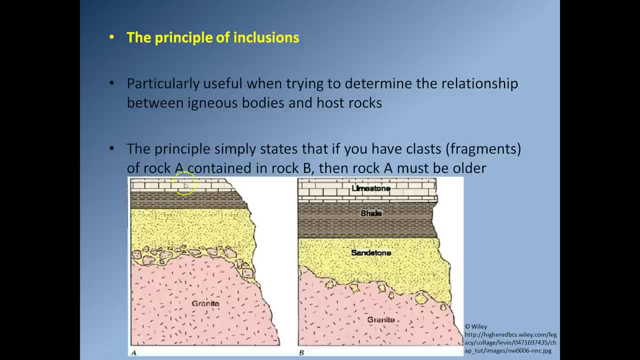 And here's a couple of diagrams that show you how it's useful. So, in this sequence, here we have a limestone, at the top we have some kind of mudstone, we have a sandstone in yellow and we have a granite down here in pink. 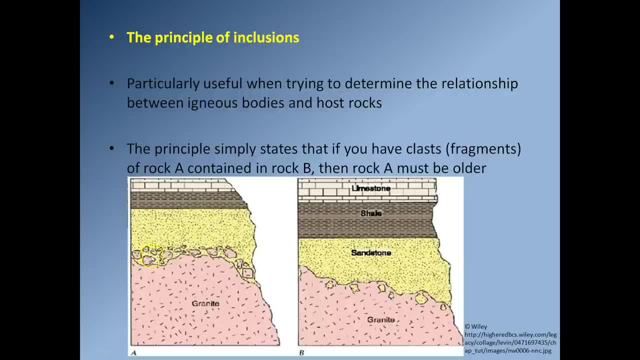 And so what we can see is, in the case of this yellow layer here, this sandstone, we can see that it includes several inclusions of granite within the sandstone. Well, that clearly means the granite must have been there before the sandstone was deposited. 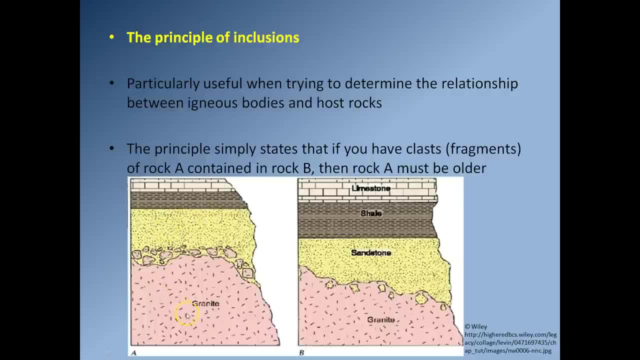 otherwise you wouldn't have pieces of the granite in the sandstone. So it means the granite is oldest, followed by the sandstone, followed by the mudstone, followed by the limestone. So limestone youngest, granite oldest. Now let's look at it the other way around. 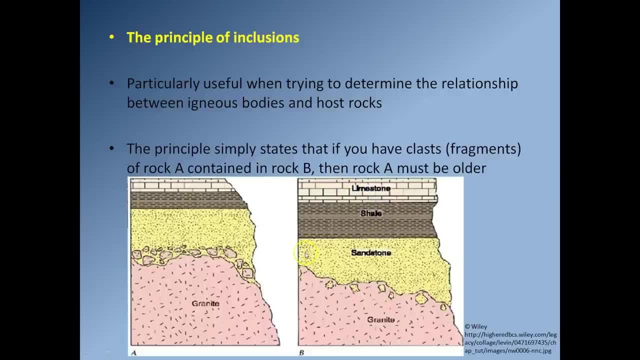 So, once again, here's our limestone, here's our mudstone, our shale, our sandstone and our granite. Well, in this instance, we can see we have pieces of the sandstone within the granite. So what this is telling us is it's telling us: well, the sandstone was clearly there first. 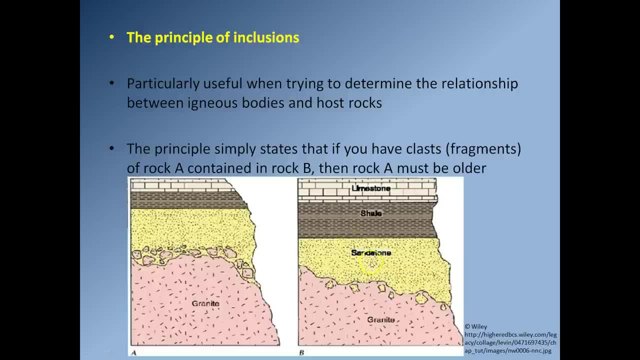 and then the granite went and intruded the sandstone and bits of the sandstone fell off into the granite And we can see those bits that fell off as the inclusions within the granite. So by looking at the inclusions we can clearly tell which rock was oldest and which rock was youngest. 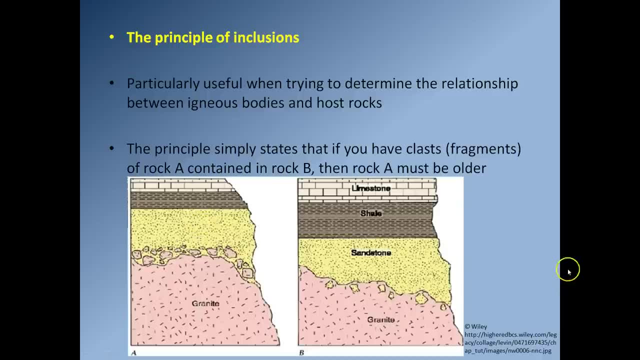 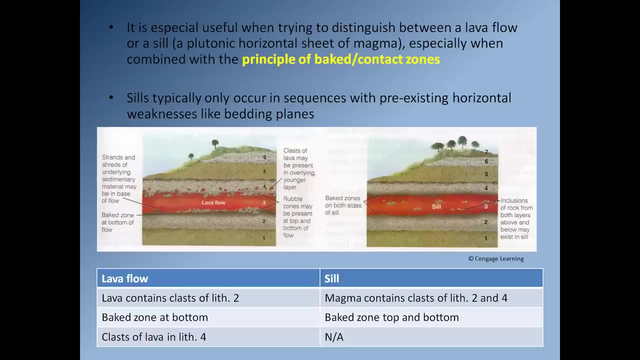 So in this case, this is the oldest, this is the youngest. in this instance, this is the oldest, this is the youngest. So that's the principle of inclusions. So the principle of inclusions is especially useful when it's also combined with the principle of baked zones or baked contacts. 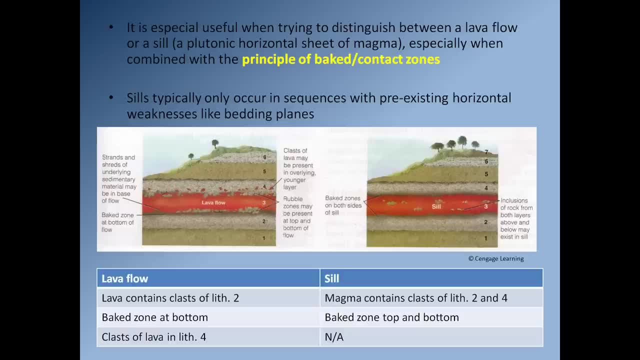 So in the case of baked zones and contact zones, what we have is a situation where when magma intrudes a rock- so let's say when magma intrudes any kind of sedimentary rock- it's going to heat up that sedimentary rock. 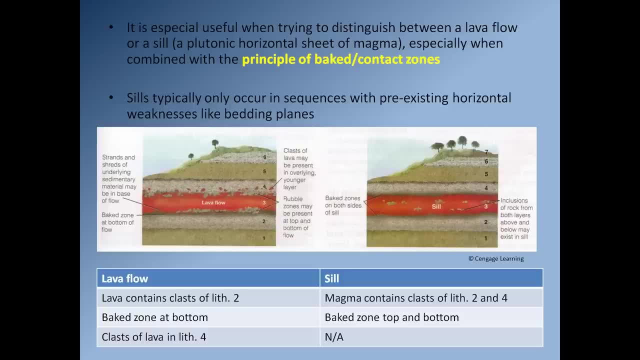 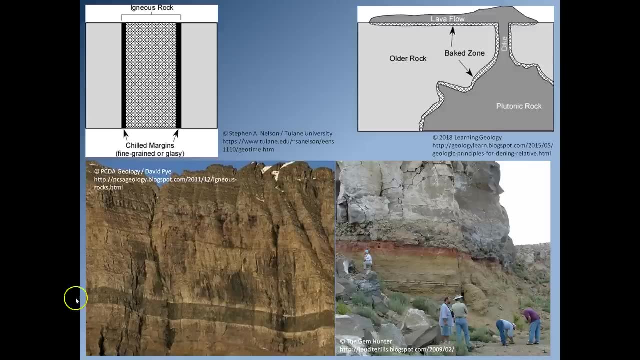 Well, when it heats up that sedimentary rock, it's going to cause the sedimentary rock to change, And so I'm actually just going to skip to the next slide here. So here we go. So here's a sequence of rocks, and you can see you have this thick dark line cutting through it. 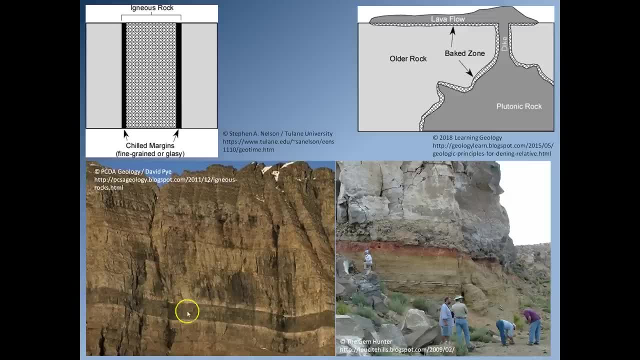 So that's a sill. Okay, so that's when you've had a sheet of magma injected horizontally. Okay, parallel to the layering in a sequence of rocks. The layering is running from left to right here, So this has been injected along the layering between rocks in the sequence. 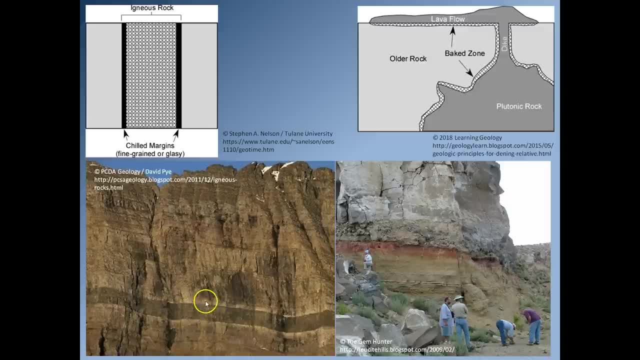 Now what you can see is when you look along the edge of this sill- here you can see these areas either side here and here- are slightly whiter than the rest of the rock sequence. So this change in color is caused by the heat that's coming off the sill. 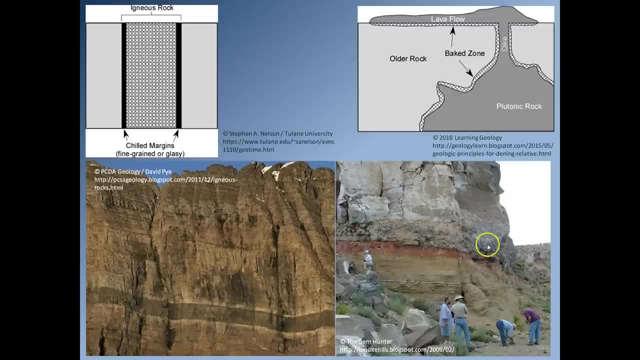 It's baking the rock that it's in contact with, and because it's heating up the rock that it's in contact with, it causes the minerals in the rock to change And therefore it gives the rock a slightly different color. We can see the same thing here. 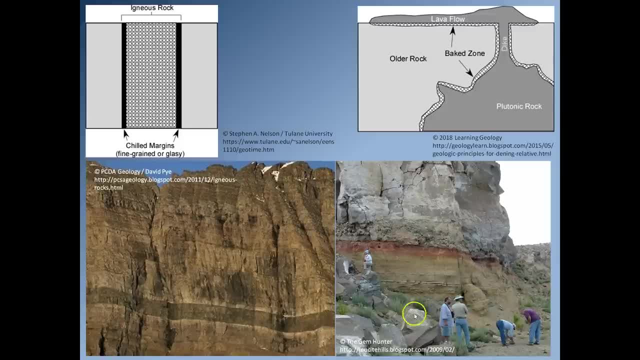 So here we have a sandstone which has got this kind of yellow tan color to it, and above it here we have an igneous rock and the contact between the igneous rock- which would have been liquid magma at one point, so it wouldn't be very, very hot- and the sandstone that would have been comparatively cold. 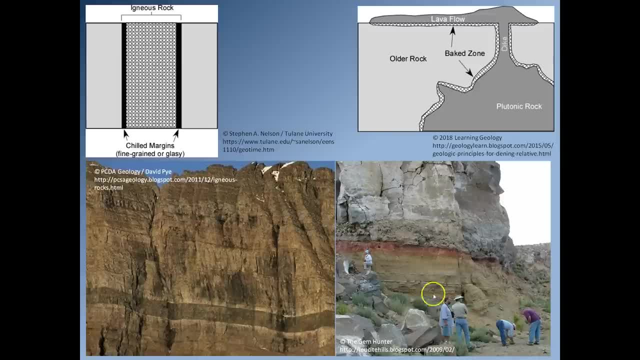 Well, the heat from the igneous rock here has heated up the sandstone below and it's caused this red staining here, this contact zone, which is produced by the heating. Once again, the change in color is the result of the heat coming off the igneous body, heating up the rock that it's in contact with. 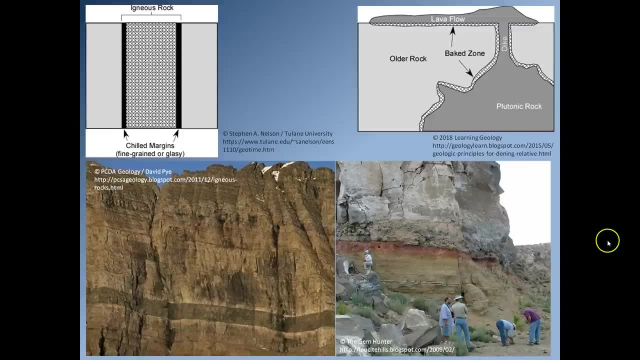 So these baked zones, these contact zones, are extremely useful because if we can see them, well, that clearly tells us which rock is younger and which rock is older. So we can clearly tell that because this igneous rock here has baked this rock above and below it. 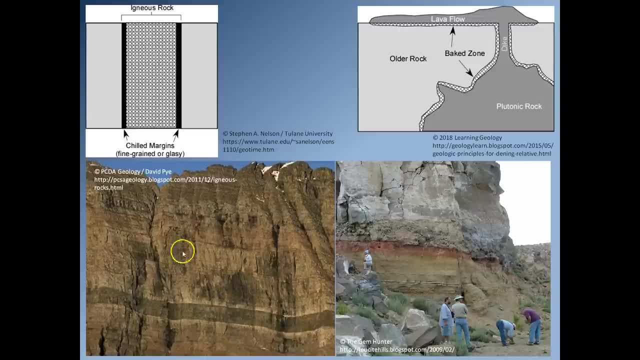 we know it must therefore be younger than the sequences of rock here. and in this case, we know that this igneous rock here- okay- has baked this sandstone here. therefore, we know this sandstone has to have been there first in order for it to be baked when this igneous rock came in contact with it. so the sandstone 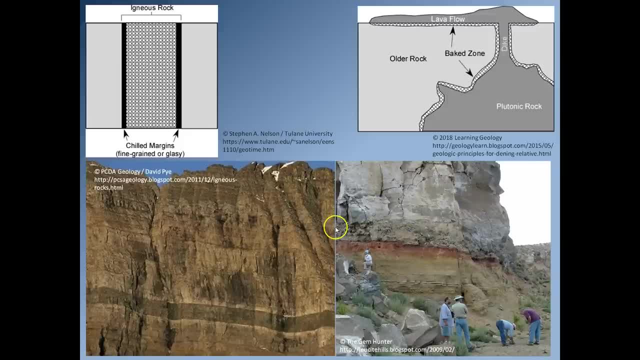 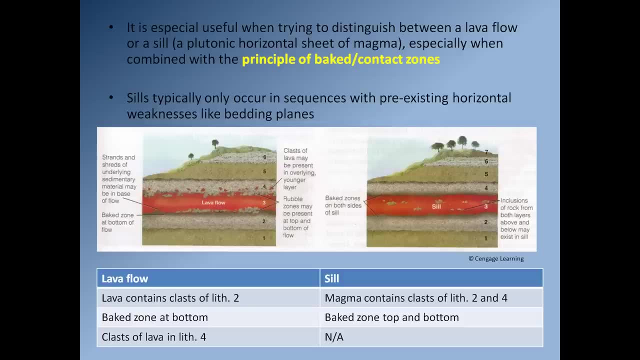 has to be the oldest rock and this igneous rock here has to be the youngest rock. So that's the basis of the principle of baked contacts or contact zones. So why is it most useful? Well, it's useful if we're trying to distinguish. 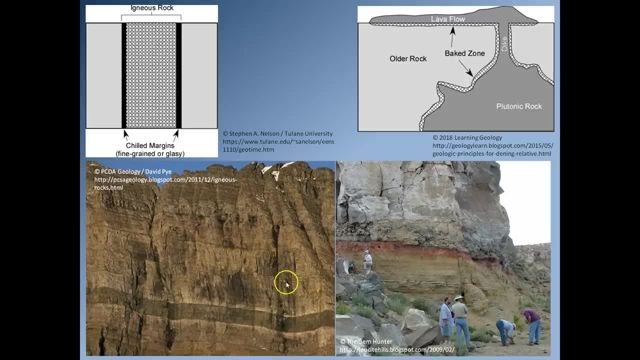 between a sill and a lava flow. So when we look at a sequence of rocks like this, imagine these baked zones weren't there, okay, so you just had a sequence of rocks and as part of that sequence of sedimentary rocks, you have this big, thick layer of igneous rock. 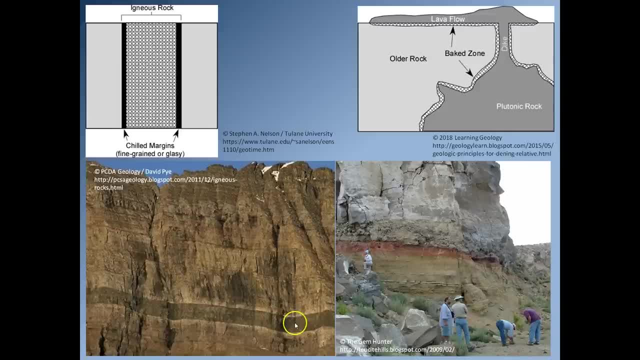 coming across like that. okay. So the question is, is this sequence of rocks deposited and then this igneous rock represents a lava flow, essentially a lava flow moving across the surface of the earth, and then these rocks were then deposited over the top of that lava? 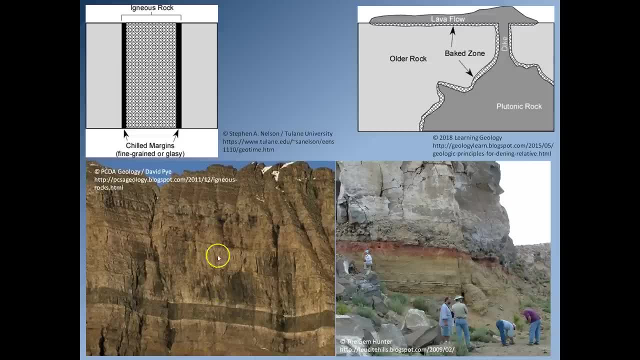 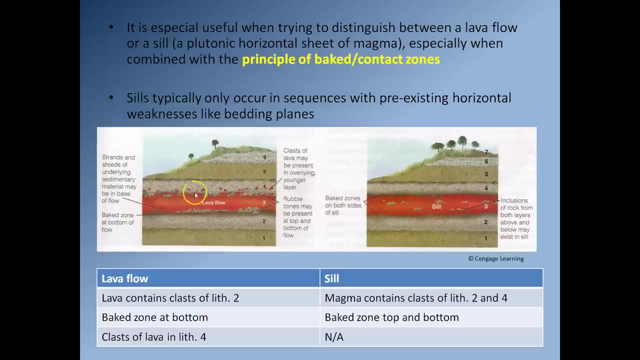 flow, or was this whole sequence of rocks deposited and then the magma was injected as a sill horizontally later? So if you just look you know if you didn't have the baked zones you wouldn't be able to tell. but because we have the baked zones we can work it out. So in this model here, 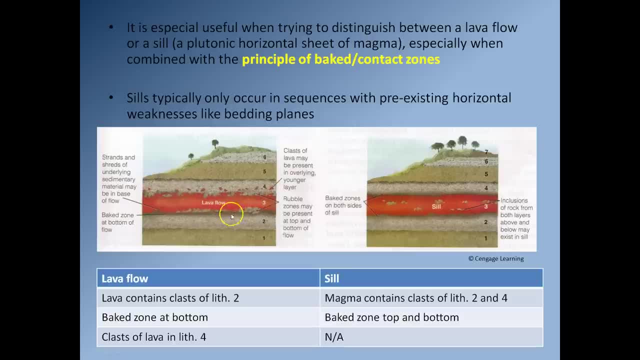 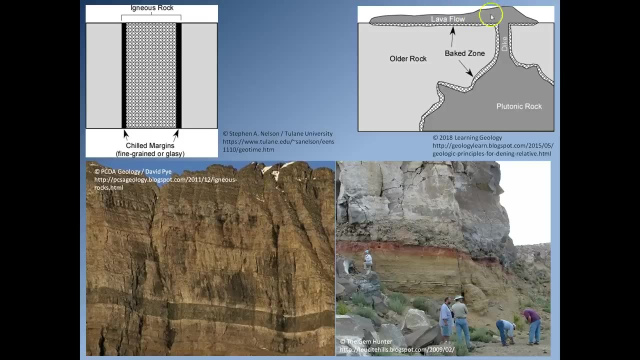 what do we see? So this model here essentially is the model we have for a lava flow. So when we have a lava flow coming out onto the surface of the earth, well above the lava flow, we have air, so there's clearly nothing there for it to bake, So the only thing, the heat from the lava. 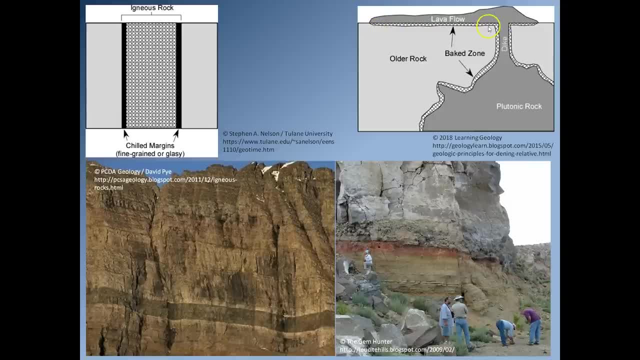 flow can bake is are the rocks directly below it. So when we see a lava flow in a sequence of rocks, we'll see the bottom of the lava flow has a baked contact, but the contact, the upper, the upper edge of the lava flow does not have a baked contact because there was nothing there for it to bake in. 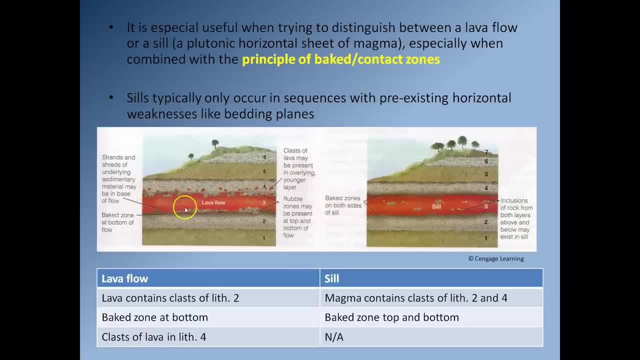 the first place. So that means that when we look at it like this, we'll see a baked zone along the bottom of the rock here, but we will not see a baked zone along the top because there was no rock there to be baked. Also, when we look at the lava flow- number three- here we might see inclusions of number two. that 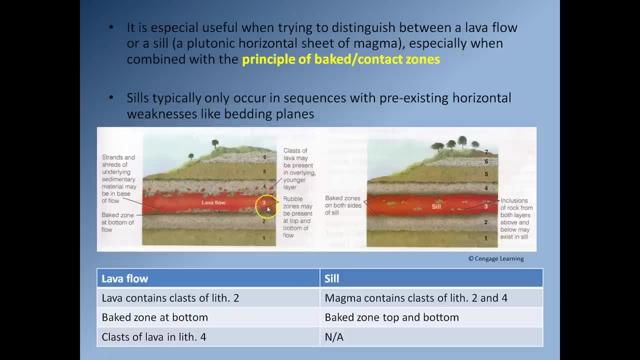 have been included in the lava flow, and we might see inclusions of rock number three in rock layer number four, which was deposited after the lava flow. so there might be inclusions of rock three in rock four, And so this is what we can see here. So here's our sandstone. 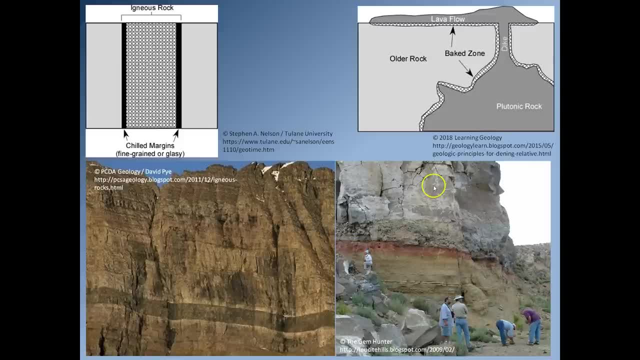 here's our baked contact and here's our lava flow coming across the top. And so the lava flow that's come across the top has gone and baked the rocks directly below it, but because there was nothing above it, there was nothing for it to bake, So there's no. 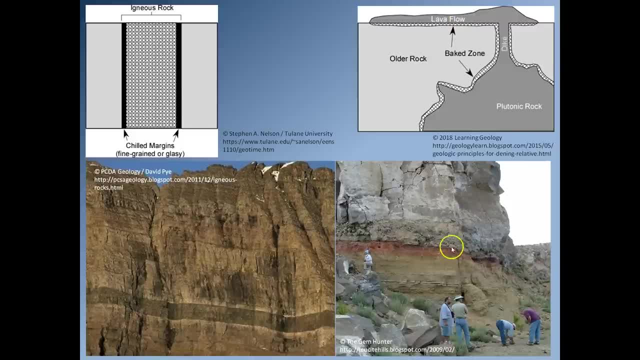 there's no baked zone on the upper edge of this lava flow. We can also see that, if you look, the bottom of this lava flow is rather chunky and blocky, and that's because the lava flow has been moving over this layer of sandstone. it's been pulling off pieces of the sandstone and incorporating 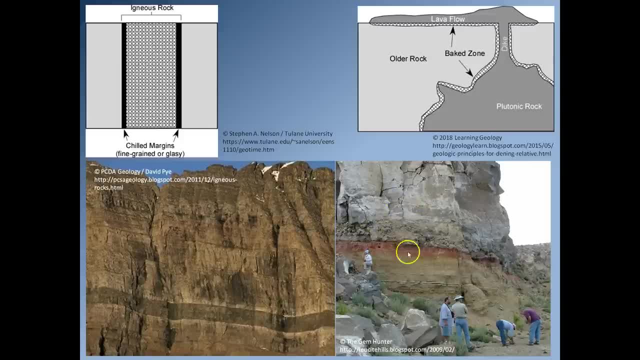 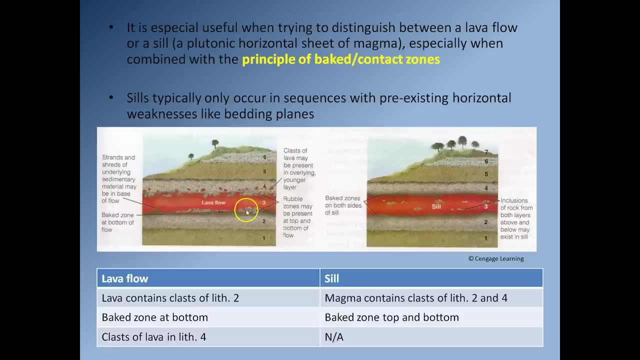 into the lava flow. So what we have here is we have pieces of the sandstone included within the lava flow, so we have pieces of essentially the layer below included within the lava flow, but the lava flow does not include any pieces of the rock that is deposited over the top of it. 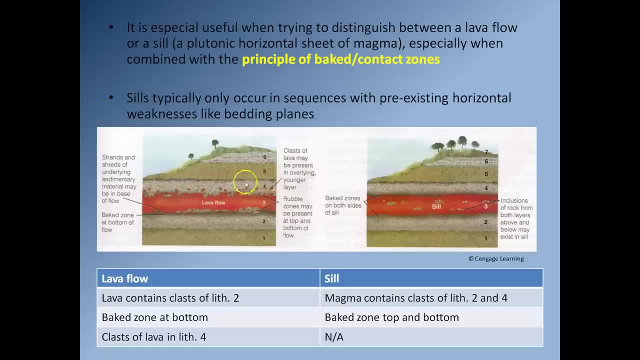 therefore we know the lava flow must have been there first, and then the layer of rock above it was deposited afterwards. So that's how you can identify a lava flow. So then we have a sill, So a sill is injected horizontally. so in this model we have rock. one is deposited, then two. 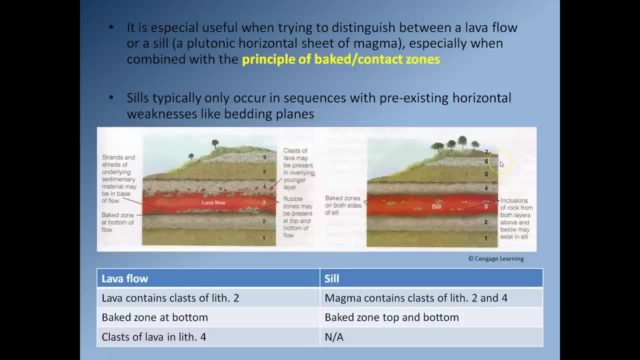 then four, then five, then six, then seven, and then, sometime later on, magma is injected along the contact between two layers and that layer of magma that's injected in becomes a sill when it solidifies and obviously, because the sill is being injected in between two layers of rock, it's going to heat. 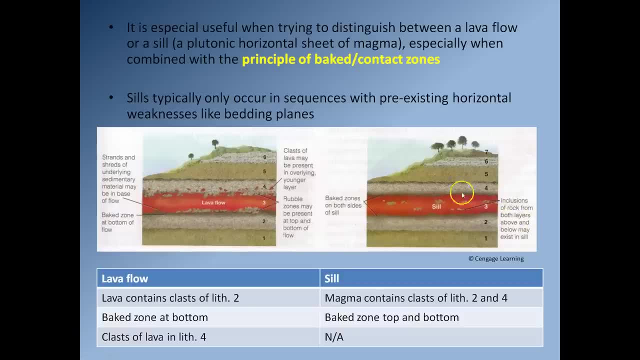 up the rock below, so we have a baked contact down here. and it's going to heat up the rock above, so we have a baked contact up here Now, because layers two and layer four were already there before the sill was injected. it means that pieces of layer number two will fall in and pieces of 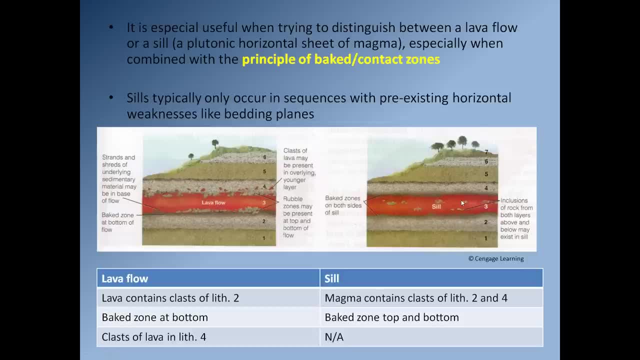 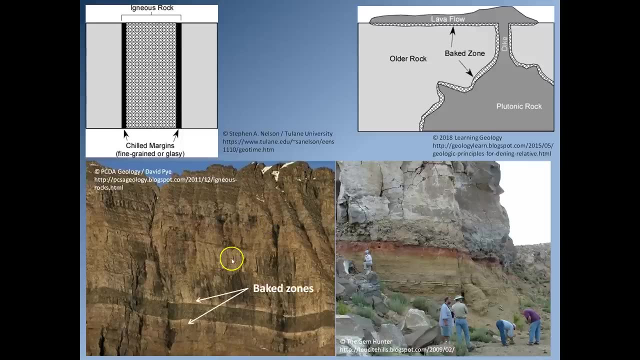 layer number four will fall in, so you'll have inclusions of the rocks above and below the sill within the sill. So here we go. so in this case, we have baked contacts above and below the sill. therefore, we know the sill has to be younger, because we know that. 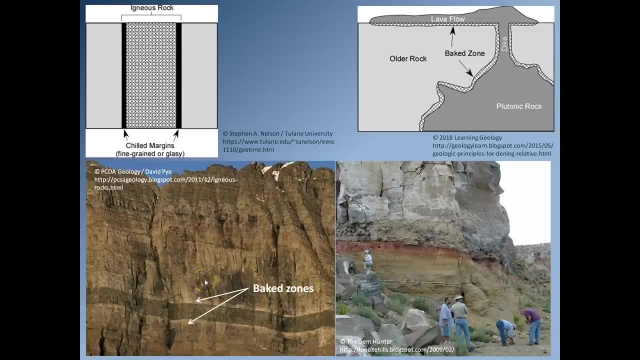 these rocks down here and these rocks up here must have been there before the sill was injected. and I dare say if we looked at this sill here carefully, we could probably see pieces of rocks below and pieces of rocks from above included within the sill. Okay, so sills have baked. 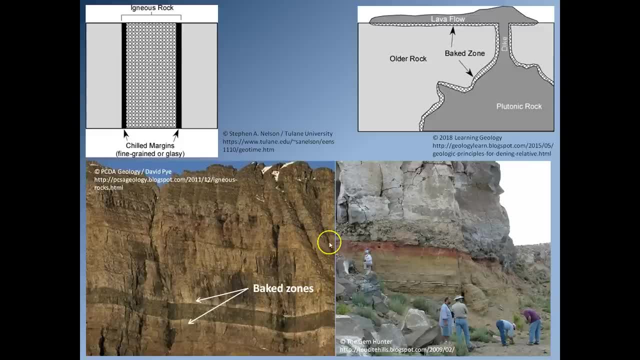 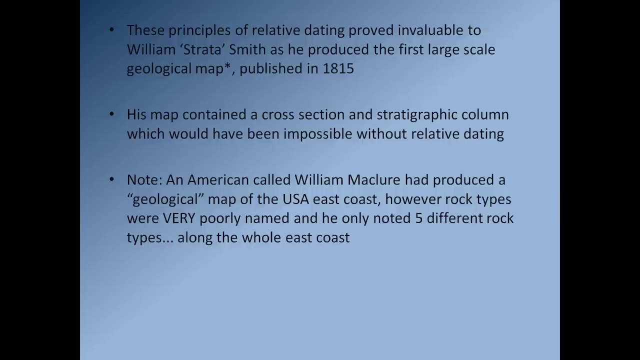 contacts along their top and their bottom, whereas lava flows will only have baked contacts along their bottom, and that's how we can tell the difference. So these principles of relative dating proved invaluable to a gentleman called William Strata Smith, and he produced the first large-scale geologic map in 1815.. So his geologic map was: 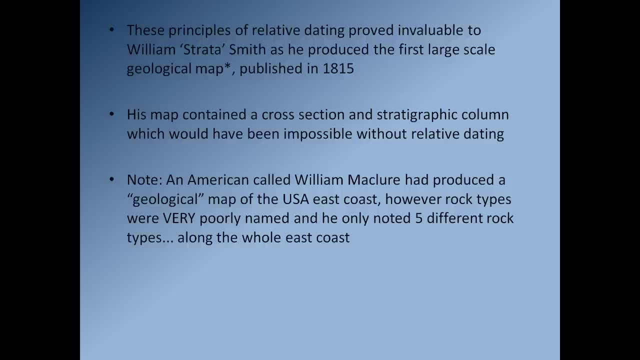 for most of the United Kingdom and it contained a cross-section and stratigraphic column, which, which would have been impossible without relative dating. so he put the rocks that he saw, that were in his map in order: Oldest rocks at the bottom. 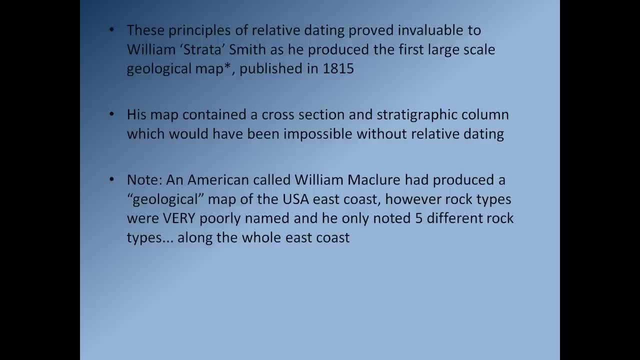 youngest rocks at the top in a sequence which we call a stratigraphic column. We should note that an American called William McClure had produced a geologic map of the the US east coast in earlier, about five years before Smith in fact. but I've got to be honest, the William McClure geologic map is pretty rubbish. So here it is. 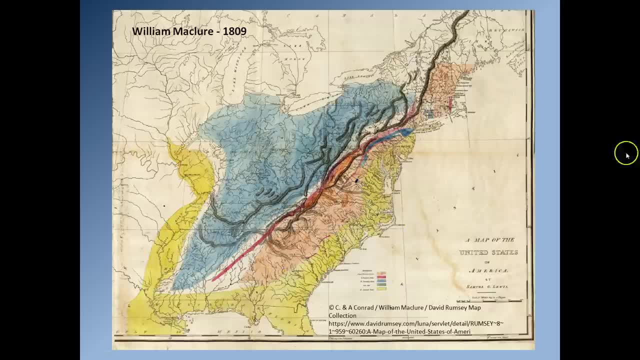 and you can quite clearly see he's got only five different rock types for the entirety of the east coast of the United States and he hasn't really taken much effort, made much effort, to actually name them. Some of them are named the primary unit, some of them named the secondary unit. 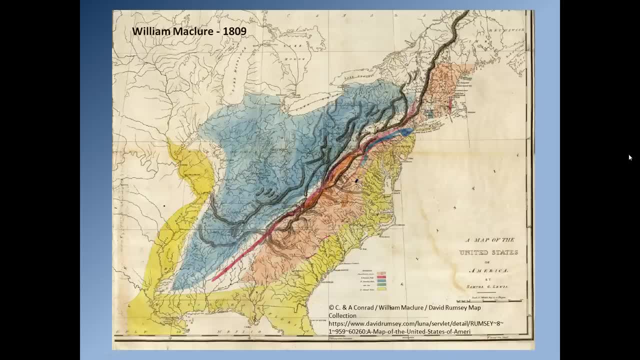 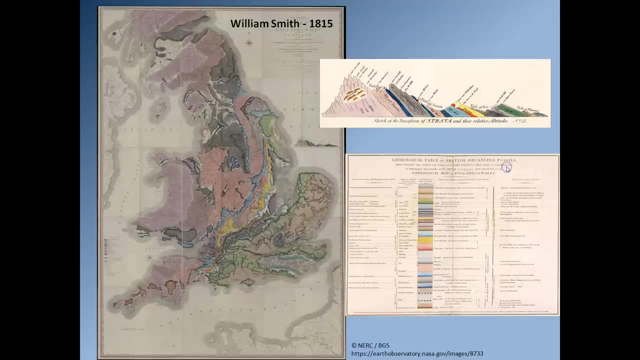 you know, some of them are simply named. you know alluvium. So I'm afraid, as geologic maps go, it's pretty horrendous, it's pretty terrible. In contrast, this is the William Smith geologic map, so you can see what Smith's done is. he's gone over the entirety of England. so there's Wales. 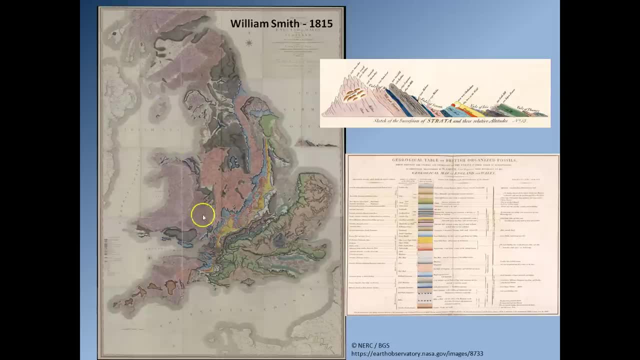 and southern Scotland here and he's mapped to the rocks, he's seen as he goes and he's, you know, given each rock type an individual colour, and because he can work out the relative relationship, which rocks are, which rocks are at the bottom, which rocks are at the top, it's allowed him to. 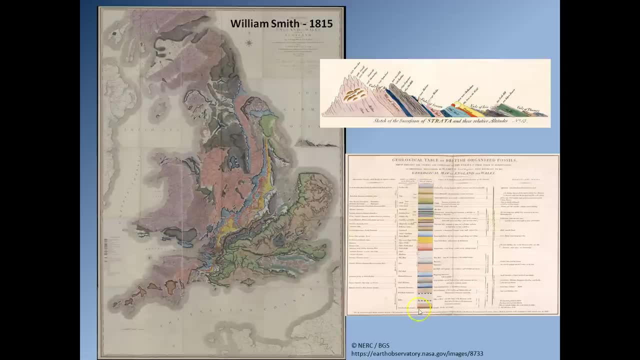 put the rocks into a stratigraphic sequence and the stratigraphic column is colour coded to the rocks on his map. Okay, so you can work out, for instance, you know, let's say, you know this yellow layer here, this kind of orange top. well, that's this layer here and you can work out, you know. 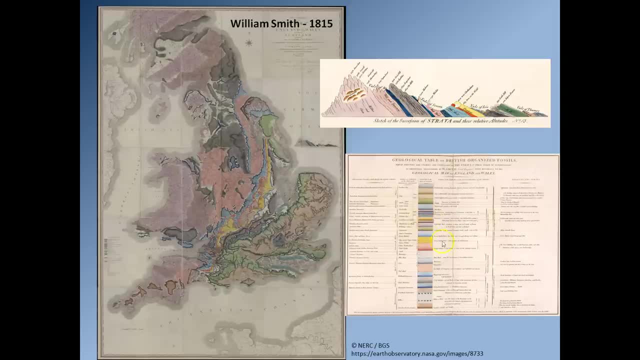 therefore, that's where it sits in the sequence. therefore, all these rocks below it must be older and all these rocks above it must be younger. Now, also because he knows the relative relationship. it also allows him to put the rocks into this. this is what we refer to as a cross-section. Now, it is a 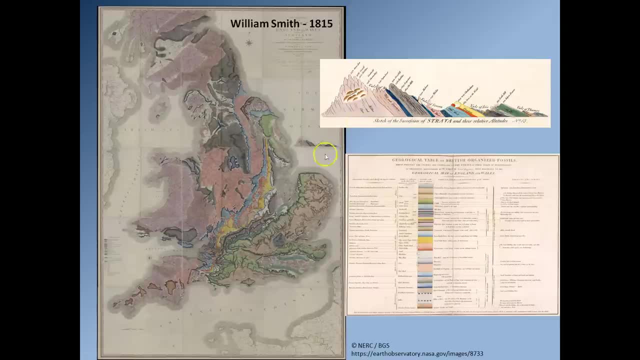 very crude cross-section, but it is a cross-section nonetheless. you can see it actually on the map here and essentially by doing this it allows him to work out the sequence of the rocks and it also shows their lithological relationships, essentially how they're. you know how they lay one. 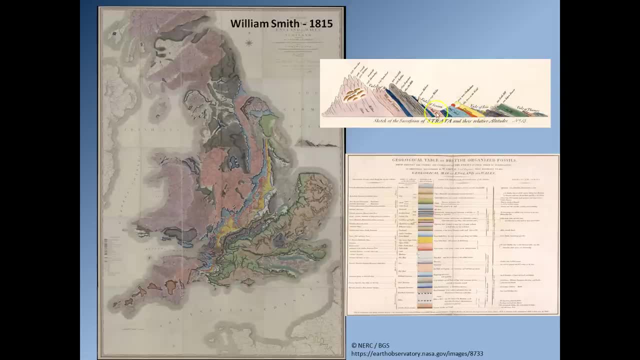 on top of another, and it also shows you the angles at which they are tilted relative to one another and the direction in which they're tilted, which is another important observation which he added to his map. And just to show you just how good this geologic map actually is, 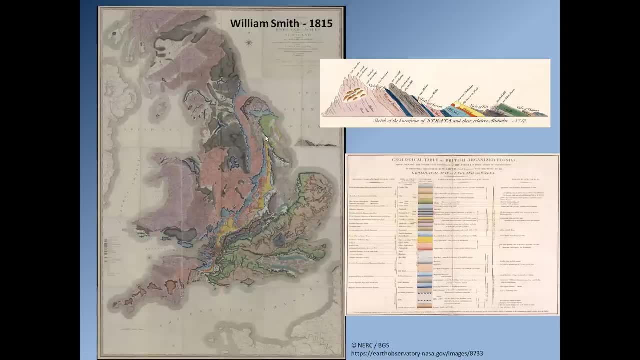 it's actually extraordinarily similar to the modern British geological survey map for the United Kingdom, So this map is extremely accurate and covers a very, very large area. In the case of William McClure's map, yes, it covers a very, very large area, but it covers a very, very large area. 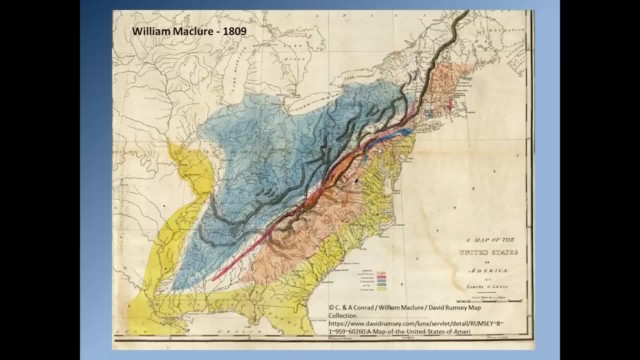 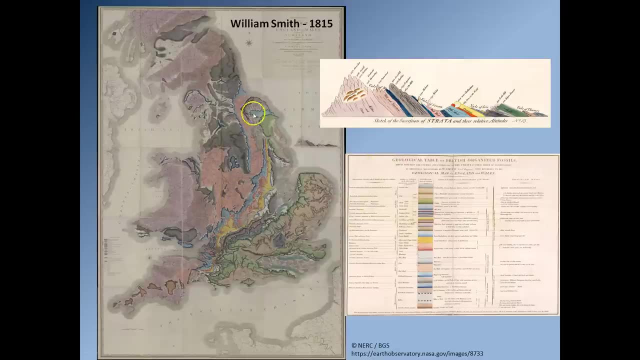 It covers an extremely large area but it's extremely coarse, so there really isn't much information to be gleaned from it. In the case of William Smith's map, you can quite clearly see there is a lot of information there to work with and you know if you remind me during the 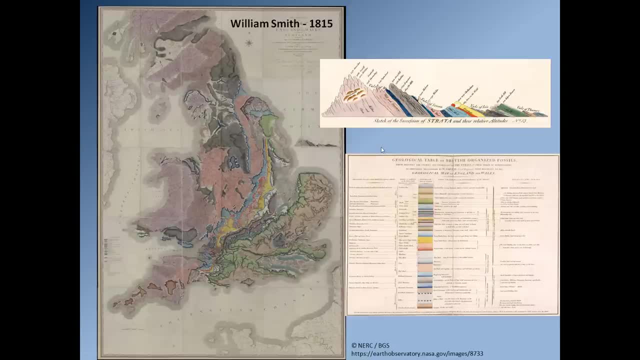 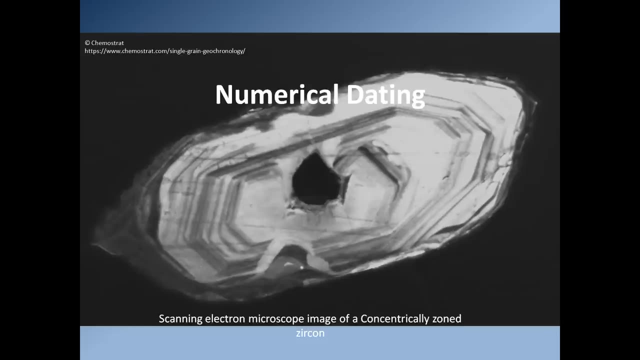 during the lab portion of this class, I will tell you about the life of William Strata Smith, because it was rather interesting. Okay, so this brings us on to numerical dating. So numerical dating uses radioactive isotopes within minerals to date rocks. So we're not. 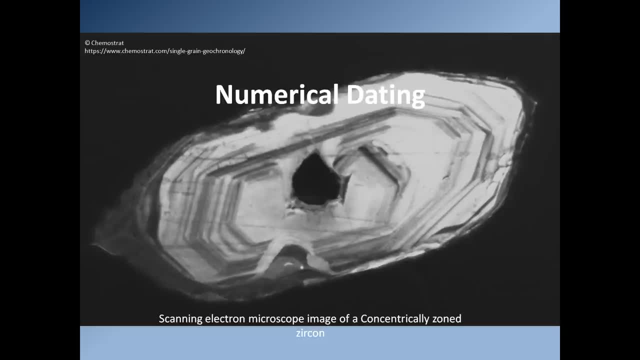 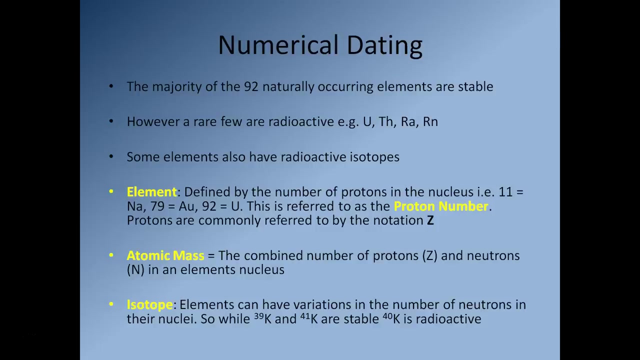 actually dating the rocks themselves. we're dating some minerals within the rocks. So, in this case, this is a scanning that your microscope image of a mineral called zircon, and zircon is one of a few minerals that we can use to date rocks. Okay, so the majority of the 92 naturally occurring. 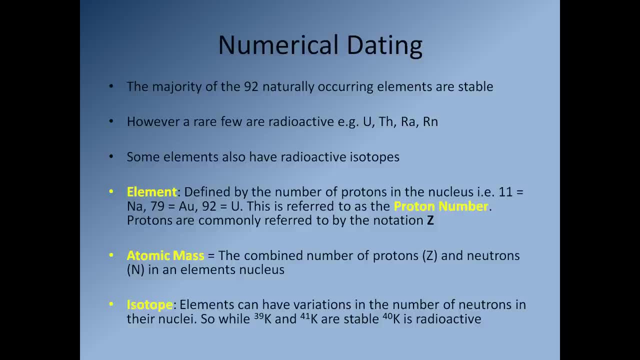 elements are stable. However, a few elements are naturally radioactive and you've probably heard of these. you know you've got uranium, thorium, radium, radon, etc. So some elements also have radioactive isotopes. so some elements on the whole will be stable and not radioactive. 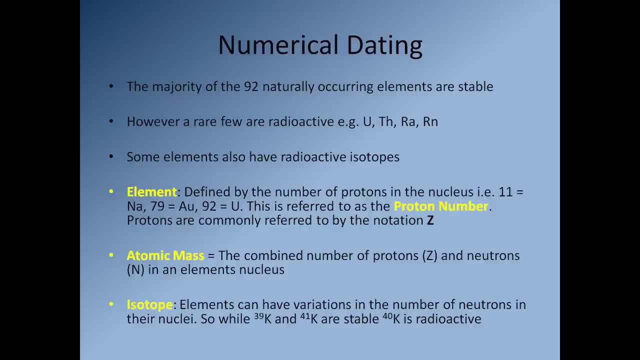 but they might have isotopes, that elements that are radioactive. So an element is defined by the number of protons in the atom's nucleus. So if you have 11 protons in the nucleus, you have sodium. If you have 79 protons in the nucleus, you have gold. If you have 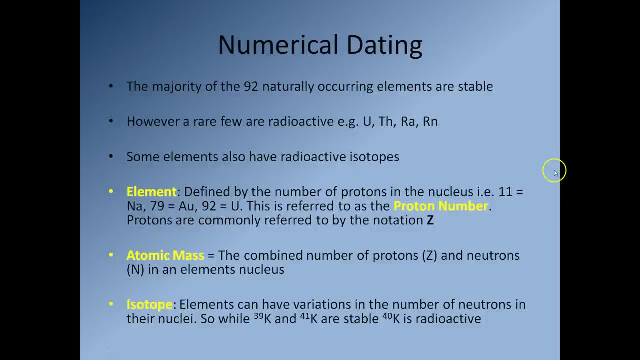 92 protons in the nucleus. you have uranium. So each isotope of uranium will have 92 protons in its nucleus. That never changes. If the number of protons changes, it's a different element. So this is referred to as the proton number. So each element will have a distinct proton number. 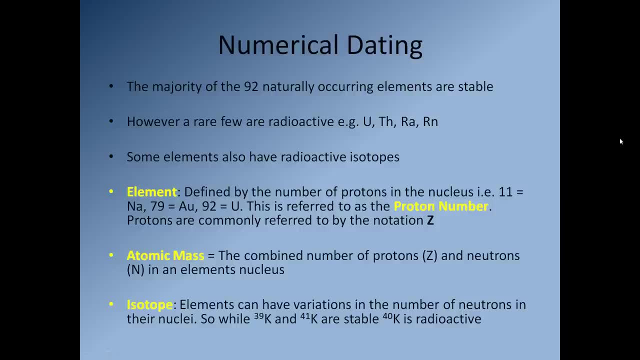 and the protons are commonly referred to by the notation z. So then we have the atomic mass. So the atomic mass is the combined number of protons and neutrons in an element's nucleus. So it's essentially z, the amount of protons, plus n, the amount 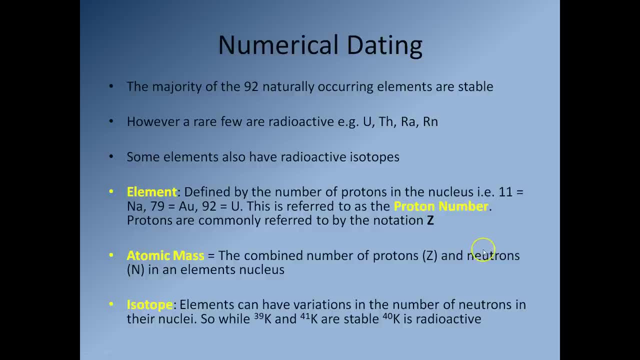 of neutrons in the nucleus and that will give you a number. So an isotope, essentially is when you have an atomic mass. So in this example I'm going to use a number, that is, the number of protons and the amount of 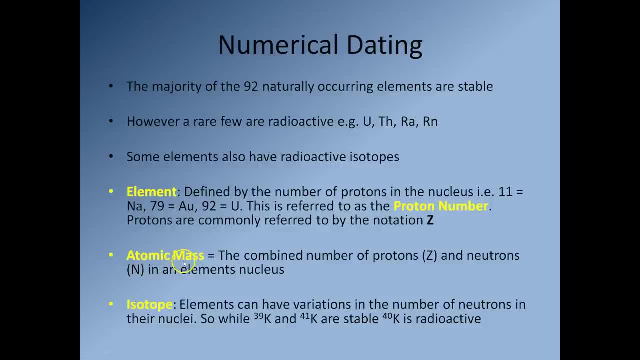 neutrons in the nucleus. So I can see that the number of protons stays the same, but the number of neutrons changes. So we can see that here This is potassium. So here you have potassium 39, potassium 41, and potassium 40. So they're all potassium. So the number of protons has to be. 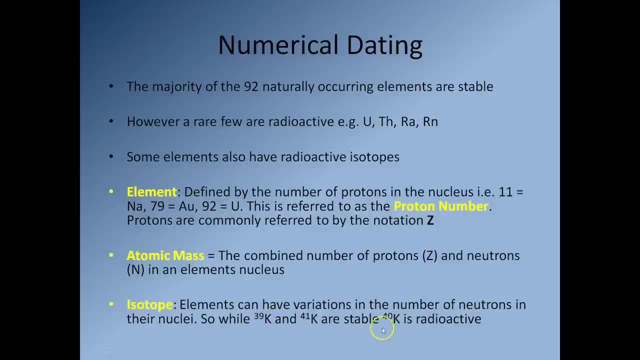 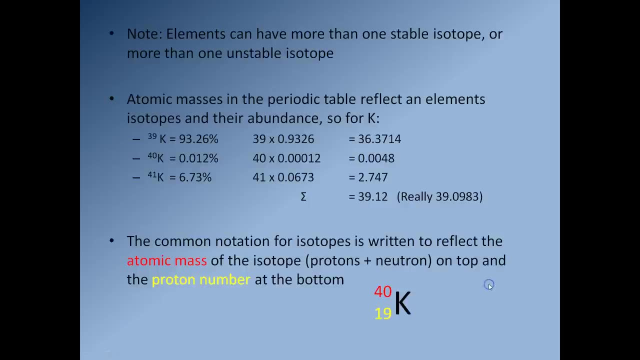 the same for each of these isotopes. However, the number of neutrons is changing and that's why we get these different atomic masses. So elements can have more than one stable isotope or they can have more than one unstable isotope. So atomic masses in the periodic table are reflected in the 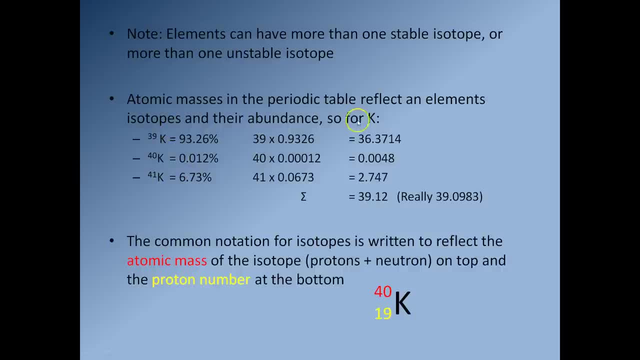 sorry, should I say let's try that one again. Atomic masses in the periodic table reflect an element's isotopes and their abundance. So if you ever looked at a periodic table and you look at the atomic mass for each element, you'll notice in a lot of cases the atomic mass isn't a nice round. 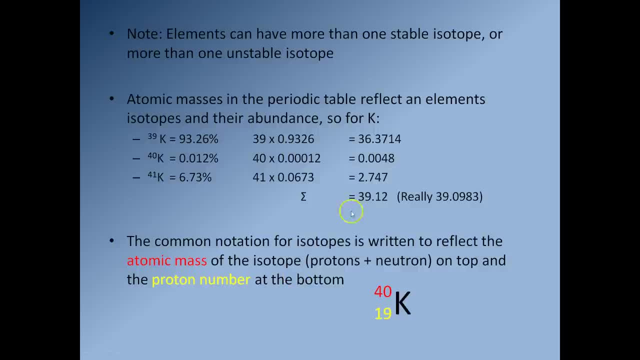 number. It typically is, you know a number, like here, like you know, 39.12.. So what's going on? Well, what it is is we have the different isotopes. so we have potassium 39, potassium 40 and potassium 41. So these are the atomic masses here: 39, 40, 41. And here we have the percentage abundance. so 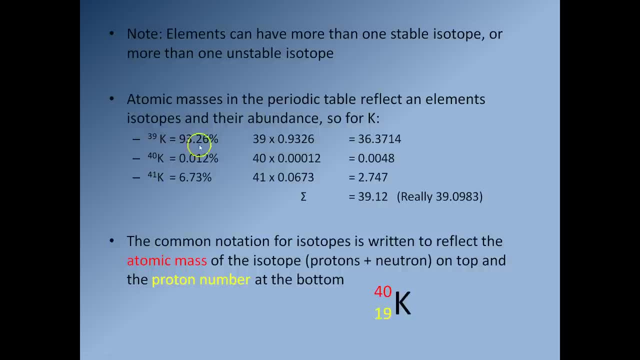 potassium 39 makes up, you know- 93 percent of all potassium. potassium 40, makes up nearly seven percent of all potassium, and potassium 40 makes up a- you know a tiny fraction, And so all you do is you take the atomic mass, multiply it by the percentage occurrence. so 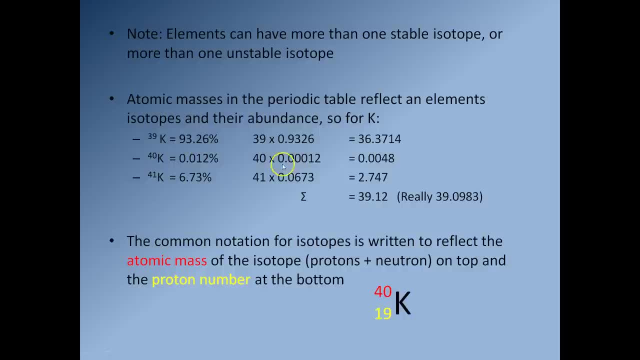 0.93,, 0.06 and 0.00012 and the number you get there, essentially numbers you get here. you add them all together and that gives you the atomic mass for that element. In the case of potassium, this number is slightly wrong. it's actually 39.09.. 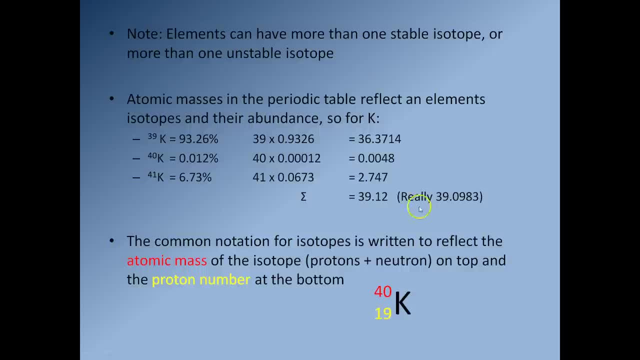 So, but anyway, that gives you some idea about why the atomic masses on the periodic table are nice round numbers. So when we write the information about an isotope, we note the atomic mass and we note the proton number, And when we do this the atomic mass is always at the top, so it 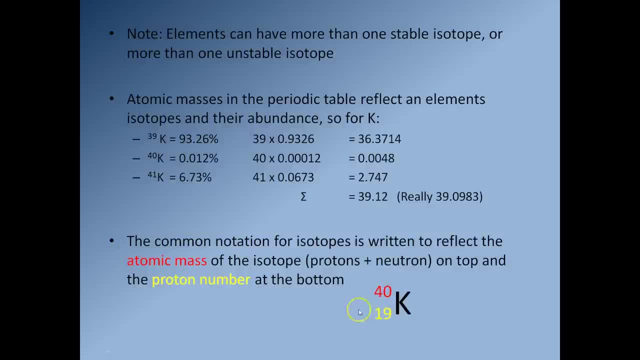 will be the larger number, and the proton number is always at the bottom and it will be the smaller number. Okay, so you'll. so this is potassium. so k is potassium, and k is potassium and k is potassium, So at the top here, this tells us it has an atomic mass of 40, so that's protons plus neutrons and a. 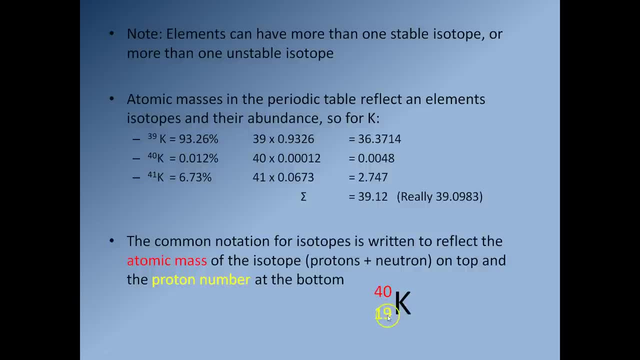 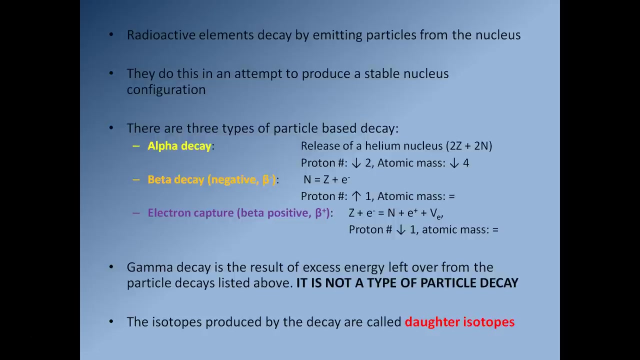 proton number of 19.. And therefore we know that this atom has to consist of 19 protons in its nucleus and 20- sorry, 19- protons and 21 neutrons. Okay, so that's been 20 minutes, so, once again, pause the video. get up, have a walk around, get a glass of water, relax for a couple of minutes. 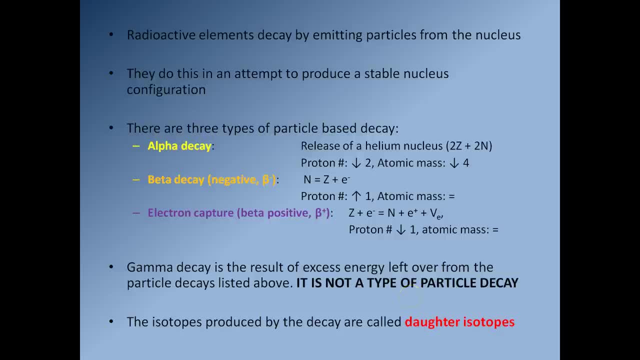 and then come back and we'll do the next 20 minutes. Okay, so the next question is is: if you do have one of these isotopes that is naturally unstable, why and how does it decay? So an radioactive isotope decays because it's trying to produce. 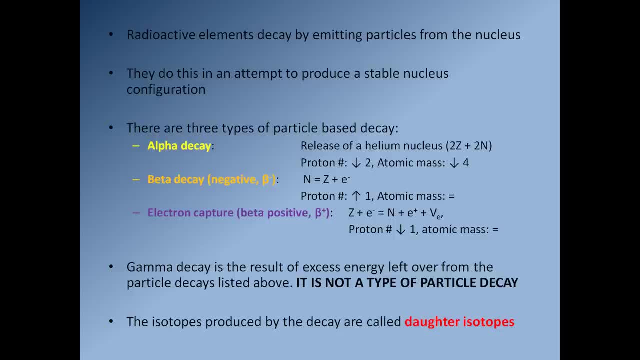 what we refer to as a stable nucleus configuration. So what it has to do is it has to be stable. it has to do is it has to get rid of protons or neutrons from its nucleus to try and make its nucleus stable. And this process of getting rid of protons or neutrons, or changing protons into 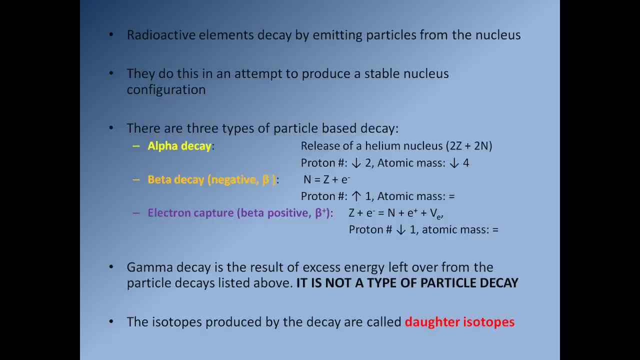 neutrons, or changing neutrons into protons to try and achieve this stability, is referred to us as radioactive decay. So there are three types of radioactive particle-based decay: There's alpha decay and there's alpha decay. So what's alpha decay? Well, in the case of alpha decay, the unstable- 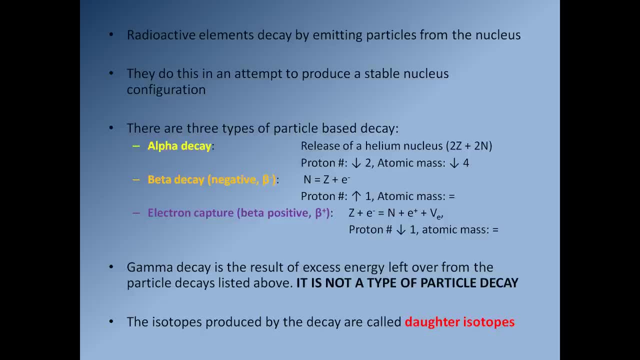 nucleus tries to achieve a stable configuration by getting rid of two protons and two neutrons. That just so happens to be the the nucleus for a helium atom. So helium atoms are two protons and two neutrons. So in the case of alpha decay the nucleus will literally throw away. 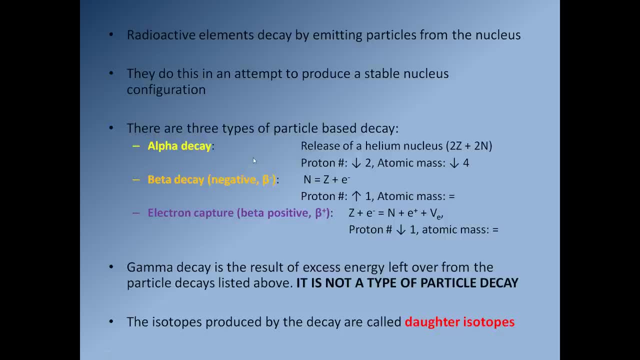 two protons and two neutrons. just it wants to get rid of them in order to try and achieve this stability. And in the case of alpha decay, the nucleus will literally throw away a stable configuration. so that means the proton number for your atom, so your isotope will decrease. 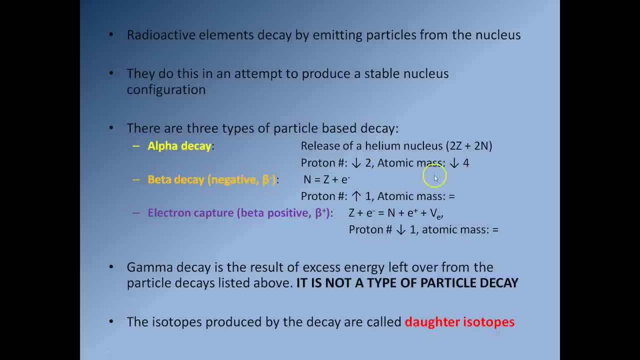 by two and the atomic mass will decrease by four. so obviously, as the proton number has decreased, has changed, you are going to have a new element. in the case of beta decay, we take, we take a neutron and we change it into a proton. okay, so when we take that neutron, we change it into a proton. 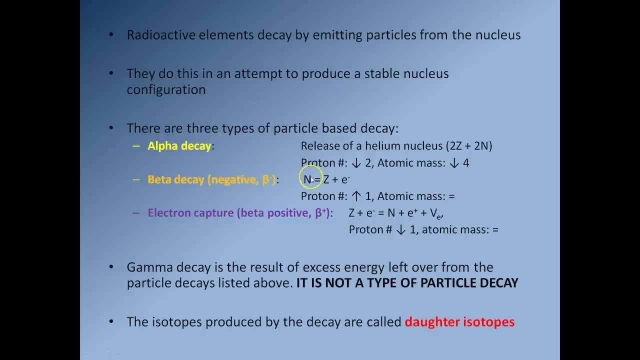 obviously we have a neutrally charged particle being changed into a positively charged particle and that means when this becomes positive we have to kick out a negative charge and that we that is kicked out in the form of an electron. so essentially we have one neutron changes into one. 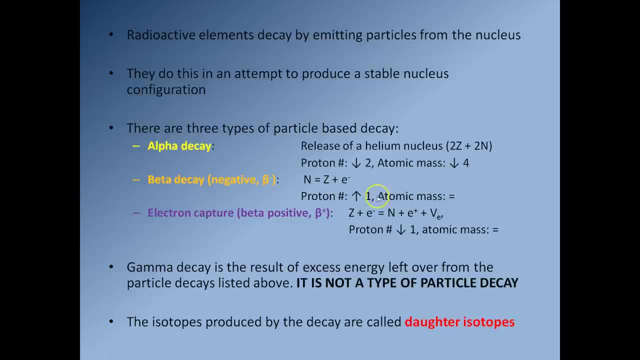 proton. so the proton number will increase by two and the atomic mass will decrease by two, increasing one by one. so we're going to have a new element again because the proton number's changed, but the atomic mass will remain the same, because all we've done is we've taken a proton and we've 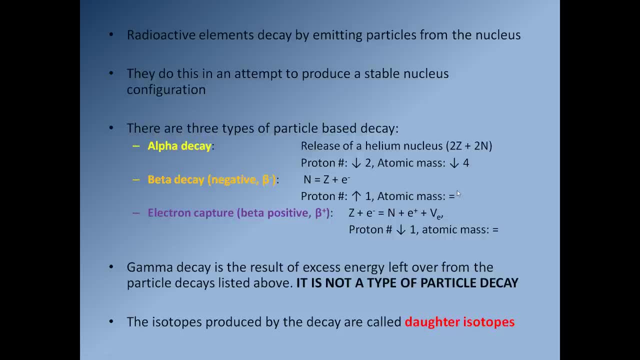 changed it. so we've taken a neutron and we've changed it into a proton. we haven't really changed the atomic with the mass of the nucleus by very much, so the atomic mass is considered to be the same. and then we have electron capture. so in the case of electron capture, we have a proton. 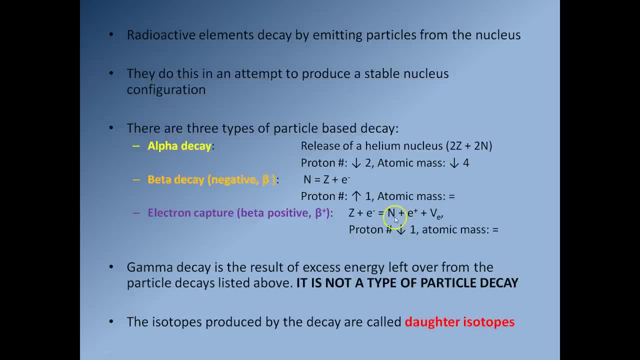 it combines an electron and it gives us a proton. so we've taken a neutron and we've changed it into a proton, so neutron plus a positron, which is this e plus here. so this process takes one neutron and it so it takes one proton, sorry, and it changes it into one neutron. so in this case we have the 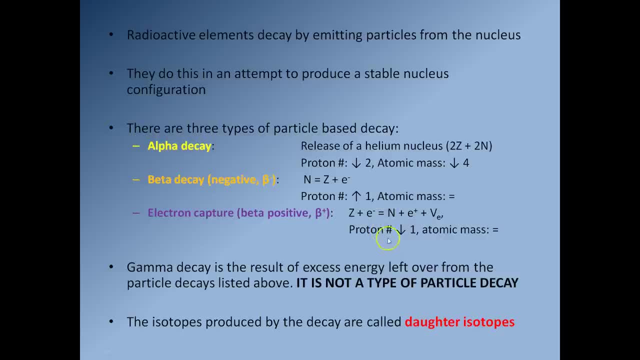 proton number decreasing by one. so once again it's going to be a new element, because the proton number's changed and, just like beta, decay, because all we've done is we've changed a proton into a neutron. we haven't actually changed the mass of the isotope that much, so the atomic mass doesn't. 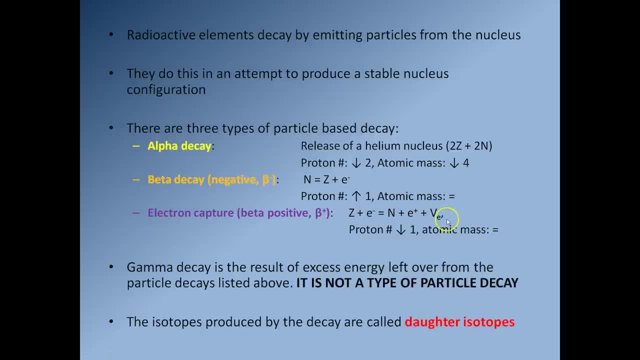 change. now you'll notice that in each of these three instances we have something being lost from the atom. so in this case, we lose one of these helium nucleuses, so two protons plus two neutrons. in the case of beta decay, we lose an electron. in the case of electron capture, we lose one of these. 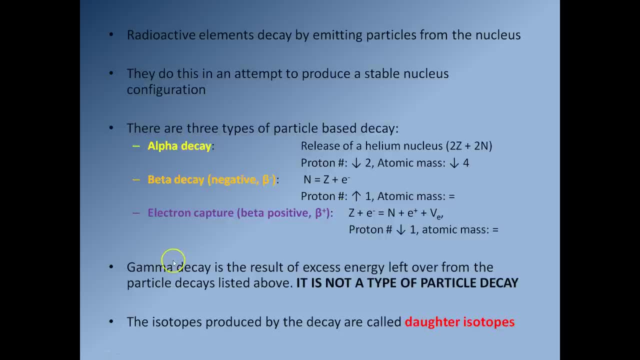 positrons. so in the during the process of radioactive decay they are throwing out these particles. that's what they're referred to as particle decay. now i'm sure there's another type of radioactive decay you'll be familiar with, but i'm not going to go through all of them because 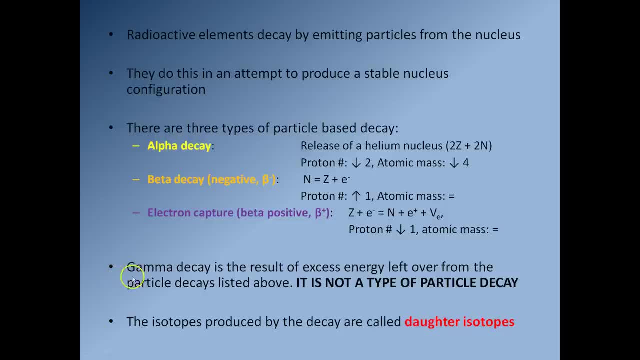 you're familiar with, especially if you've ever read the incredible hulk comics, and that's gamma decay. so gamma decay is the result of the loss of excess energy, and so gamma decay does not lose mass. so gamma decay does not cause the loss of any mass, so no particle is lost. all it is is just. 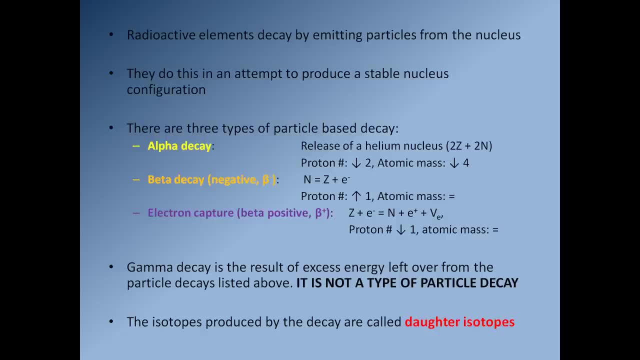 the atom getting rid of excess energy in the form of a electromagnetic wave, a little bit like, you know, an x-ray, for instance. you know, but obviously a gamma ray is a slightly different type of ray. it's not a type of particle decay, because no particle is kicked out of the atom during the 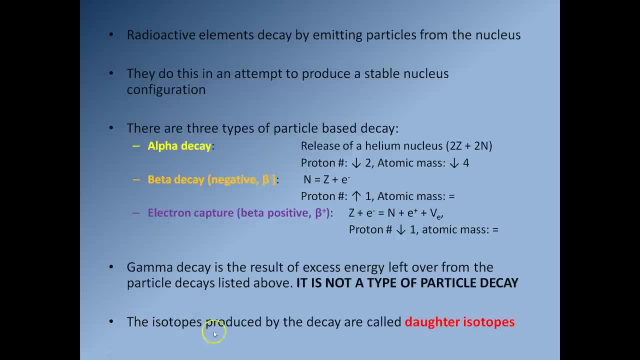 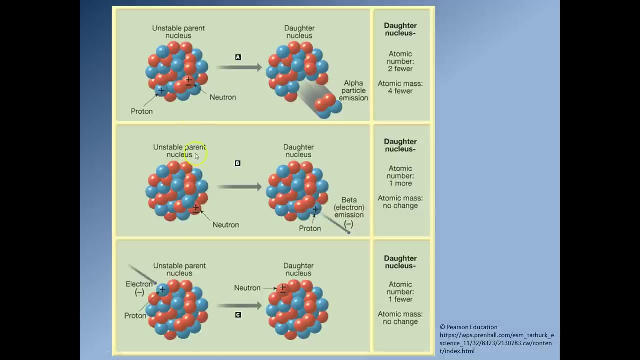 decay. so the isotopes produced by decay are called daughter isotopes. so the starting isotope is called the parent isotope, and the isotope that's produced by decay is called the daughter isotope. so this diagram here kind of summarizes the three types of particle decay. so up here we. 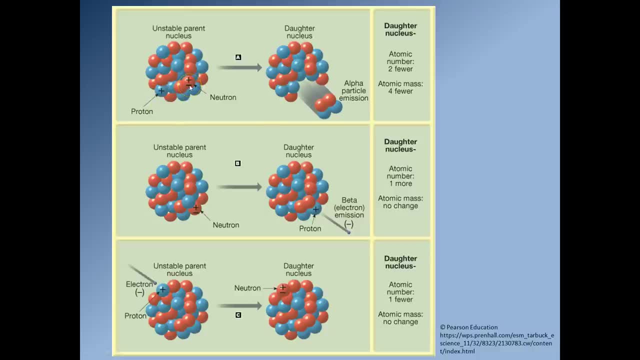 have alpha decay. so in the case, so we have proton decay and then we have gamma decay, and then we have neutrons in blue and neutrons in red. so in the case of alpha decay, you kick out a particle that consists of two, two neutrons, two neutrons and two protons, so it has an atomic mass of four, one, two. 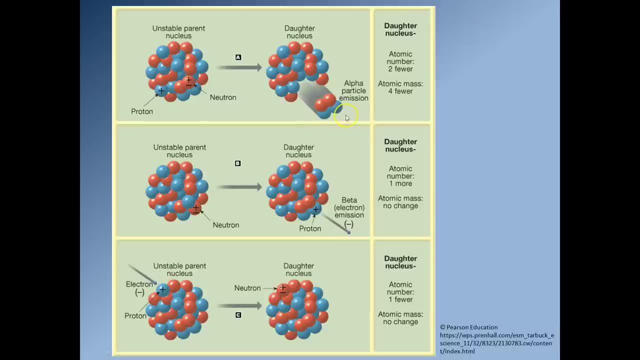 three, four and has a proton number of two. so you have two fewer protons in your nucleus and you lose an atomic. you know, your atomic mass decreases by four during alpha decay. in the case of beta decay, you take a neutron and you take a proton and you take a neutron and you take a proton and you. change it into a proton and you lose an electron as part of that process. so in this case, the proton number has increased by one because we've changed a neutron into a proton, but the atomic mass does not change. in the case of electron capture, we have a proton combining with an electron to give us a 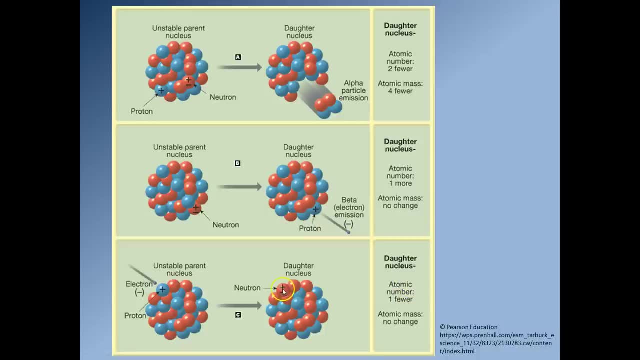 neutron. so in that instance the proton number has decreased by one because we've lost a proton. but once again the atomic mass does not change, because all we've lost is a proton. so in this case we've done is change a proton into a neutron, so there's practically no change in the atomic mass. 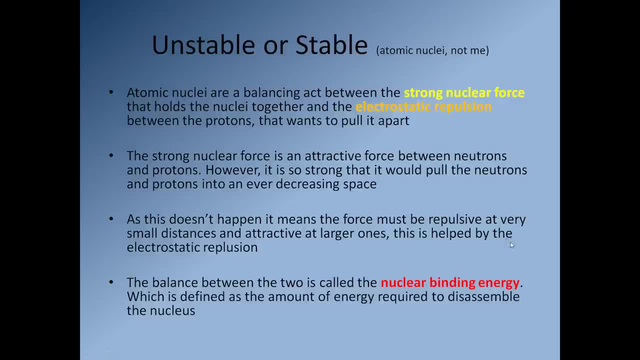 so the next question is is: well, why are some isotopes stable and why are some isotopes unstable? so atomic nuclei are a bouncing act between two forces. there's the strong nuclear force that holds the nucleus together and there's the electrostatic repulsion between the 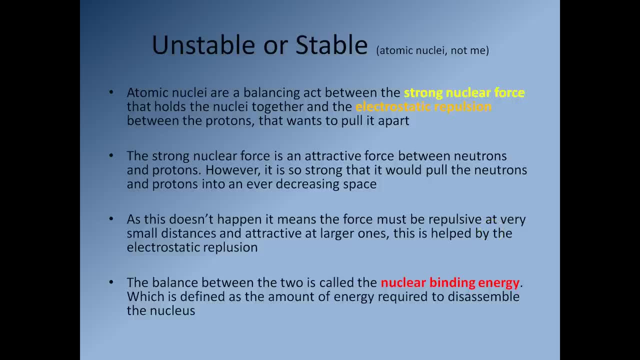 protons. that wants to pull the atom apart, or should i say the nucleus apart. so the strong nuclear force is attractive, so it's like gravity, so it wants to keep pulling the protons and neutrons in the nucleus into a smaller and smaller and smaller space. it wants to keep pulling them. 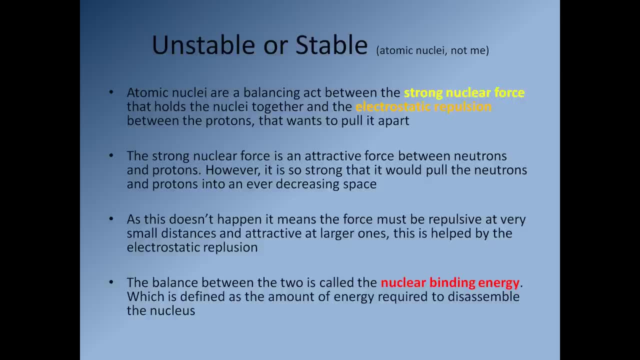 into a tighter and tighter sphere. however, it is so strong that it would pull the neutrons and protons into an ever-decreasing space if it could. as this doesn't happen, it means that there has to be a magic point where you pull the protons and neutrons so close together that they actually 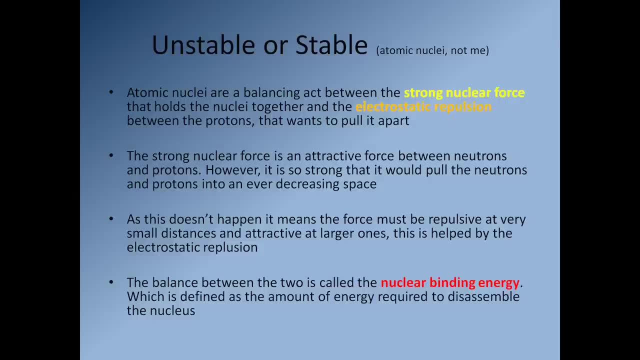 begin to repel each other. so that stops the nucleus, you know, being pulled into a smaller and smaller space. so there's also electrostatic repulsion. so if you imagine taking the negative end of two bar magnets and trying to push them together, well i'm sure you know if you try and push the two negative. 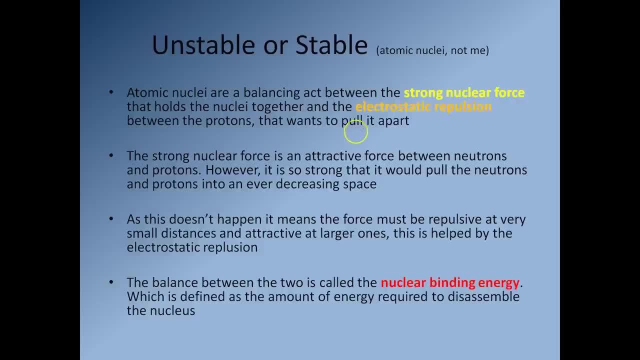 ends of bar magnets together, they repel each other, don't they? so that's the kind of situation we have with protons. now, in the case of the protons, they're not the same as the protons. they're not the same as the protons. it's like pushing the two positive ends towards each other. when you push a proton, 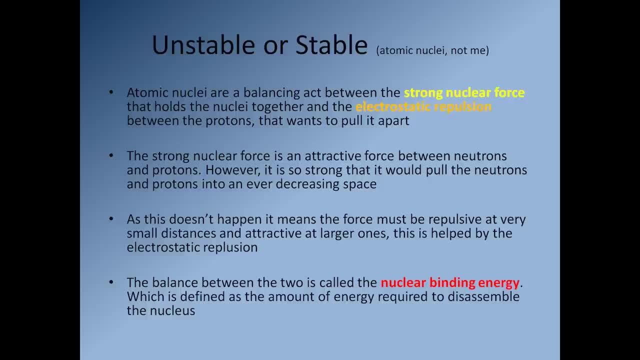 towards a proton. they both have a positive charge, so when they get close enough, they'll begin to repel each other, and so that's the balancing act you have in your nucleus. the strong nuclear force is trying to pull the nucleus into an ever smaller space, whilst the electrostatic repulsion between 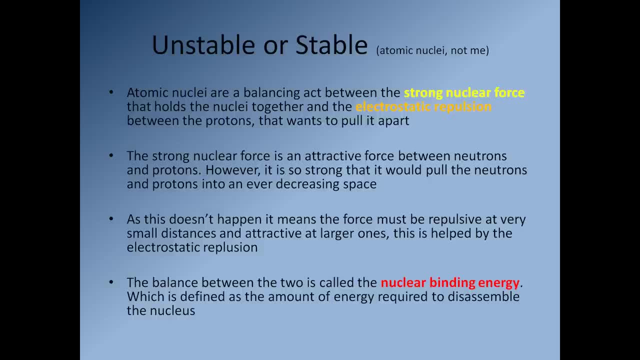 the protons, is trying to push the protons further apart, and so your nucleus has to be very, very carefully balanced or things are going to start going wrong. so this balance between the two is called the nuclear binding energy, and that's defined as the amount of energy required to disassemble the nucleus. so once you exceed the nuclear binding, 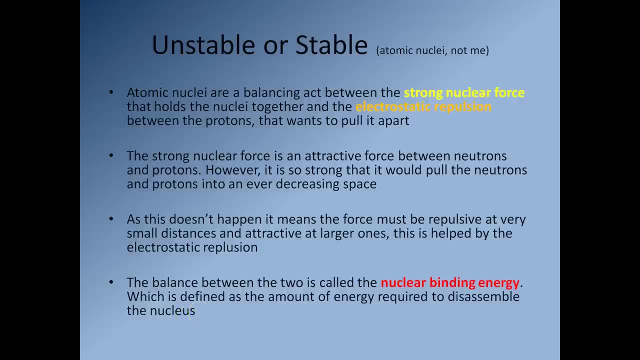 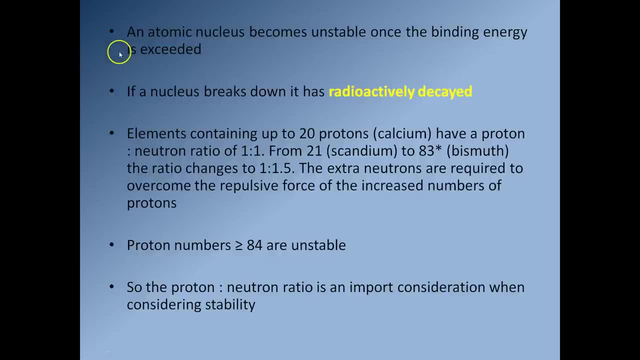 energy, the nucleus will naturally start to fall to pieces. so an atomic nucleus becomes unstable once the binding energy is exceeded, as i just said. so if a nucleus breaks down, we refer to it as radioactive decay. but what can we do to stop this from happening? so if a nucleus breaks down, we can see these two. 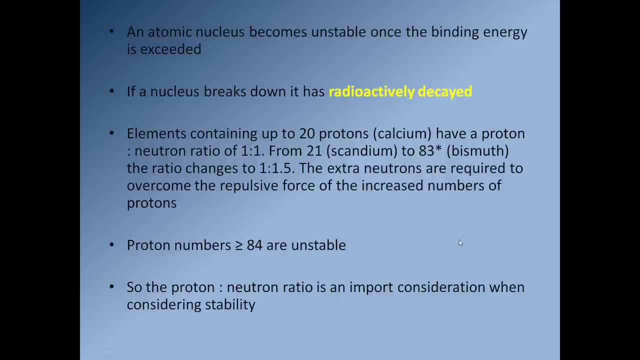 protons that are on the nucleus have a ratio of 1.5 neutrons and the protons containing up to 20 protons- that's from hydrogen to calcium- have a proton ratio of 1 to 1. so for every proton in the nucleus you have 1 neutron. from 20 protons to 83 neutrons, so that's from scandium to bismuth. 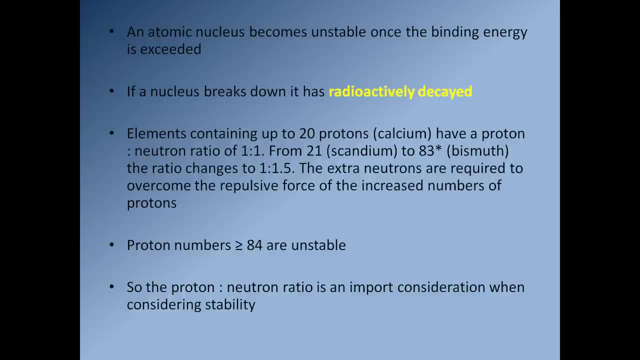 you have a ratio of: for every one proton, you have to have 1.5 neutrons, and so the extra neutrons are required to overcome the repulsive forces caused by the increased number of protons. so as the number of protons and the protons goes up, you have to have more neutrons to pack in between them to stop the protons. 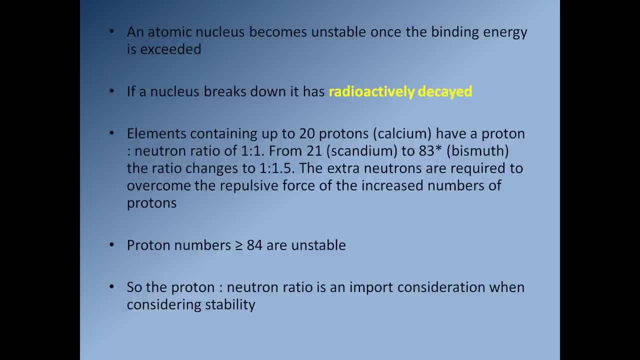 repelling each other, and so that means that, as I just said, once you have more than 21 protons, you need to add more and more and more neutrons to make sure this repulsive force doesn't become too strong, because if the repulsive force becomes too strong, it's going to start pulling the nucleus. 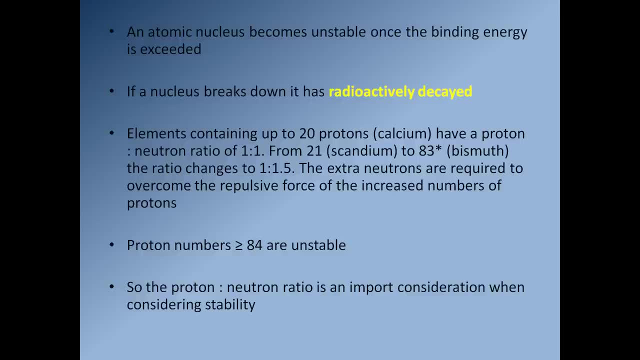 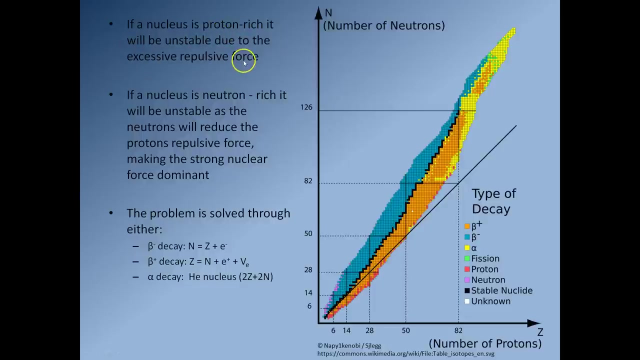 apart Protons. proton number in excess of 84 is unstable and those elements will naturally be radioactive. So the proton to neutron ratio is important when you consider the stability of a nucleus. So if the nucleus is proton rich it will be unstable due to the excessive repulsive force. 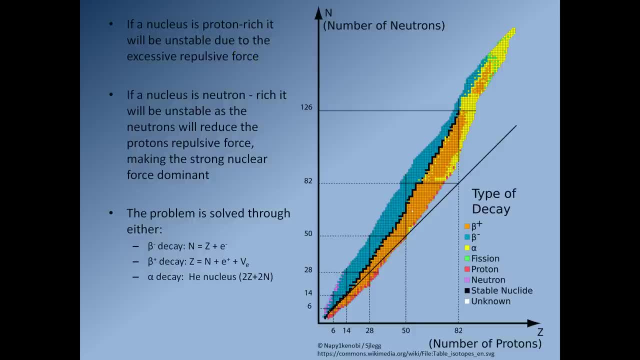 If you have too many protons, well, those protons are going to be pushing each other away, and so your nucleus will be unstable. So if you have too many protons, well, those protons are going to be nucleus is going to be unstable because it's going to have too much of this repulsive force. 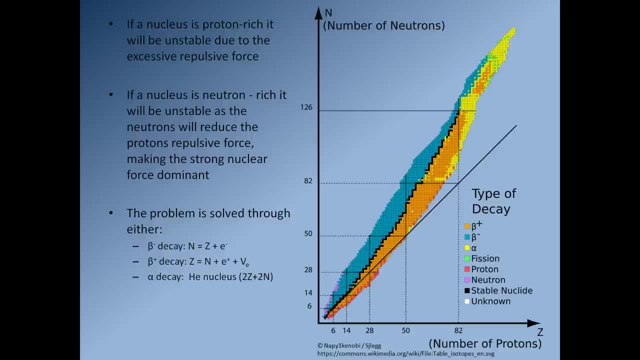 trying to rip the nucleus apart. In contrast, if your nucleus is too rich in neutrons, it means that you'll have so many neutrons that the protons won't be repelling each other very, very well, and so that means this strong nuclear force will be dominant and it will be trying to pull the 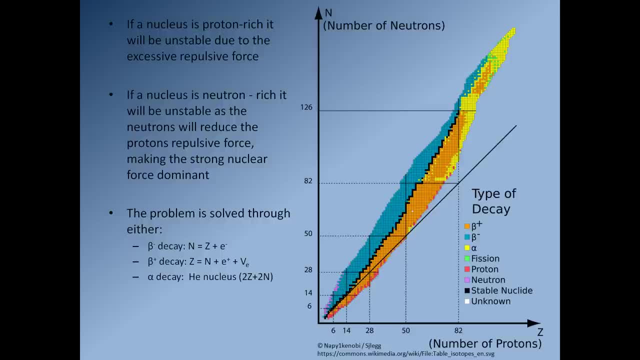 nucleus into an ever smaller and smaller space, and once again, once the nucleus gets pulled into too small a space, it's going to become naturally unstable, and so that's why you have to have just the right amount of protons and neutrons to keep the nucleus balanced, and if you don't have that, 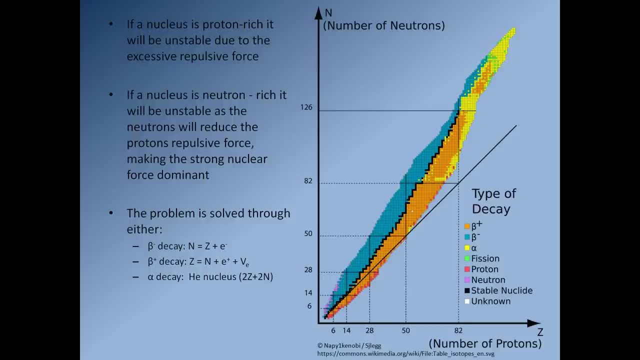 incorrect ratio. well, the nucleus is going to be naturally unstable and it's going to want to try to achieve that stable configuration. So this diagram here kind of shows you what's going on. so each of these squares represents isotopes. okay, so we have the number of protons here. 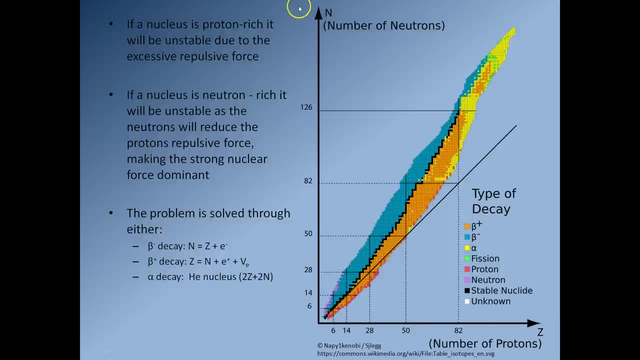 and we have the number of neutrons and we have the number of neutrons and we have the number of neutrons on the x-axis and the number of neutrons here on the y-axis. Now, these black squares here represent stable nuclei. okay, so these are elements, isotopes, that will not naturally decay. okay, they're. 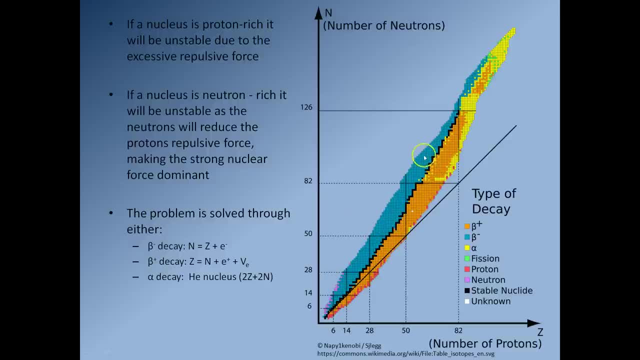 stable. Once you go above this line, you go into this blue field here, and these are nuclei that will decay through beta decay, so that's when you take a neutron and you change it into a proton. Okay, so that means essentially, up here you have too many neutrons in your nucleus, and so this: 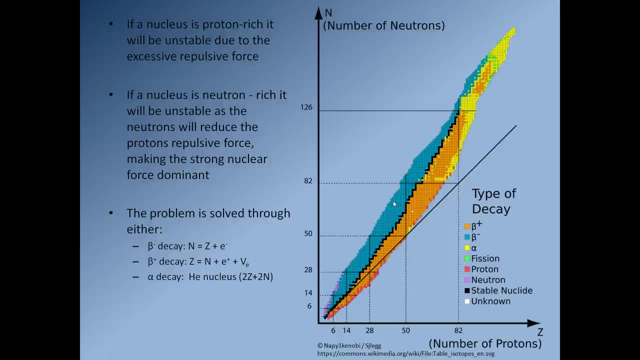 strong nuclear force is dominating and it's pulling the nucleus into a smaller and smaller and smaller space, and so the nucleus becomes unstable, and so it gets around this instability by simply changing neutrons into protons, and so that increases this, so that will increase the repulsive force and once it, you know, and it will help to balance out this strong nuclear force. 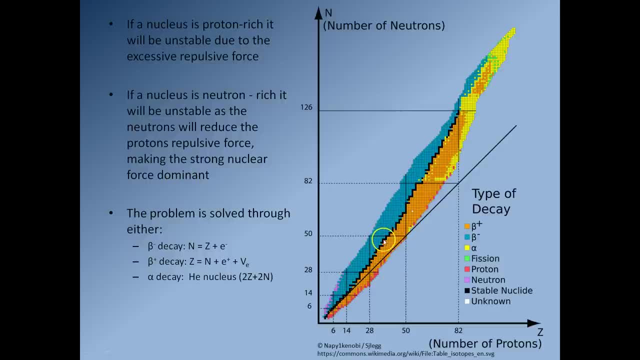 Okay, so that's, if you have too many neutrons, if you have too many protons, on the other hand, you can decay by either electron capture, so we take a proton and we change it into a neutron, or it can decay by alpha decay, which is up here. okay, so those are your possible options. so in that case, 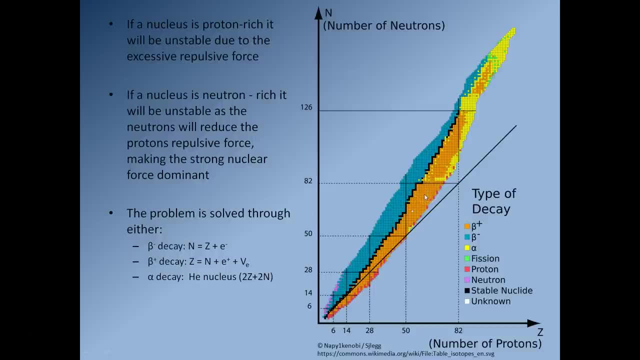 it's getting rid of excess protons in order to try and reduce the repulsive force. So by getting rid of protons, either changing them into neutrons or simply just kicking them out of the the nucleus altogether, you manage to bring stability by reducing the repulsive force. 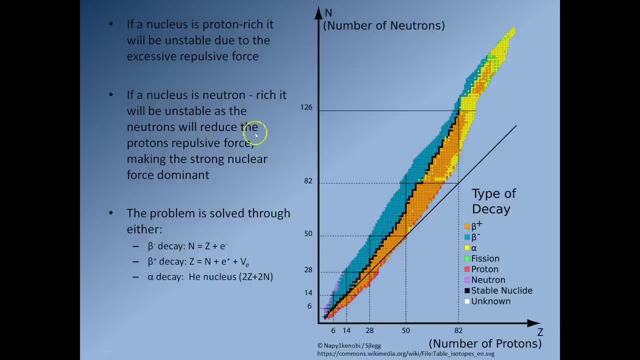 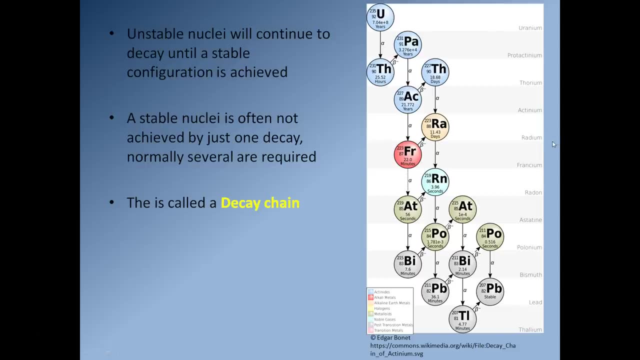 to the point where it's balanced with the strong nuclear force, at which point your, your nucleus, achieves balance and it will become stable. So unstable nuclei will continue to decay until they achieve a stable configuration. The vast majority of cases, nuclei have to decay more than once to actually reach a stable. 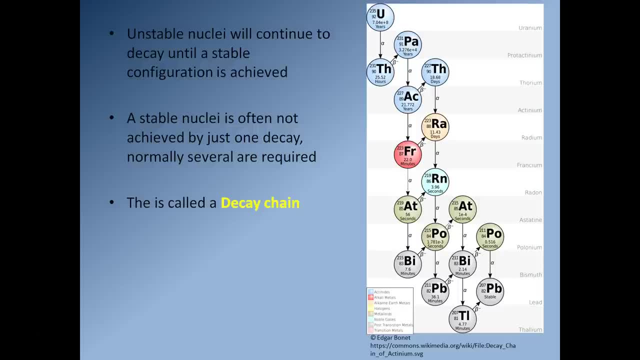 a stable configuration. There are very, very few nuclei that decay just once and then they instantly turn into a stable isotope. Most of them will have to go through several intermediate stages before they achieve a stable configuration. So here we go. so this is uranium-235 up here. so that's a radioactive isotope, uranium-235, you might know. 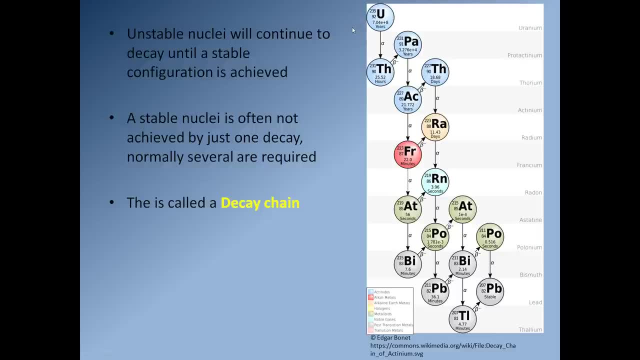 because it's the stuff that's used in nuclear weapons and in nuclear reactors. So uranium-235 will decay to give us lead-207, and lead-207 is stable, so it won't decay any further once it reaches lead-207.. But in order to get from the uranium-235 to lead-207 it has to go. 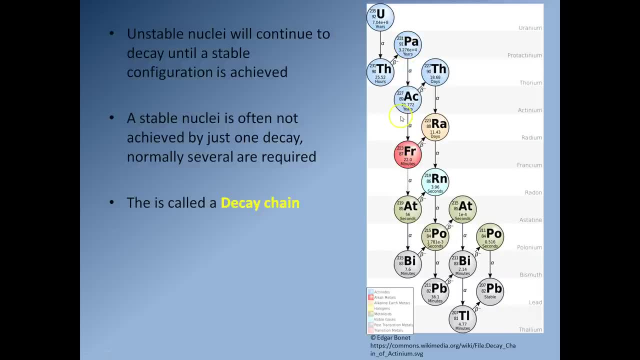 through all of these intermediate steps and you can see the intermediate steps are marked out as either alpha decay, which is in the form of the, the alpha symbol there, or beta negative decay, which is essentially beta decay. okay, So, in order to get from the uranium-235 to lead-207, 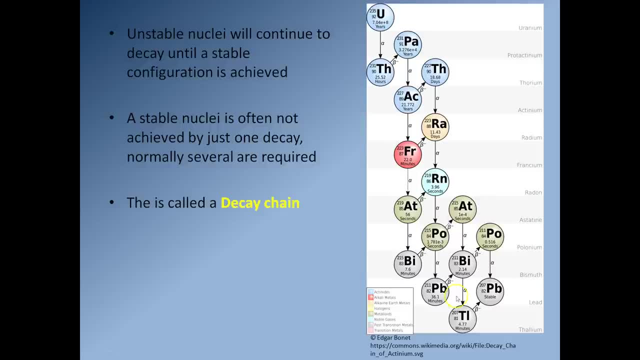 it's essentially kicking out protons and neutrons during alpha decay and it's changing neutrons into protons during beta decay. okay, So it has to go through all the intermediate steps. So these all these intermediate steps to get from the unstable isotope to the stable isotope. 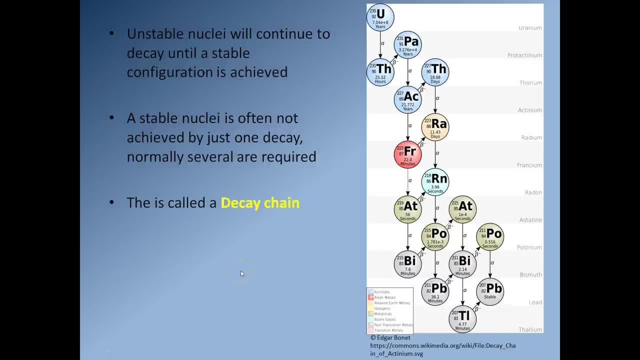 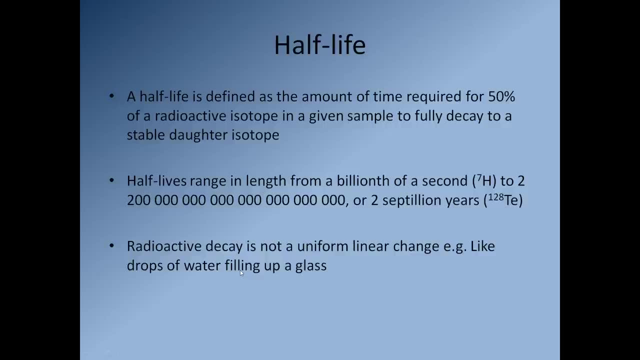 is referred to as the decay chain. So this then brings us on to halftraces. So a half-life is defined as the amount of time required for 50% of a radioactive isotope in a given sample to fully decay to a stable daughter isotope. 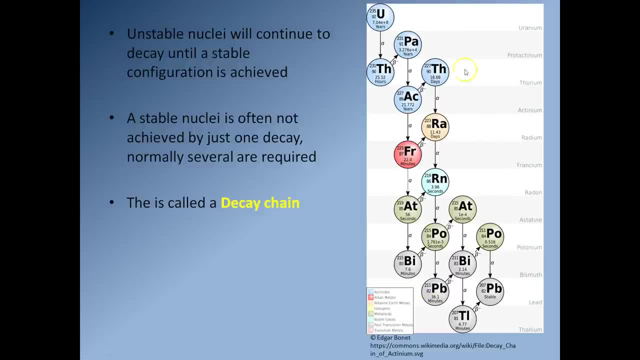 Okay. so we're not talking about the intermediate steps, okay, we're talking about how long does it take for 50% of this to decay to this? okay, We ignore all this stuff in between. So half-lives are defined as the amount of time required for 50% of a radioactive isotope in a given sample. 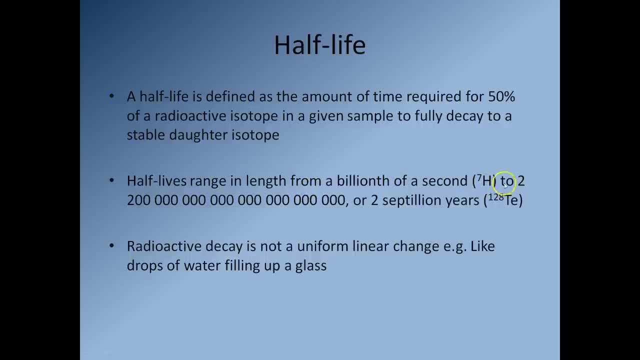 lives range in length from billionths of a second- so hydrogen 7 has a half life of a billionth of a second- to uh tellurium to 128. that has a half life of somewhere in the region of this number, which is two septillion years. so path lives vary quite significantly. so radioactive decay is also. 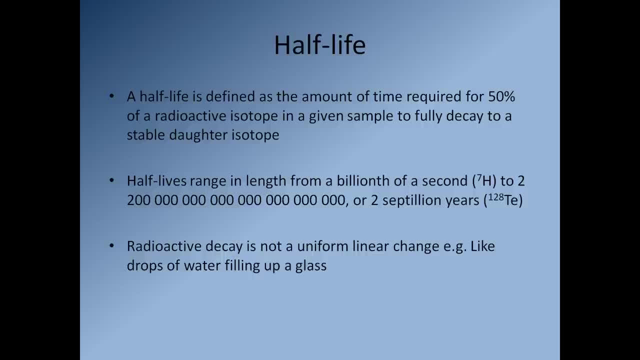 not a uniform linear change. so a uniform linear change is, like you know, drops of water falling into a glass. every drop of water increases the level in the glass by a set amount each time, in the case of half lives. you'll note, you'll see in the second, the graph that we have is not a nice. 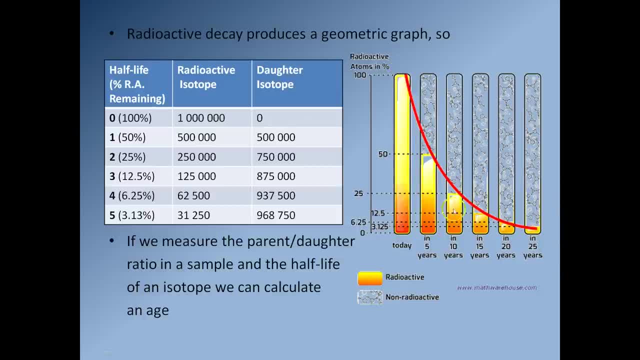 straight line. it's a curve, so it's not linear. so radioactive decay produces what we refer to as this geometric graph instead. so how's it working? so when we start off at you know the start time, obviously we have 100 parent isotopes and there's been no radioactive decay at that point, so we 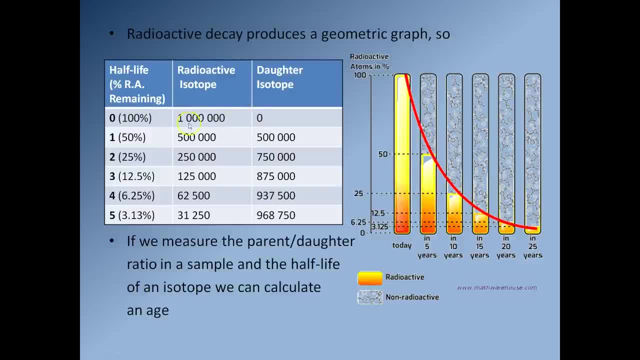 have a half life of a billionth of a second. so we have a half life of a billionth of a second. we have zero daughter isotopes. so in this model we're starting off with one million parent isotopes and at this point we have no daughter isotopes because nothing's decayed yet. 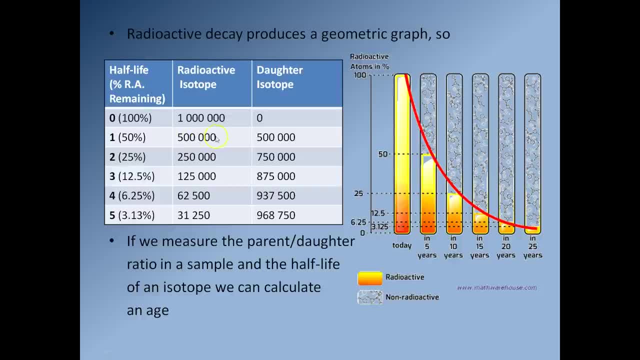 so after one half life, 50 percent of the parent isotopes have broken, broken down to give us daughter isotopes. so after one half life, we have 500,000 parent isotopes left and we now have 500,000 daughter isotopes. because these 500,000 parent isotopes 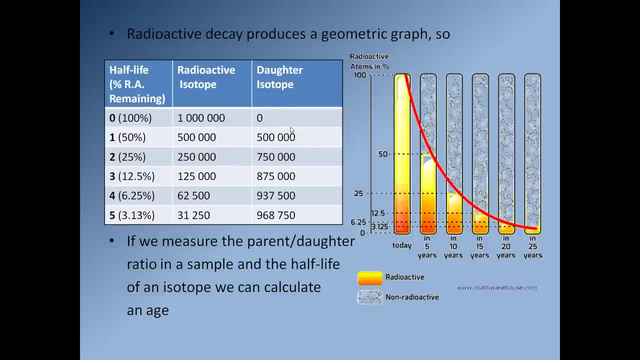 that are missing over here have changed into daughter isotopes. so after two half lives this number here is now divided by two, so we now have 250 parent isotopes left. i do apologize, that's 250,000 parent isotopes left and the 250,000 parent isotopes that 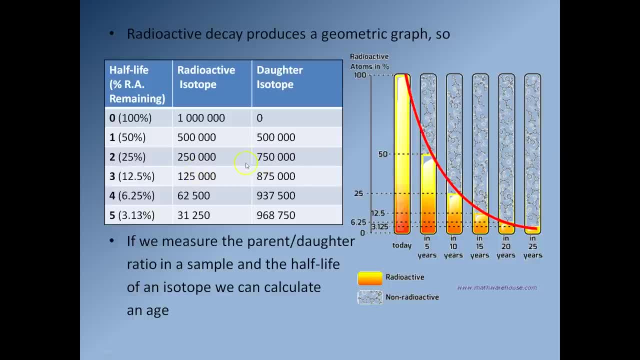 now disappeared, have now turned into daughter isotopes. so the amount of parent isotopes is now down at two hundred fifty thousand, but the amount of daughter isotopes is now increased to 750,000, and as we go down each half life you'll notice that this number here. 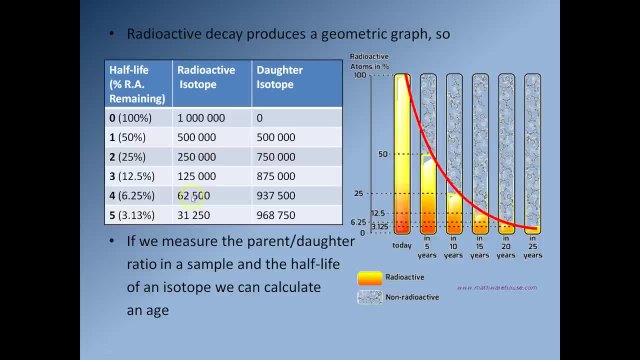 essentially, this number here is half this number. this number here is half of this number and this number here is half of this number. so every half life the amount of the parent isotope decreases by half. now what you'll notice is that when you add together the amount of parent isotope, 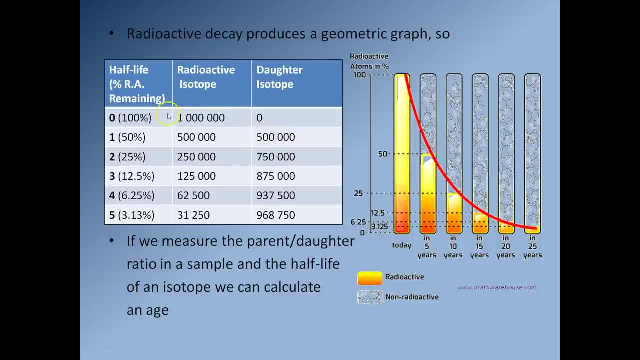 and the amount of daughter isotope, it equals the starting number of isotopes. so we started off with one million isotopes and when we add together the parent and daughter isotope for each half life, you'll notice it still equals one million. so all we're doing is we're changing parent isotopes. 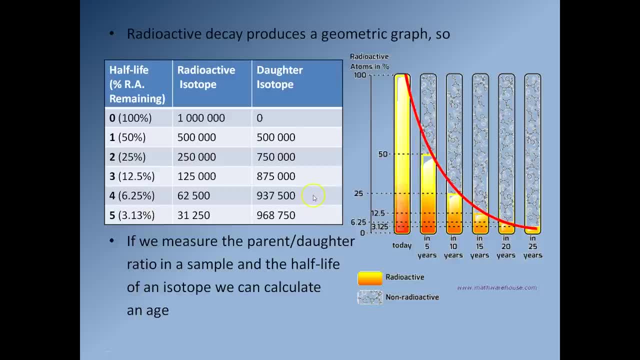 into daughter isotopes, we're not actually losing anything. so the total amount of isotopes is a constant. so that means that if we want to work out the amount of parent isotopes- let's say here four half lives- all we have to do is we have to take the total number of isotopes we started with. 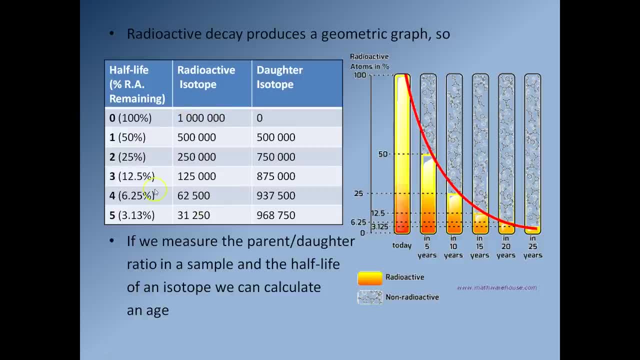 which was a million subtract 62,500, and therefore whatever number we end up with must be the amount of daughter isotopes. it's a relatively simple calculation, and so this means that when we look at this here and we transfer it onto a graph like this, as we go down each half light, you see, we go 50. 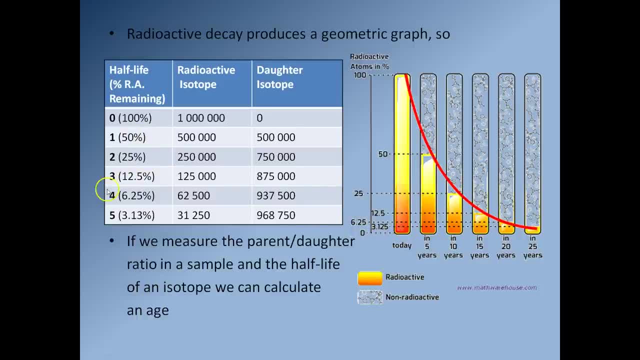 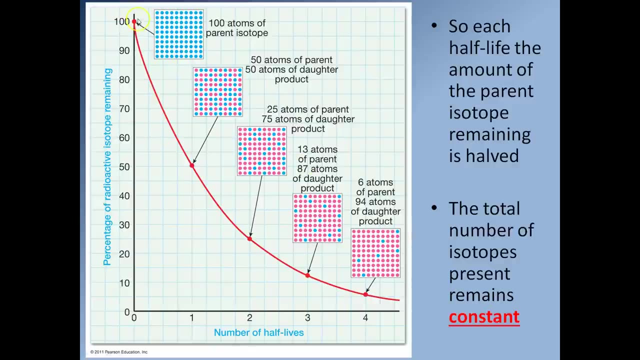 25, 12.5, 6.5, 25, 3.13- that's the amount of the parent isotope remaining as a percentage, and you'll see it gives us this curved graph rather than a straight line, and so this graph here shows you the same thing. here's this curved line. so each half life, 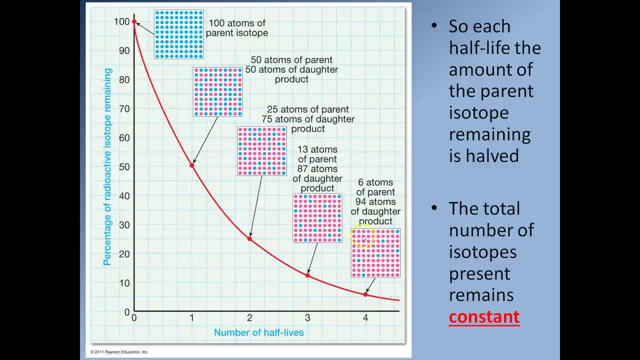 we can see the amount of the parent isotope is decreasing by half each time and you can see this in this case. it occurs in the form of these changes in the color dot. so the parent isotope is marked out in blue, the daughter isotope is marked out. 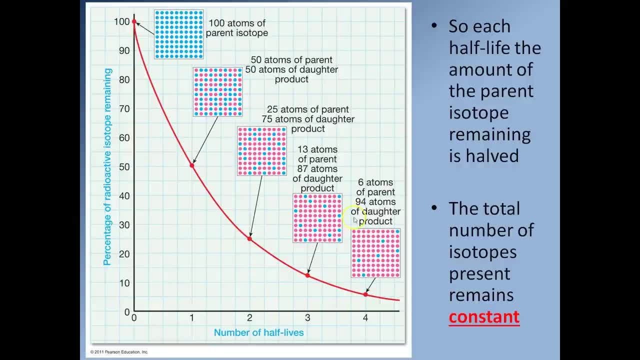 in pink and each time you'll see the amount of daughter isotope is increasing and the amount of parent isotope is decreasing. now the nice thing about this process is that it is constant. it happens at the same rate, so every second, let's say for argument's sake. 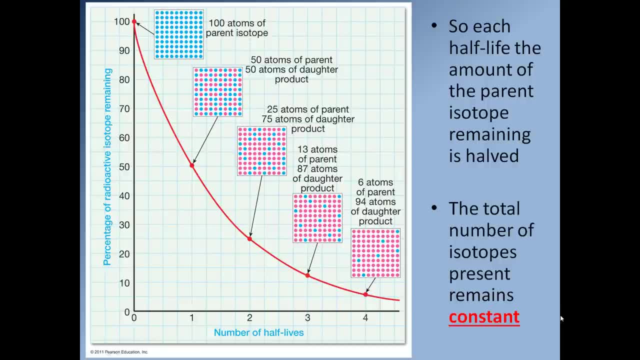 every second one isotope of the parent, i one isotope of the parent isotope decays the daughter isotope. so it's literally like a clock: it's going click, click, click, click, click. and so if we know the amount of the isotope that we started with, 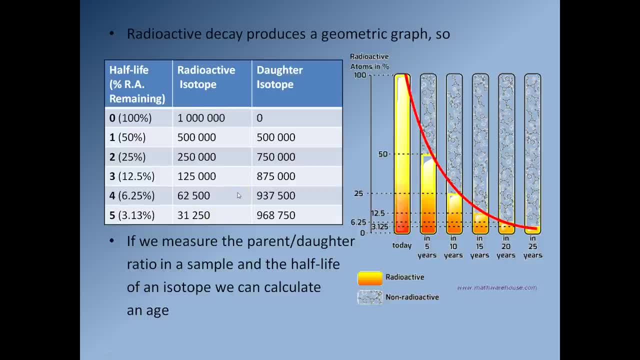 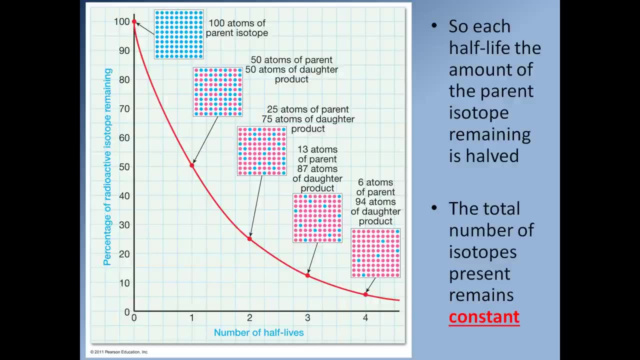 and we can measure the amount of parent and daughter isotope we have at any given time. well, all we it's very, very simple to calculate the age of a mineral, because the change is constant and we're going to, you know, as part of today's lab, we'll actually look at how you do that. 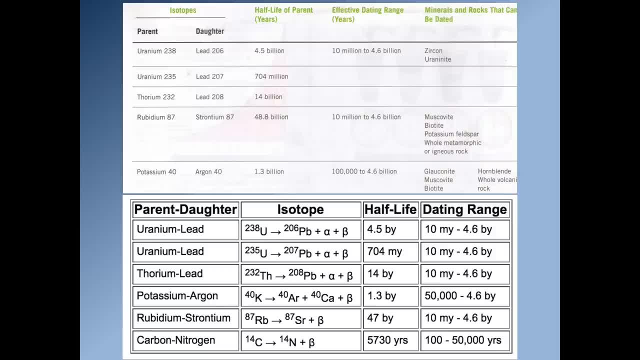 so, uh, it's been 20 minutes again, so this is a good time to stop for a second once again, pause the presentation, get up, have a walk around, have a drink of water, relax for a few minutes and then come back and we'll keep going, okay? so, uh, some of you might have heard Rupert snoring in the background. I do apologize for that. 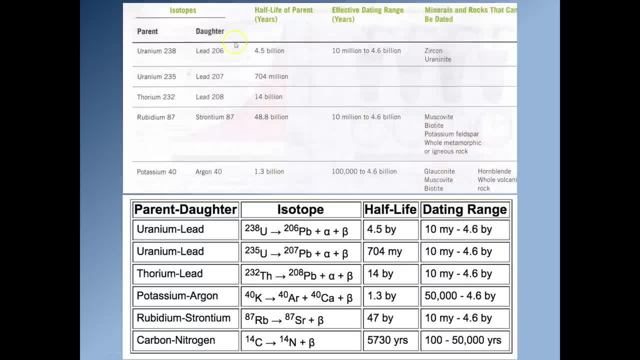 what can i say? my dog likes to snore, uh right. so these graphs here show you some of the classic uh parent daughter isotope relationships, and show you some of the half. So typically when we date minerals, we tend to use some of these relationships. 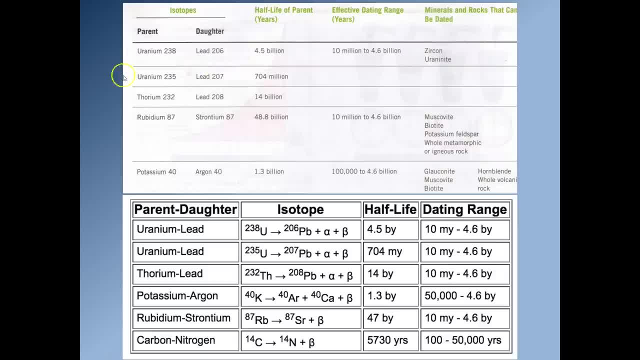 So uranium-238 decays to lead-206,. uranium-235 decays to lead-207,. thorium-232 decays to lead-208,. rubidium-87 decays to strontium-87,. potassium-40 decays to argon-40. 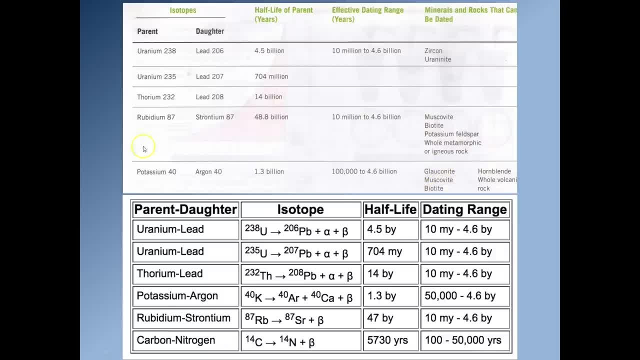 And over here you can see a list of minerals that we can use with these parent-daughter relationships to actually date the mineral, And here you can see the half-life. So in the case of uranium-238 and lead-206, we can use the mineral zircon or uranonite to date rocks. 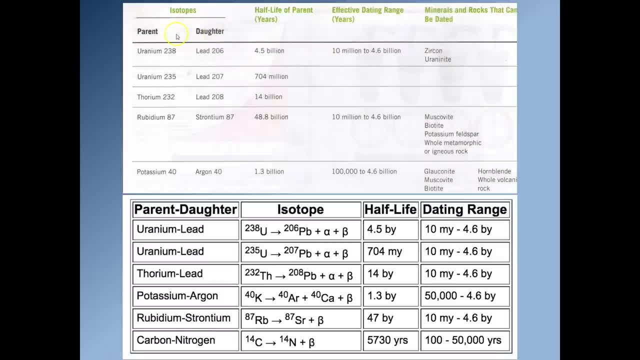 and it has a half-life of 4.5 billion years. So it means that only recently, in terms of geologic time, half of the uranium-238 the Earth originally started with has changed into lead-206, because the Earth is 4.56 billion years. So the Earth has just gone through its first half And it has a half-life with respect to uranium-238.. In the case of uranium-235,, it has a half-life of 704 million years. In the case of thorium-232,, it has a half-life of 14 billion years. 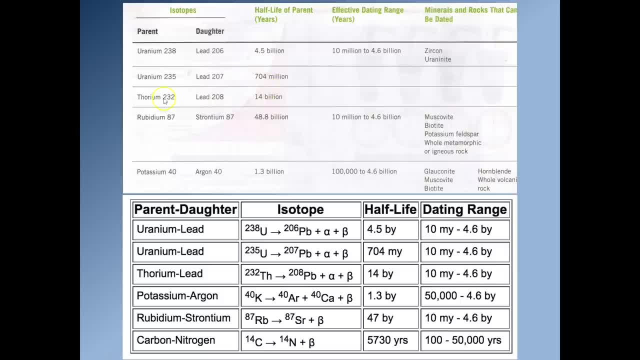 So the universe is about 13.8 billion years old. So we're just coming up on the first half-life for uranium-232.. In the case of rubidium-87 to strontium-87, the half-life is 48 billion years. 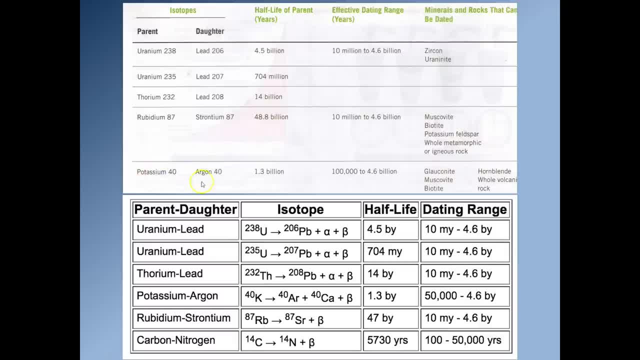 So we're nowhere near that half-life yet, And in the case of potassium-40 to argon-40, the half-life is around 1.3 billion years. So we can use these decays to essentially date rocks, because once again it happens at a constant rate, just like seconds ticking by. 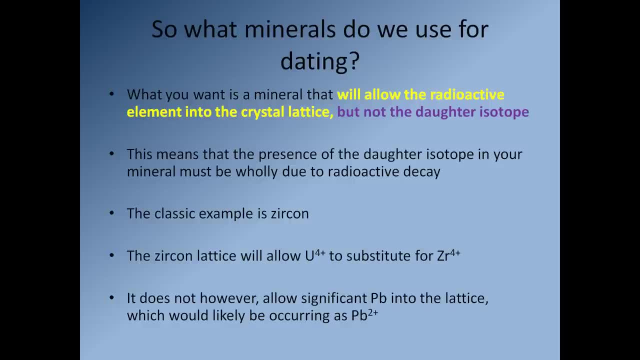 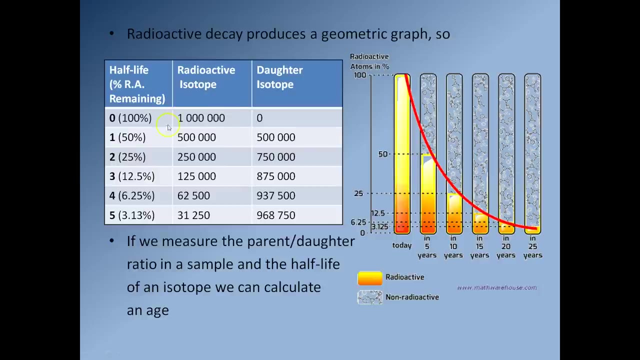 So the next question is: what minerals do we use for dating? So what we want is a mineral that will allow the radioactive element into the crystal, but not the dioxide. So what we want is a situation like this: We want a mineral that lets in the radioactive parent isotope but not the daughter isotope. 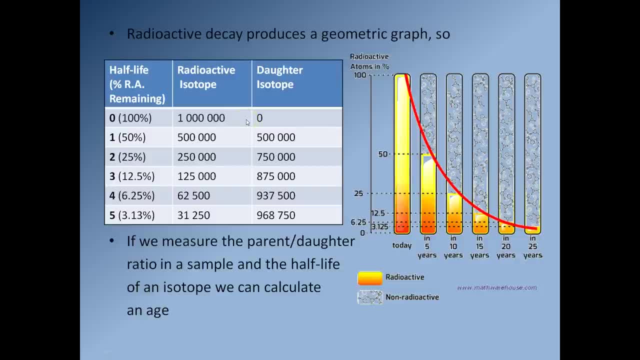 So that means when we come along later and we look at the mineral, if we find the daughter isotope in that mineral, it means that any daughter isotope that's in that crystal must have come from the decay of the parent isotope, because initially there was no daughter isotope. 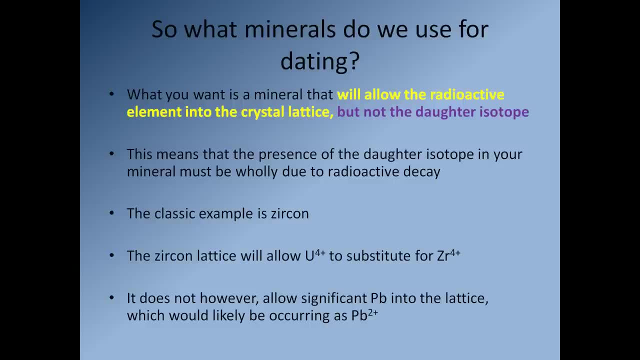 So what we want to do is we want to make sure that there's no daughter isotope in the crystal. So that's super important. So a classic example of this is the mineral zircon. So zircon is a zirconium silicate. 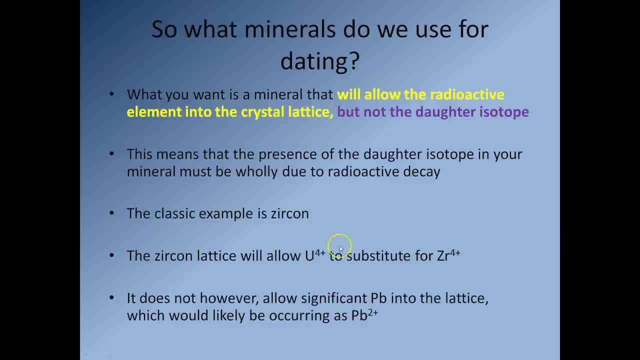 So what zircon will do is it will allow uranium into the crystal lattice, because uranium-4-plus can substitute for zirconium-4-plus. The two isotopes can substitute for one another quite easily in the crystal lattice, So zirconium-4-plus can substitute for zirconium-4-plus. 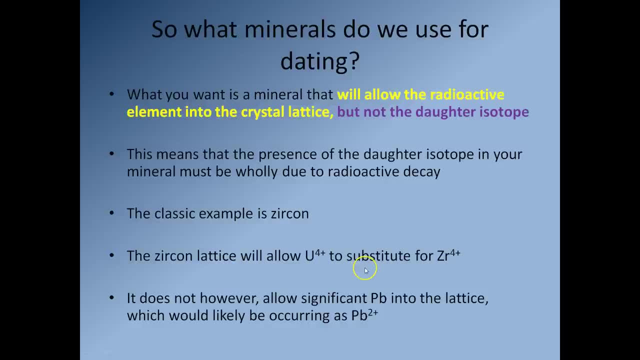 They can exchange quite happily. So this means that when crystals of zircon grow, as they grow, they will incorporate some crystals, some atoms of uranium, into the crystal lattice. However, zircon will not allow lead into the crystal lattice as the crystal grows. 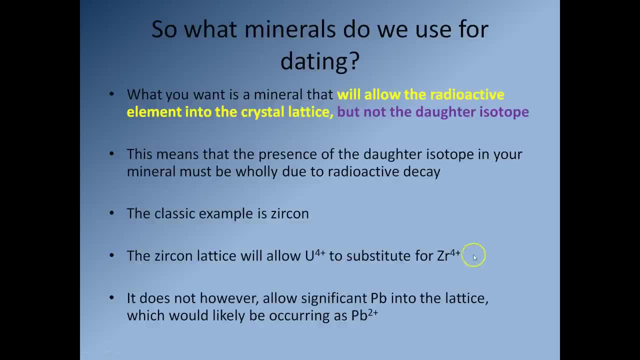 So this means that as your crystal of zircon is growing, it's going to contain lots of zirconium, a little bit of uranium, but absolutely zero lead. So that means when we come along in a billion years and we date that crystal, 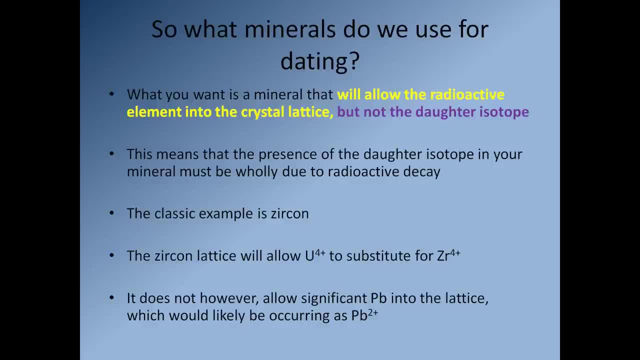 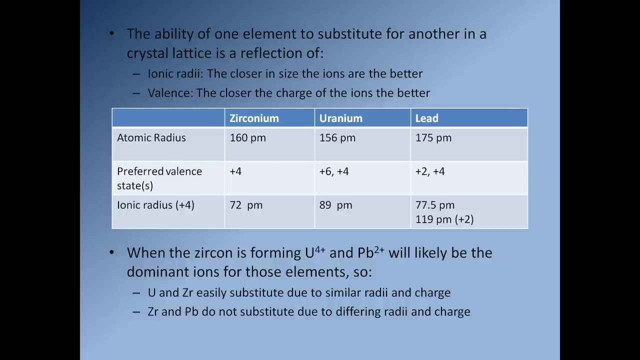 that means any lead that's in that crystal must have come from the decay of the parent isotope, Because when the crystal was newly formed it had no lead in it. So the ability of one element to substitute for another element in the crystal lattice. 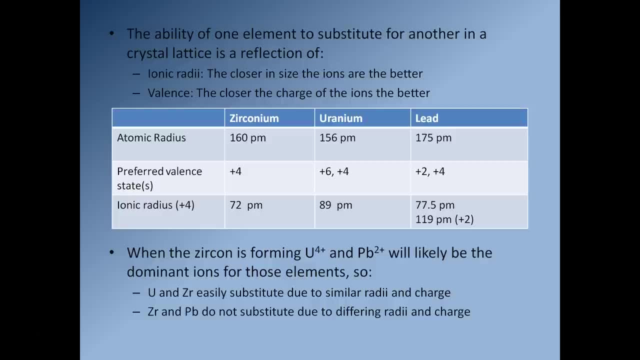 is a reflection of two things. The first one is the ionic radii. How big is the ion? So obviously, for two elements to substitute for each other, it's easier if the elements are the same size. If you're trying to substitute one element for a much larger element, 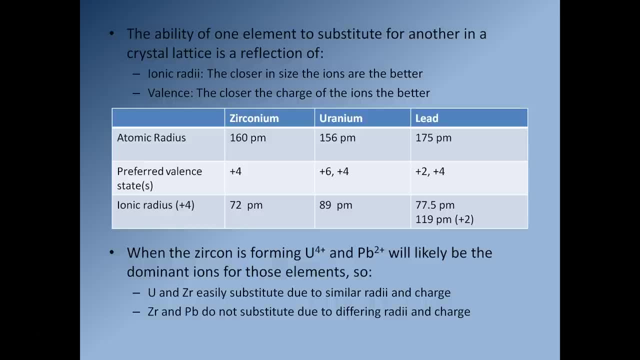 that's going to be a lot more difficult because you'll have to start rejigging the crystal lattice to make room for the new, larger element. The size of the isotope is all important. The other thing is the valence: How strongly positively or negatively charged is the ion? 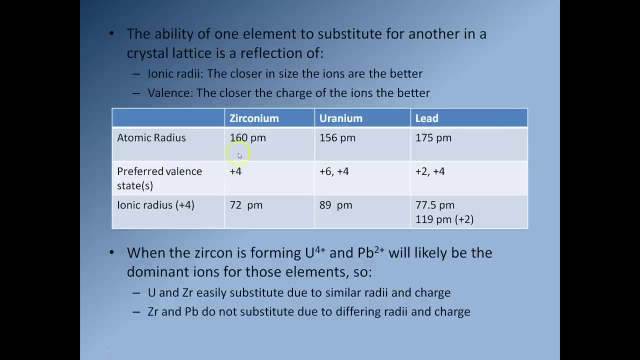 So if you're trying to substitute an ion like zirconium 4+ that has a 4 plus positive charge, well, obviously the easiest thing to substitute it for would be uranium 4+, because it has the same charge, a plus 4 charge. 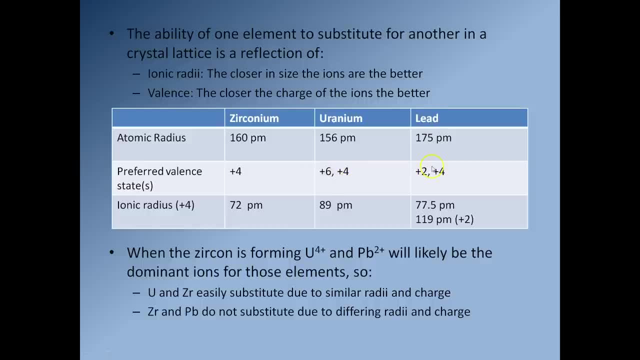 In contrast, if you're trying to substitute lead in, lead prefers to have a 2 plus charge, So it only has 2 positive charges, versus uranium and zircon, which typically have 4 positive charges, And so that means once again. 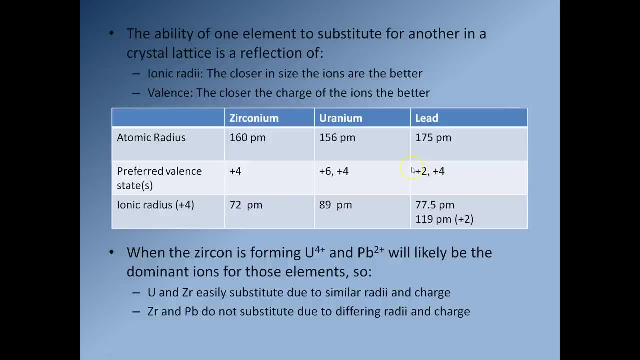 it's more difficult to squeeze the lead in because it has a different charge. So, in the case of zirconium, here's the valence state for zircon and here's the ionic radius. This is the important measurement here. 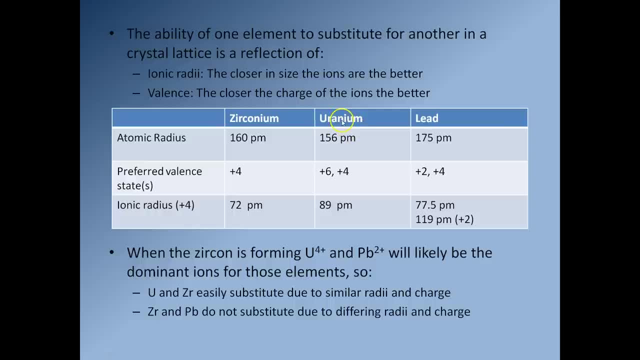 So it's 72 picometers. In the case of uranium, the preferred valence state is 4+, so that's a like-for-like substitution, so that's good. And the ionic radius is 89 picometers, so relatively close in terms of size. 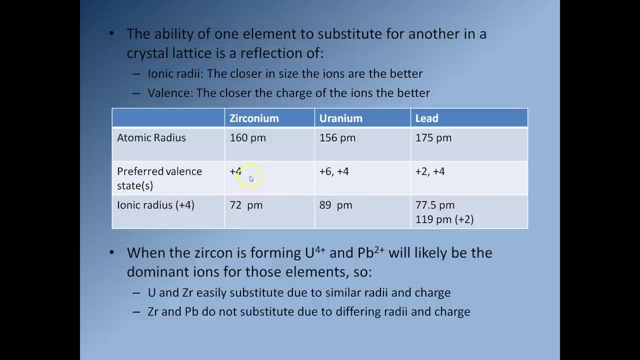 so they can substitute for one another relatively easily. Same valence, similar size. That's why uranium can substitute for zircon in the crystal lattice of- sorry, let's try that again. That's why uranium can substitute for zirconium in the crystal lattice of zircon. 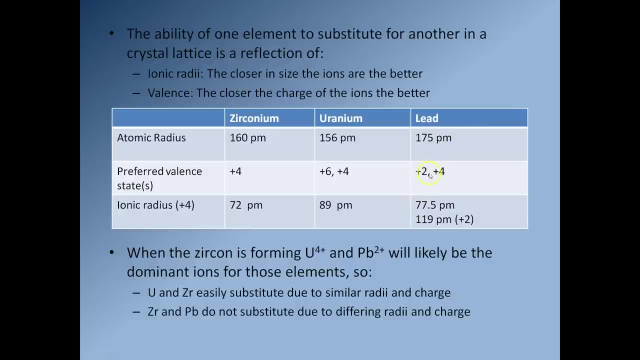 Now let's look at lead. Lead prefers to form ions that have a valence state of 2.. So, as you can see, 2 plus versus 4 plus, we have a different valence state. So that's going to be a strike against lead straight away. 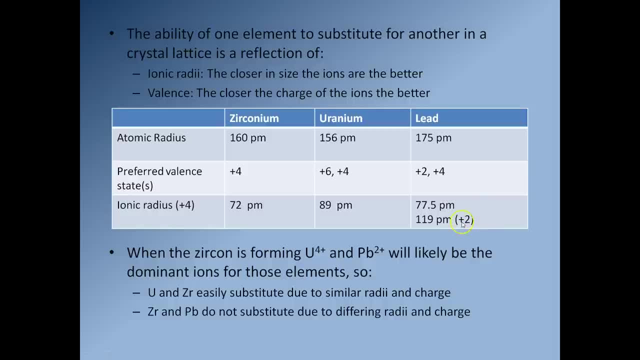 And the other thing is the 2 plus ion of lead has an atomic radius of 119 picometers, That is considerably larger than the ion of zirconium, And so that makes it really really difficult for lead to squeeze into the crystal lattice. 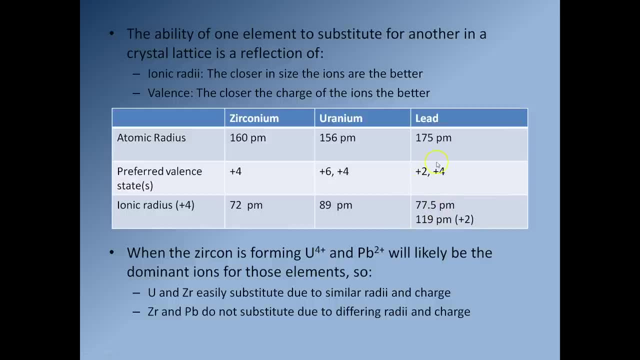 because it's very, very big and it has a lower charge, And so that makes it very, very difficult. And so lead will not go into the crystal lattice because it cannot easily substitute for zirconium. Uranium can substitute for zirconium. 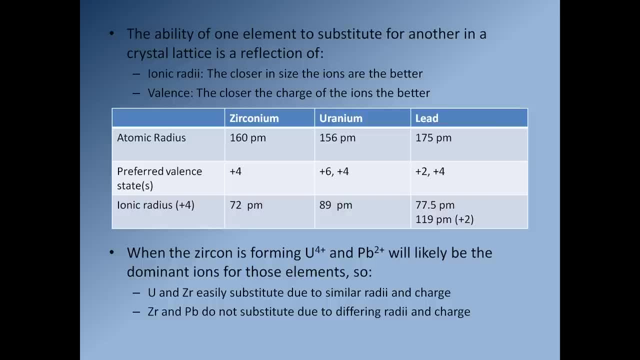 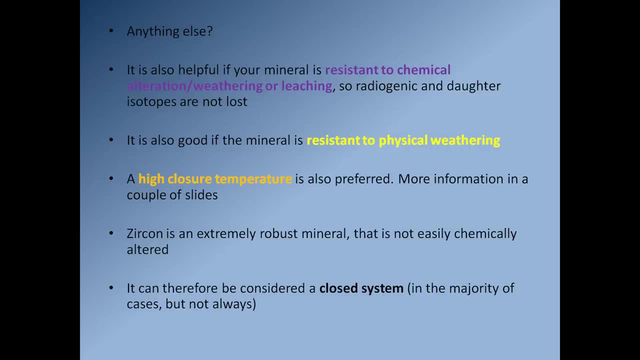 so, as the zircon crystal grows, some zircon will substitute for uranium in the crystal lattice. So is there anything else that's helpful when we're looking for minerals to date? Well, yes, The next thing is we would like our mineral to be resistant. 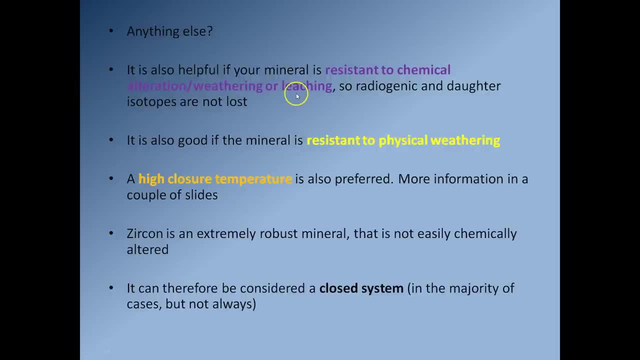 to chemical alteration, weathering or leaching. So what we really want is we want a crystal, a mineral that's going to be very, very physically robust, so it will persist for a long time. It won't break down. 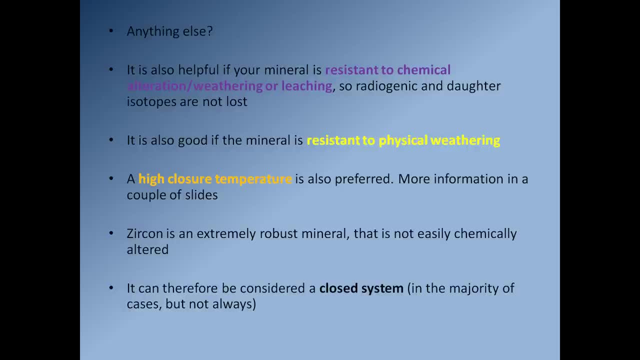 And we want our mineral to be chemically robust. because that means if it's not chemically robust, the mineral will alter to a new mineral and when it does that, it might lose parent or daughter isotopes. or it means that even if the mineral doesn't change, 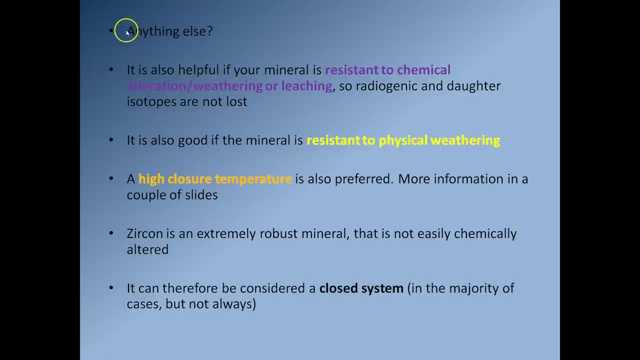 if it's not chemically robust, it might lose parent or daughter isotopes through the process of leaching, So radioactive isotopes have to be chemically and physically resistant to change. We also want a mineral that has a high closure temperature, So I'm going to give you more information about that. 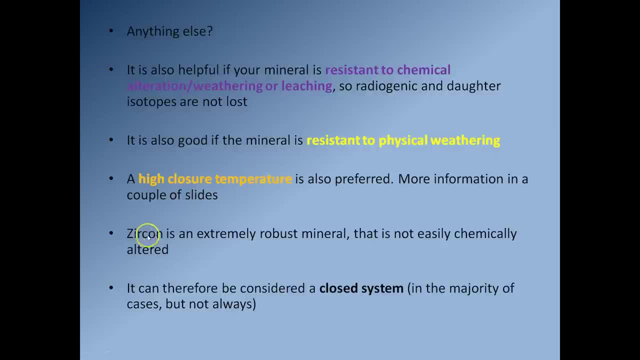 in a couple of slides' time. So that's why zircon is so good. zircon is an extremely robust mineral. it's chemically inert and it's also very physically strong. It's very resistant to erosion. The nice thing about zircon is that you can therefore. 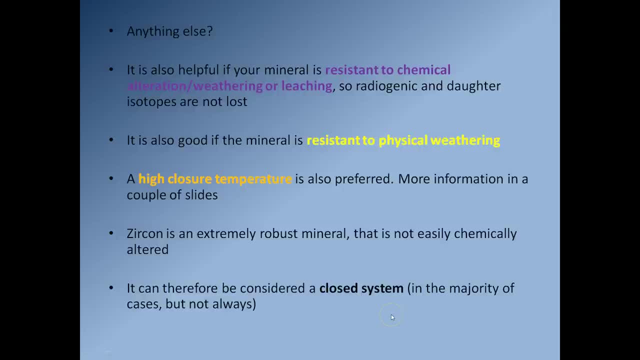 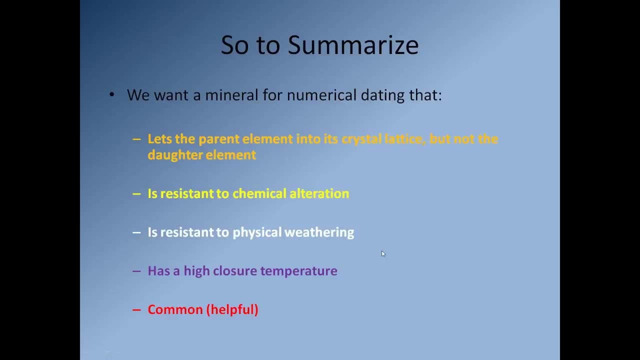 consider it a closed system in the majority of cases. So it means nothing has come in, nothing has been lost once the zircon crystal formed. So to summarise, what we want is we want a mineral when we're doing numerical dating. 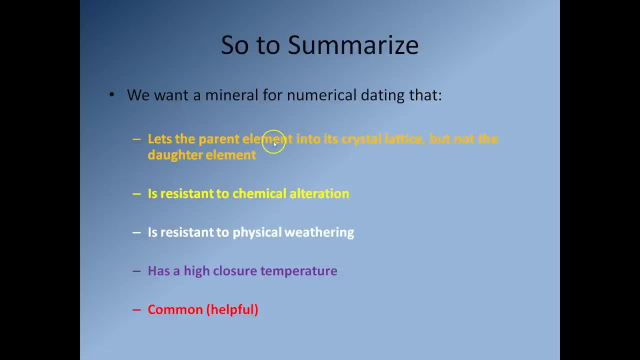 that lets in the parent isotope but not the daughter isotope. We want a mineral that's resistant to chemical alteration. We want a mineral that's resistant to physical weathering. We want a mineral that has a high closure temperature, And it's also really helpful if the mineral is common. 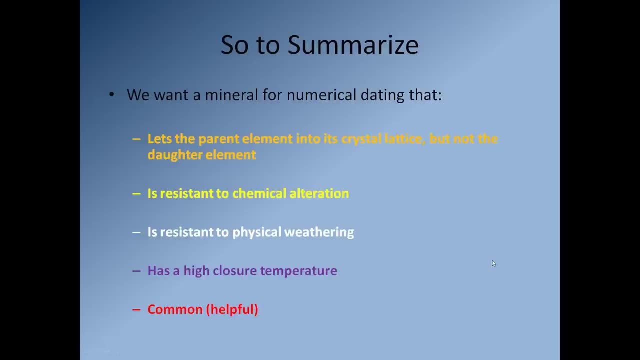 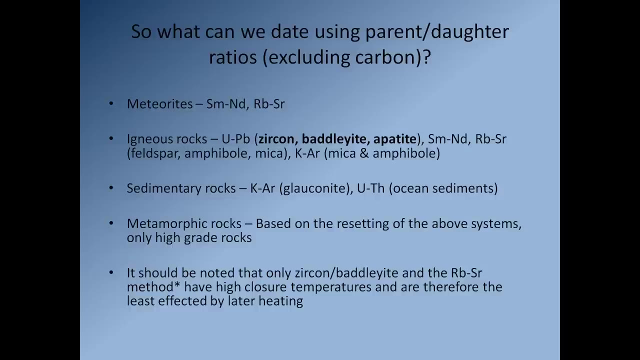 The more common it is, the easier it is to find and therefore the cheaper the dating will be. So the next question is: well, what can we actually date using parent-daughter isotopes? So just to be clear, I'm never going to ask you about this. 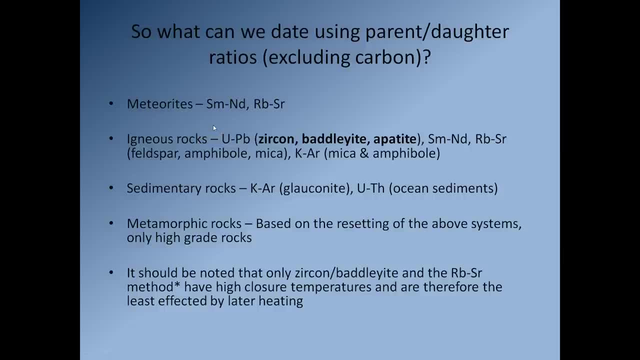 so we're just going to zip through this slide relatively quickly. So when we date things like meteorites, we tend to use isotopes that have quite a long half-life. We tend to use things like samarium, neodymium or rubidium strontium. 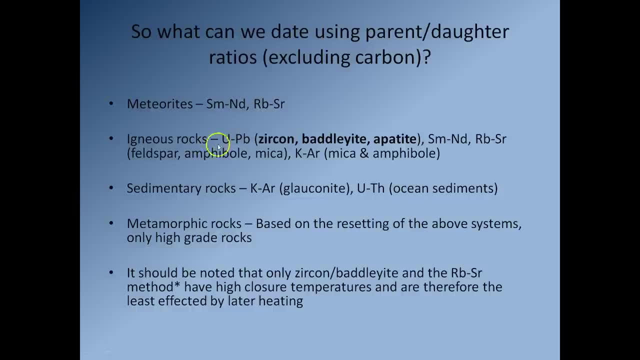 Igneous rocks. we tend to really love to use uranium lead dating, and we tend to use minerals like zircon, badellite or apatite for that. We can also use other methods like samarium, neodymium, rubidium, strontium or potassium argon. 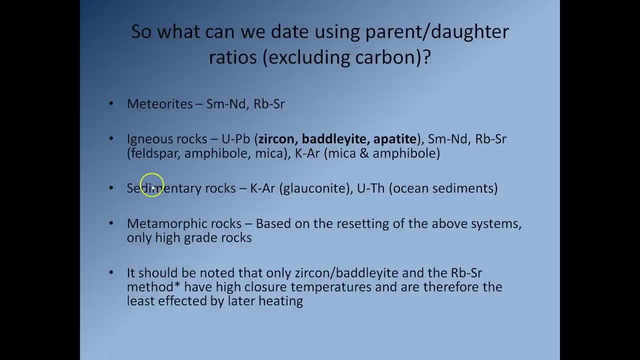 if the situation requires it, I'm going to skip sedimentary rocks for a second: Metamorphic rocks. well, metamorphic rocks. we actually date based on what we refer to as the resetting of the crystals, and that's due to leakage. 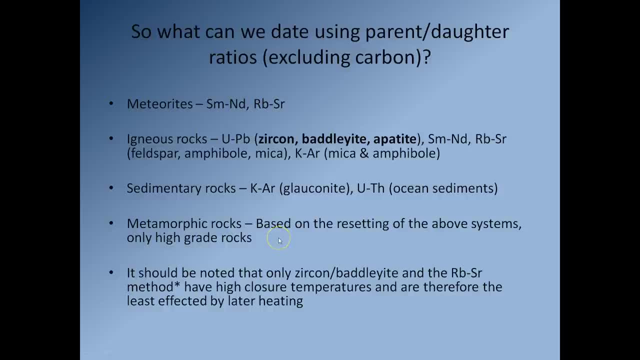 So when we take the mineral back up above its closure temperature, it can lose parent or daughter isotopes and that will actually affect the date which we get from the crystal. And so when we you know, we can actually date when that leakage occurs. 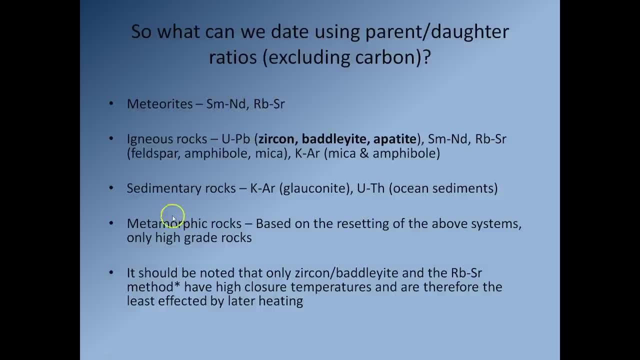 and that's how we date metamorphic rocks. Now, in the case of sedimentary rocks, we can use potassium argon dating for a mineral called glauconite, and we can use uranium thorium dating for certain types of ocean sediments. 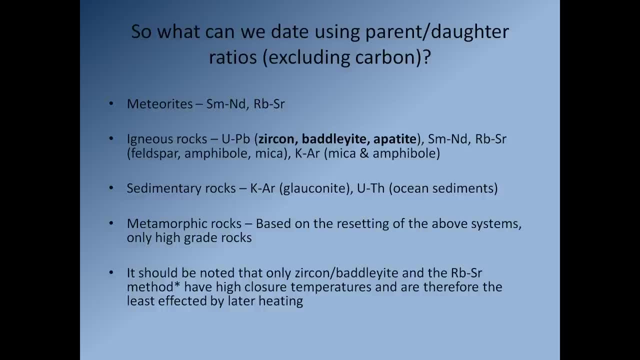 However, I need to make this very, very clear: You can't really date sedimentary rocks using numerical dating. It's extremely difficult and extremely inaccurate. The main problem is this: When you're dealing with classic sedimentary rocks like a sandstone, 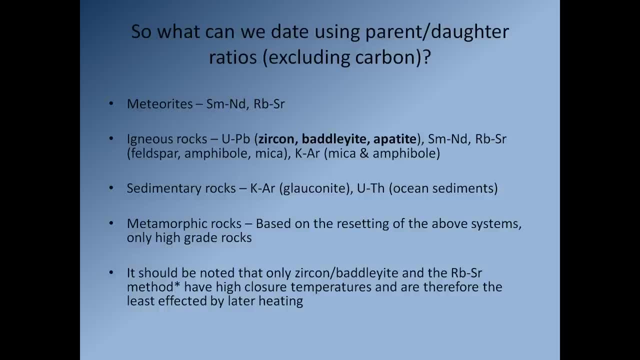 well, sandstones are made up of lots of crystals. yeah, The crystals that make up a sandstone were not made when the sandstone was forming. The crystals that make up a sandstone were formed when, let's say, the rock that was weathered to make that sediment formed. 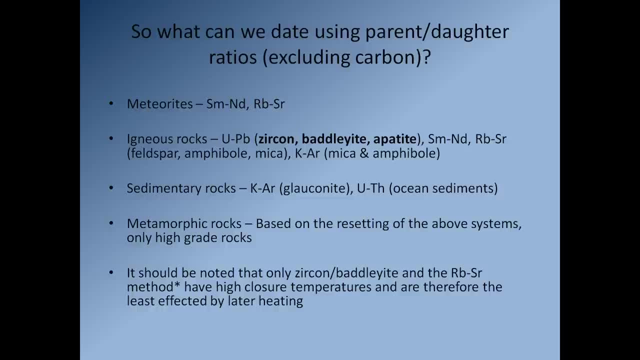 So your sandstone might be made up of crystals of quartz that were formed when a granite cooled 1.5 billion years ago. Your sandstone might only have been deposited, let's say, 100 million years ago, But when you date your sandstone, 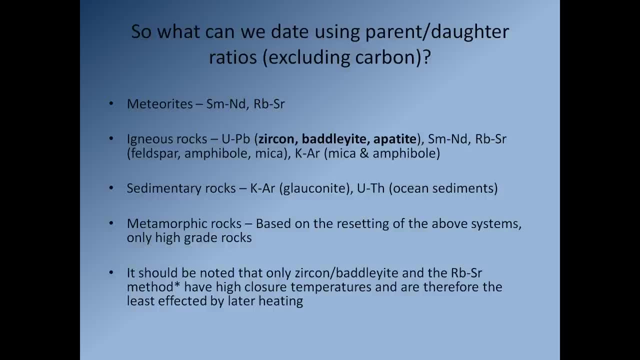 it's going to contain crystals from the granite in it, and so when you date the sandstone, it's going to give you an age of 1.5 billion years, even though the sandstone didn't form until you know. let's say: 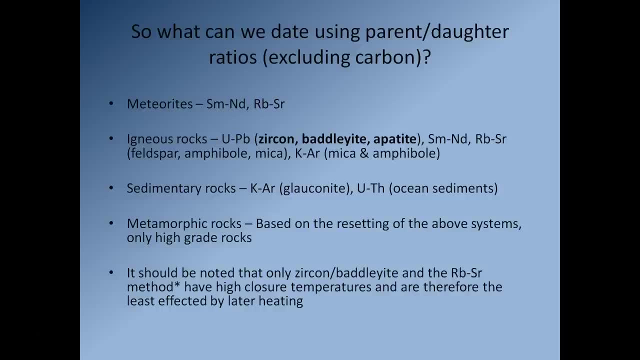 100 million years ago. So classic sedimentary rocks are notoriously difficult to date because the crystals, the clasts within them are not actually from the sedimentary rock itself. They're formed somewhere else, as another rock forms, and they're transported in. 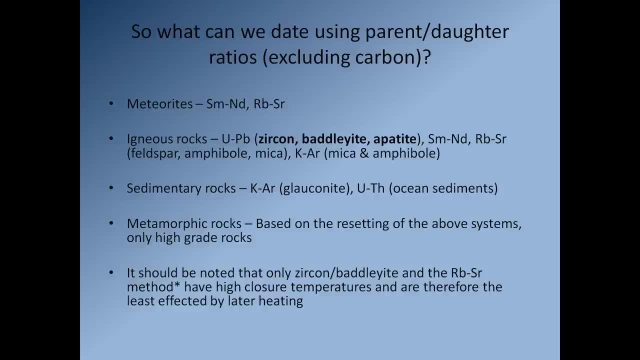 So when you date a classic sedimentary rock like a sandstone, you're actually dating the parent rock from which the sediment formed. So it should also be noted that only zircon and badellite- badellite is zirconium oxide- and rubidium strontium have high closure temperatures. 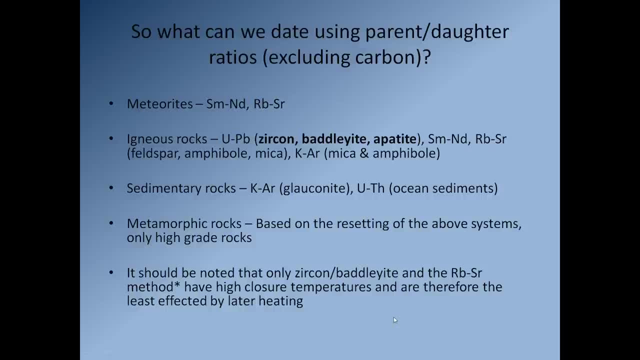 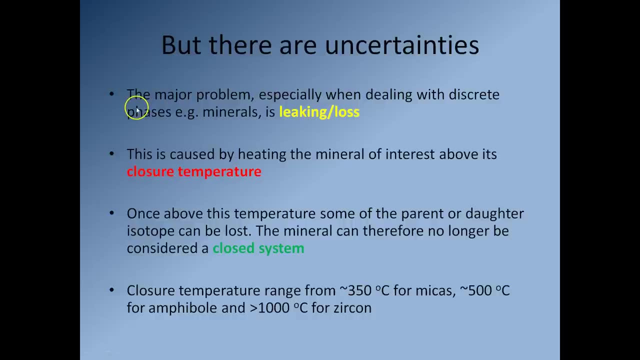 and therefore they're less affected by later heating. So our one problem is: what happens if we take our mineral back up above its closure temperature? Well, the main problem with radioactive dating is what we refer to as leakage or loss, And this is caused when you take a mineral up above its closure temperature. 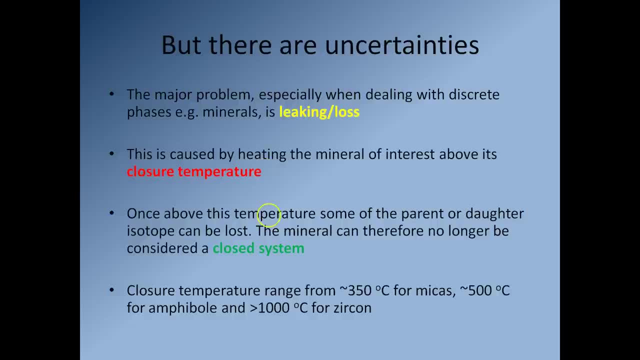 So when you take a mineral back above its closure temperature, it means you can lose parent or daughter isotopes. So that means this ratio between parent and daughter isotopes has been building up over time as parent isotopes changing to daughter isotopes will be lost. 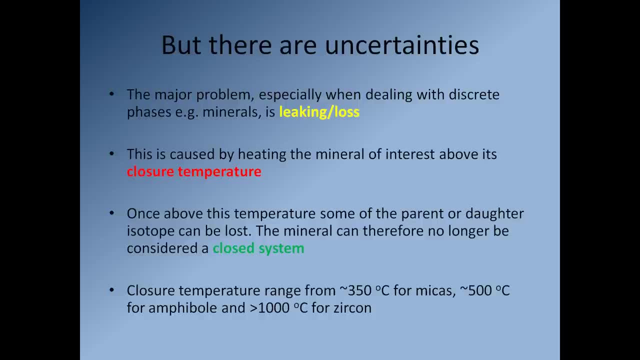 because we'll lose either parent or daughter isotopes. So when that happens, the crystal can no longer be considered a closed system, And so any data we get from it is going to be bad. So the closure range for minerals, so the closure range for the micas. 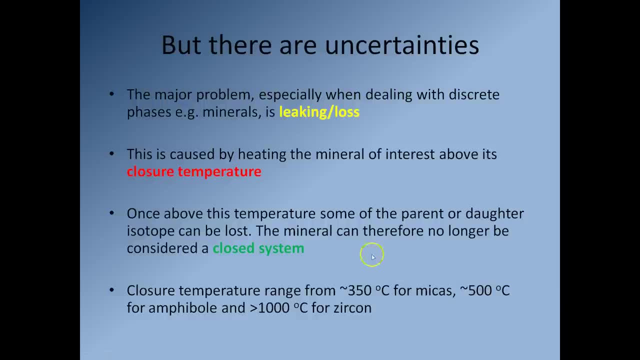 like biotite or muscovite, is in the range of about 350 Celsius. So if you take a crystal of biotite, if you take a crystal of biotite above 350 Celsius, then that means any potassium or argon that's formed in it. 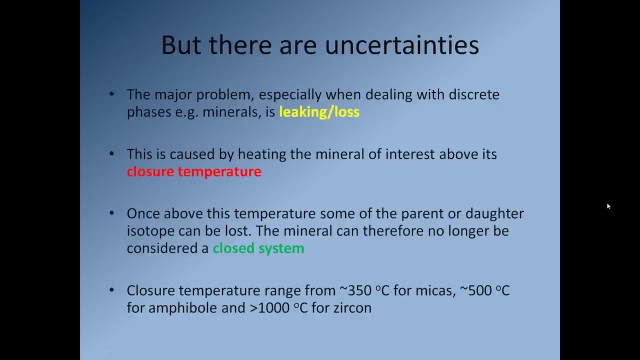 due to potassium-argon decay, some of it will be lost, and that means you can't use the crystal for dating. In the case of amphibole like hornblende, the closure temperature is about 500 Celsius, And I need to point out. 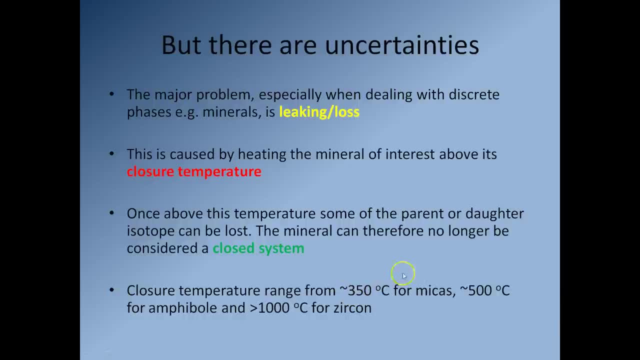 in terms of geology, taking a rock to 350 Celsius or 500 Celsius is pretty easy. It's not that difficult to do, And so that means minerals like micas and amphiboles are pretty bad for dating because it's so easy to essentially cause them to suffer leakage. 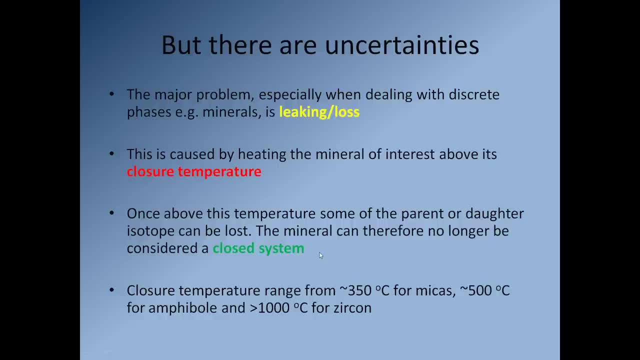 due to raising the temperature above their closure temperature. Now, in the case of zircon, the closure temperature is in excess of 1,000 Celsius. That's a pretty high temperature, and so it's pretty high to achieve that kind of temperature. 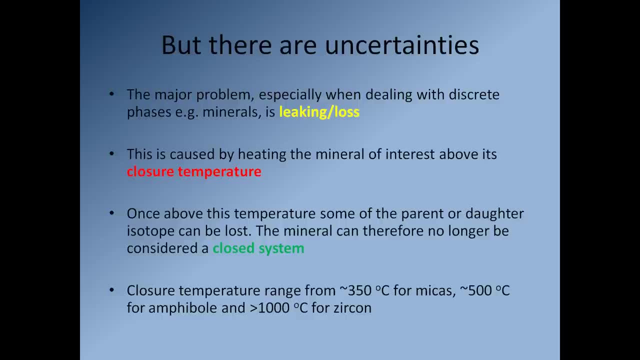 And so that means it's very, very hard to make a zircon crystal exceed its closure temperature, And so most zircon crystals will not have suffered leakage, And so the amount of parent and daughter isotopes you have in the crystal will represent what was there initially. 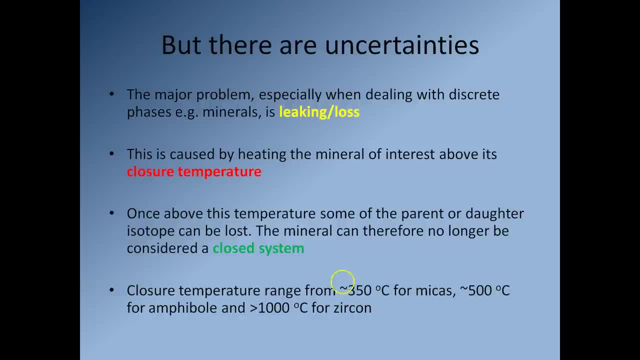 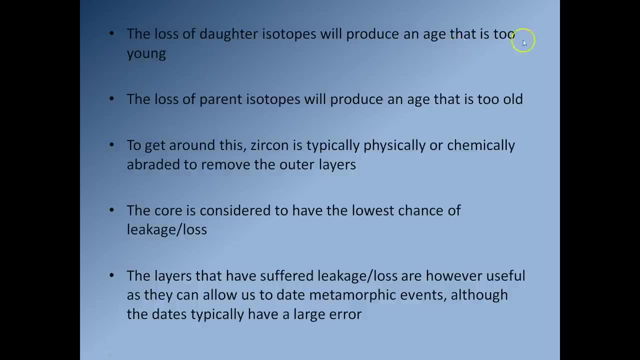 or should I say the amount of parent isotope that was there initially. So if we do suffer leakage and we lose daughter isotopes, that will produce an age that is too young. In contrast, if we lose parent isotopes, that will produce an age that is too old. 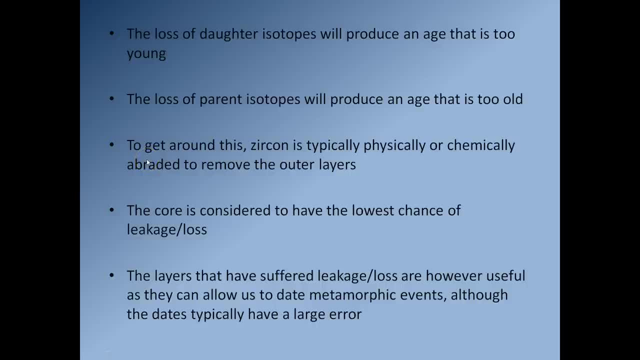 So, to get around this, what we typically do is, before we analyze a zircon crystal, we will either physically or chemically abrade the crystal to remove the outer layers. So if a zircon crystal, well, if there's the possibility that a zircon crystal, 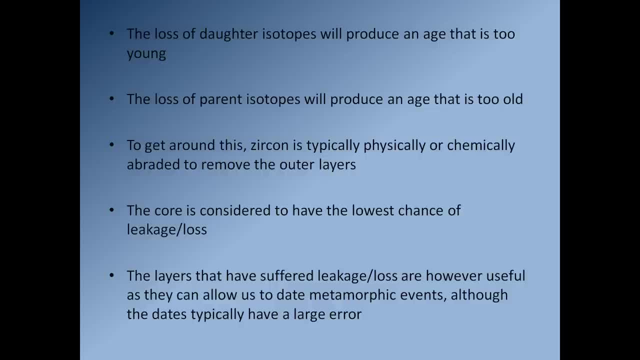 has suffered some leakage. what we'll do is we'll say: well, most of that leakage will have occurred along the outer edge of the crystal. So all we'll do is we'll just strip off the outer edge of the crystal and we'll keep the core of the crystal. 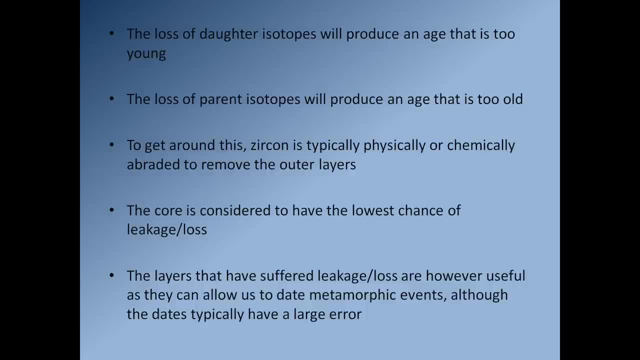 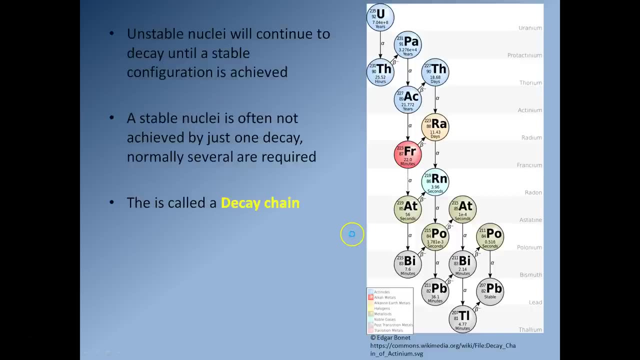 because that region is less likely to have suffered leakage. So by removing these outer layers, by abrading them away, we just retain the core. So I'm actually going to zip all the way back to this picture here. So here's our zircon crystal. 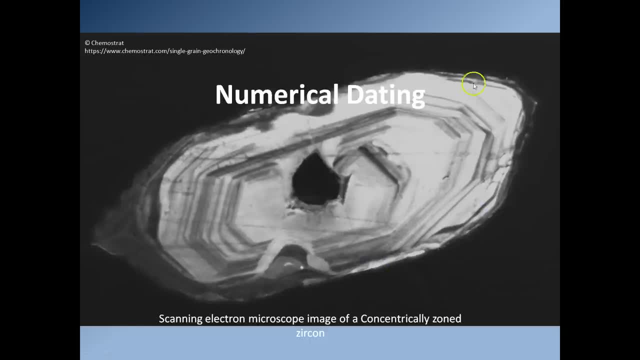 So if we were to date this zircon crystal, we would abrade it first and we would strip off these outer layers, because if there was any leakage, though, that would be the area that would be most likely to be affected. That would mean we'd be left. 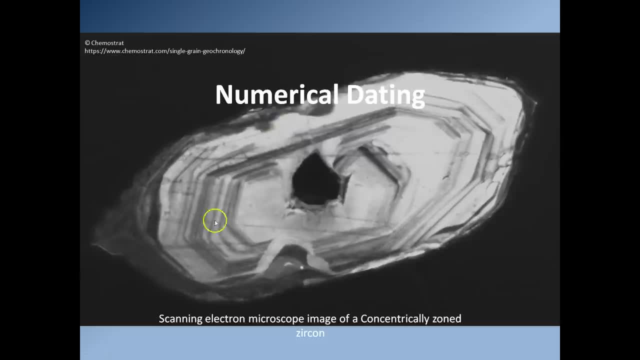 with just this core region here. That's the area that is least likely to have suffered loss or leakage, So it's going to give us the best data. And it's also the region that formed first, And so it's going to give us. 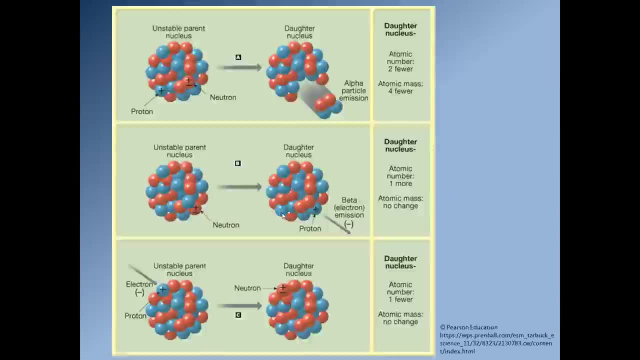 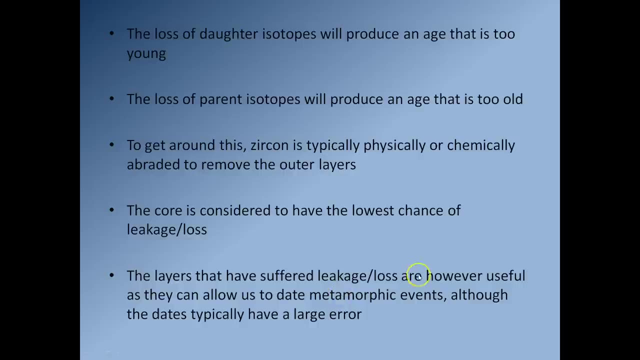 the maximum possible age for that crystal. So the layers that have suffered leakage or losses, depending on how you want to describe it, are, however, useful, as they can allow us to date metamorphic events, although the dates typically have a large error. So, by analysing these outer layers, 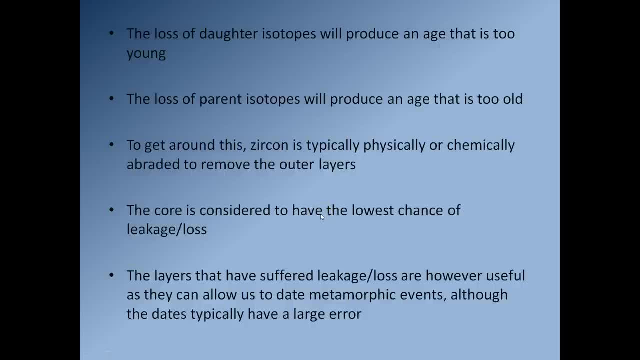 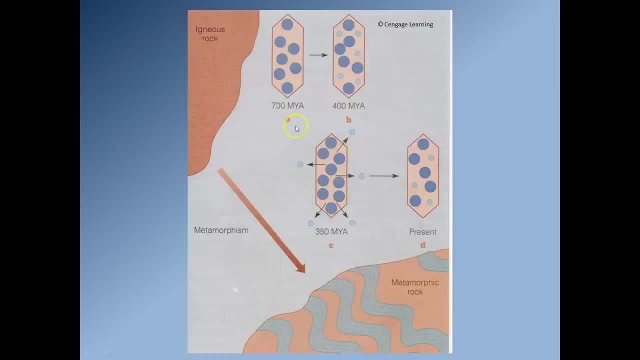 it can also help you work out some other things, but in most cases it's a hindrance. So this is our situation. So here's our crystal of our mineral. So 700 million years ago our crystal formed. let's just say for argument's sake, 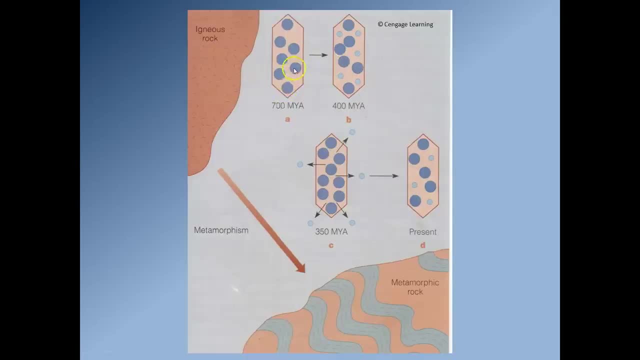 this is zircon And you can see that it contains the parent isotope. which are these large blue circles here? Obviously contains none: the daughter isotope. Now, after 300 million years, we can see that some of the parent isotope has decayed to the daughter isotope. 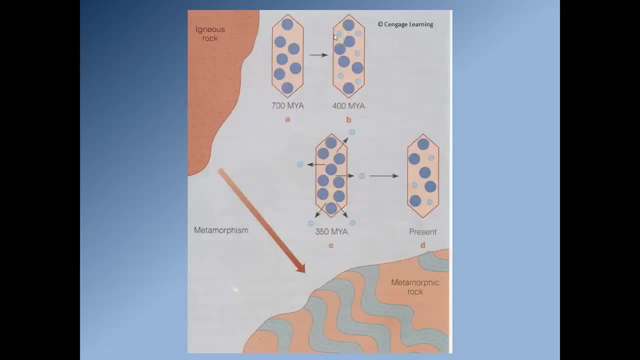 which is marked as these small blue circles here. So typically, if we were to analyse the crystal at this point, we would tell that this crystal here formed 300 million years ago, 700 million years here, 400 million years ago here. 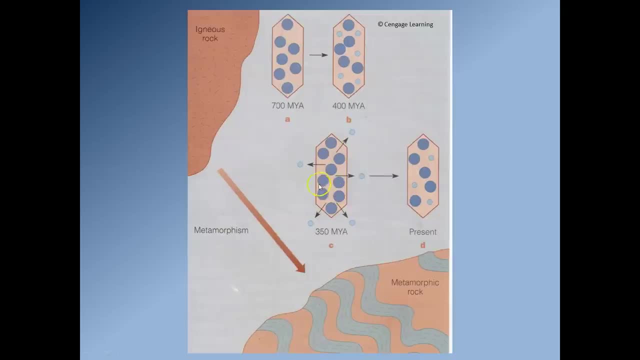 Now what's happened in this case is the zircon crystal has then been heated up to above its closure temperature, And, as it's exceeded its closure temperature, it's undergone the process of loss, And so it's released some of in this case. 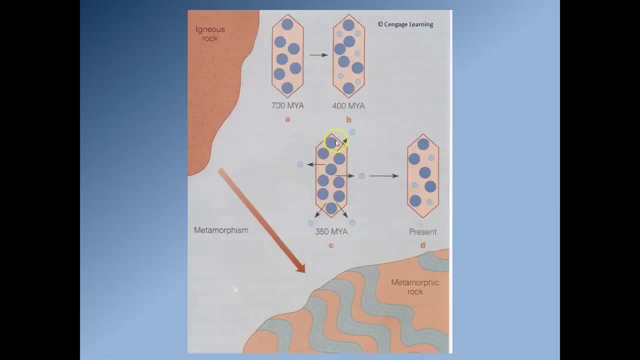 the daughter isotope into the surrounding environment, And so that's obviously affected the parent isotope to daughter isotope ratio, And so this means that any age we calculate from this crystal here is going to be incorrect, And so this means that you know. 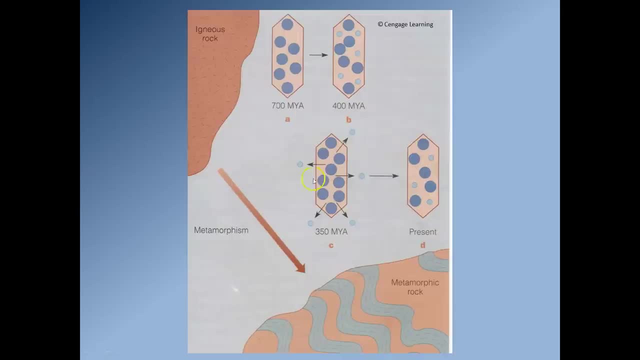 from 350 million years ago to the present day. essentially, it means that by the time we make it to the present day, we do not have the correct amount of daughter isotopes in the crystal because we've lost some to the surrounding environment. 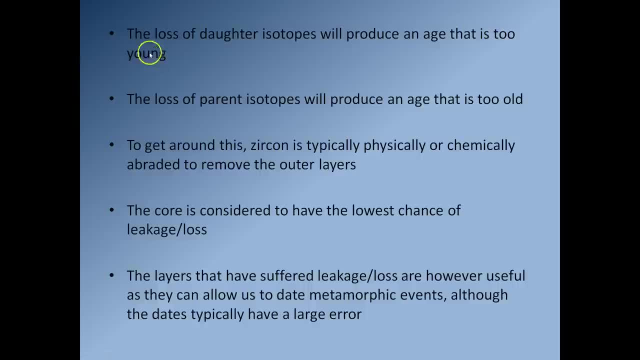 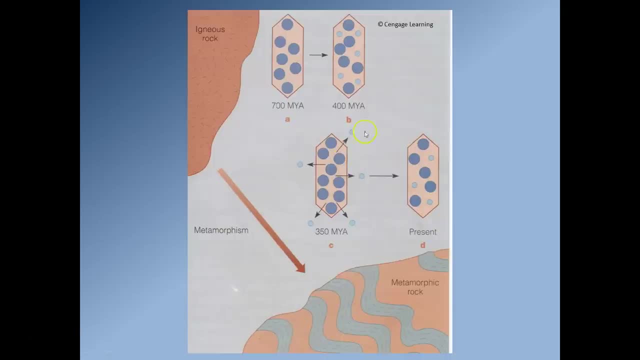 And so the loss of daughter isotopes will produce an age that is too young, And so if we were to date this crystal here, we would get an age that was too young because we have lost some of the daughter isotope. So that's the danger of leakage. 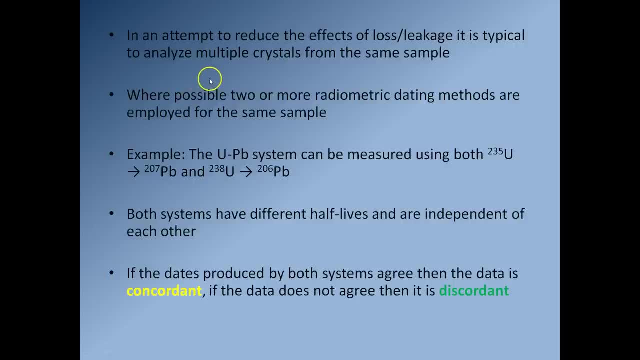 So, as I said, the other thing we can do is, in an attempt to reduce the effects of loss or leakage, we typically just don't analyse one crystal from the sample. We'll typically try and analyse as many crystals of zircon from the sample as we possibly can. 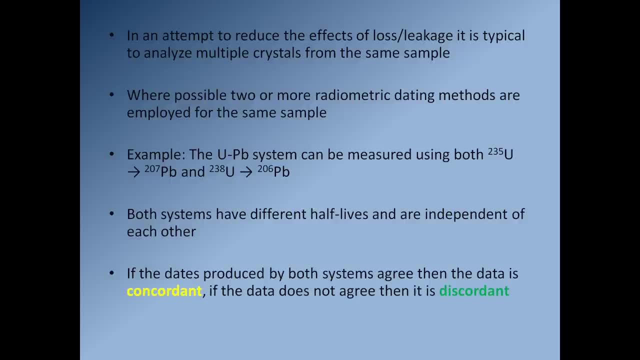 So the logic of that is, the more data you have, the easier it is to spot bad data. essentially, Another thing we can do is we can use two radiometric dating methods at the same time. So for zircon, it lets in uranium. 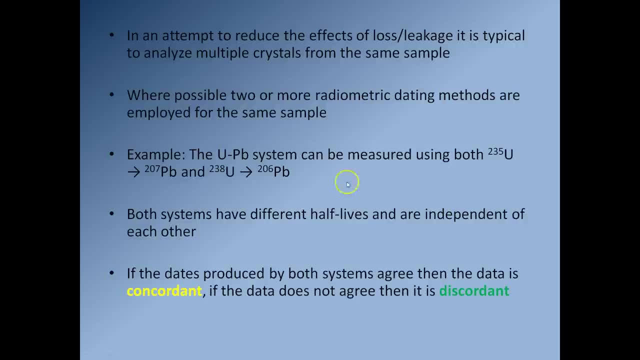 That means the zircon will let in uranium-235 and uranium-238.. Uranium-235 decays to lead-207 and uranium-238 decays to lead-206.. And so that means within one crystal of zircon we have two different dating methods. 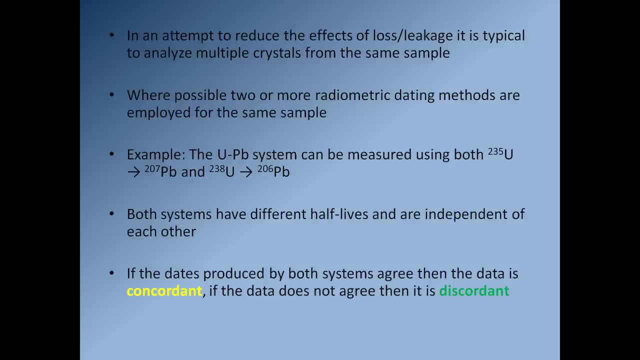 And so what we can do is we can analyse the crystal of zircon using these two different dating methods, and if the numbers match, then great, that means our data is good. If the numbers do not match, that means we have a problem. 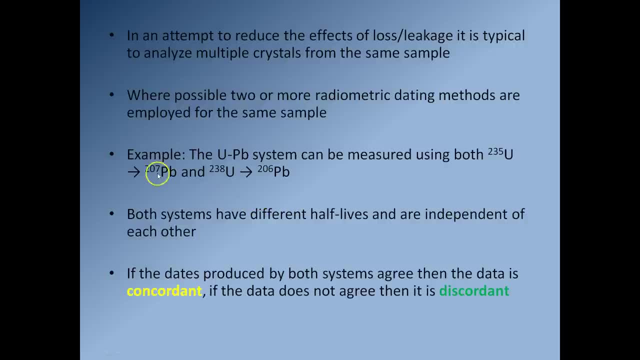 So both of these systems have different half-lives and they run independently of one another. That's why we can compare the data and look at whether it matches or doesn't match. So if the dates produced by this process agree, then the data is referred to as concordant. 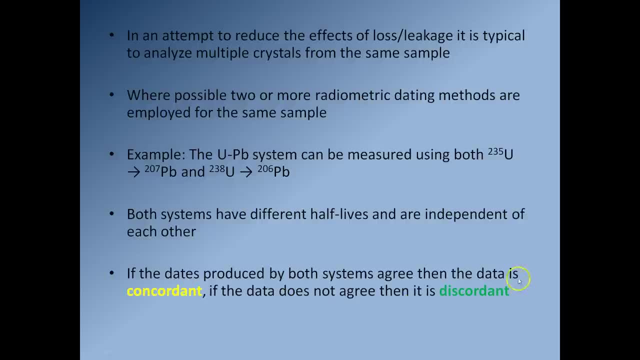 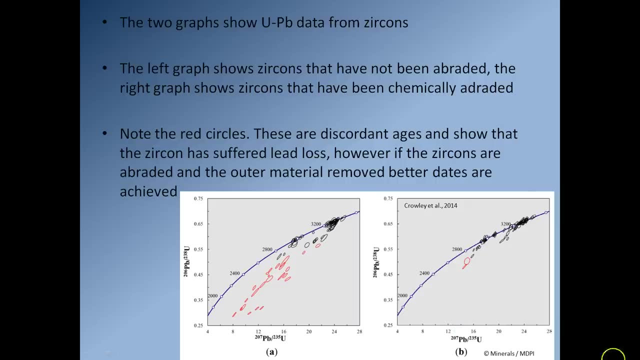 If the data does not agree, it's referred to as discordant, And discordant data is bad. So here we have two graphs for the analysis of crystals of zircon. So we have lead-207, so we have uranium-235 down here on the x-axis. 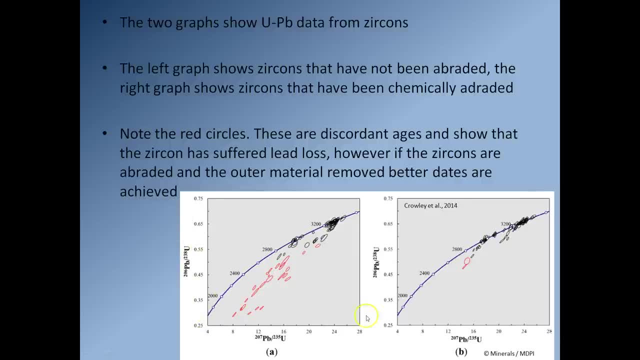 and we have uranium-238 up here on the y-axis And this line here is referred to as the line of concordia. It's marked out in blue And that's a line we just calculate in the lab. So when we look at these two graphs, 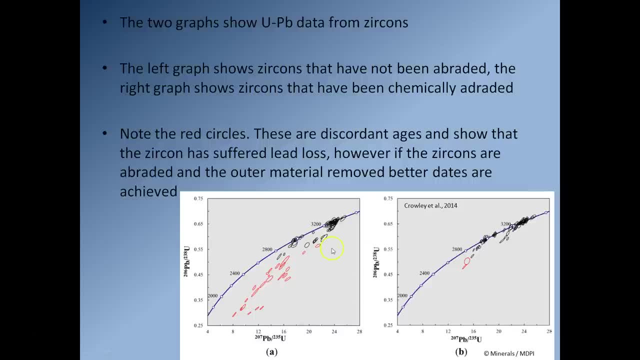 what do we see? Well, the good data, the concordant data, is marked out by these black circles. That's the data that falls on or very near the line of concordia. Now, all these red circles here, you can see, are a very, very long way. 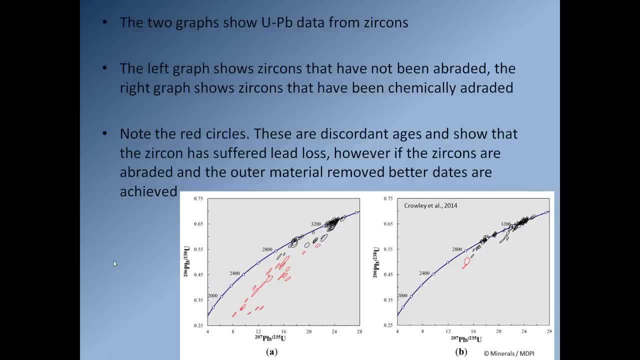 from the line of concordia, and so we know this is bad data. So what can we do? Well, if we abrade the zircons to get rid of the outer layers of the zircon, those are the layers that are most likely. 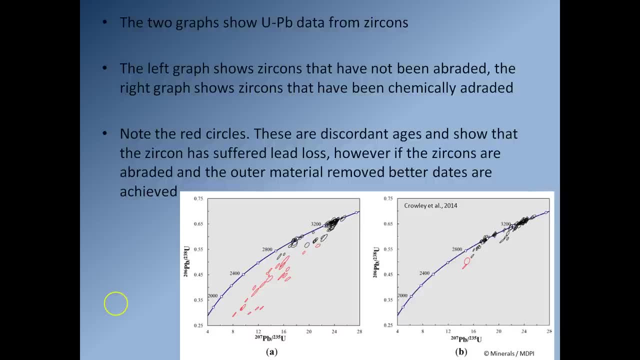 to have suffered loss due to leakage. If we get rid of them and then analyse crystals again, what do we see? So over here we have the same crystals being analysed, but in this case they've been abraded to get rid of the outer layers. 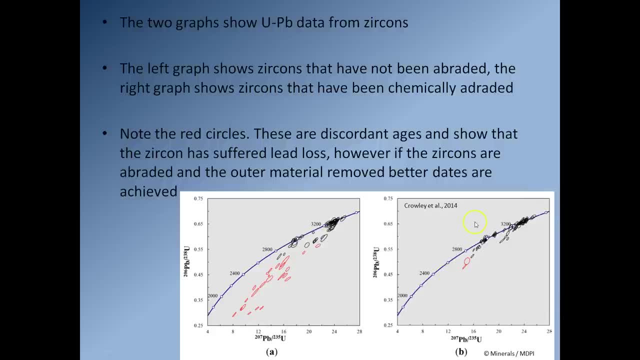 that could have suffered loss or leakage. And so what you can see is that when you remove these outer layers, when you abrade them away, you can see that the data moves towards the line of concordia. so it's good data. 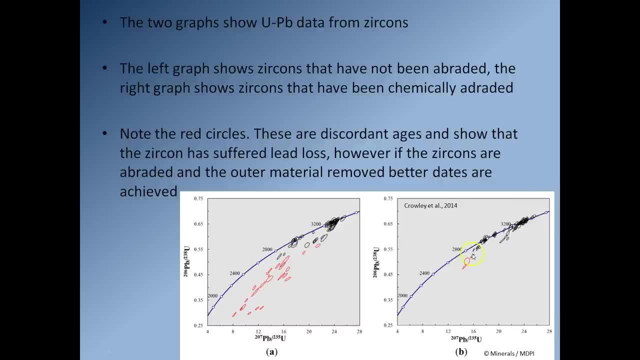 And we only get a few outlying points out here. These are points which are bad data. We would call them discordant and we would remove them from our analysis. We wouldn't count them when we're doing our dating. So by abrading the crystals. 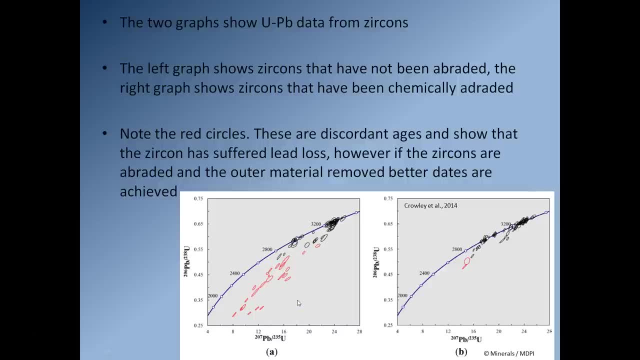 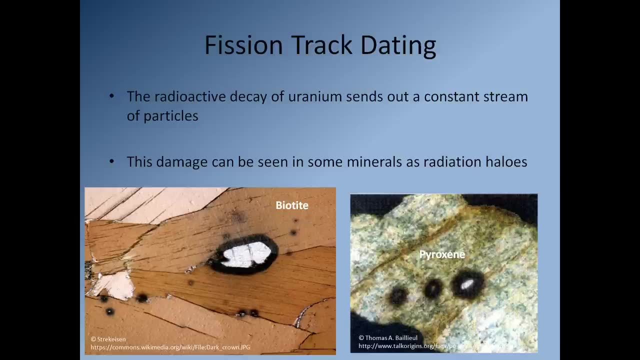 we get rid of this problem relatively easily. OK, so it's been another 20 minutes, so this is a good time once again to pause the video, get up, have a walk around, have a drink of water and then come back when you've had a bit of time to relax. 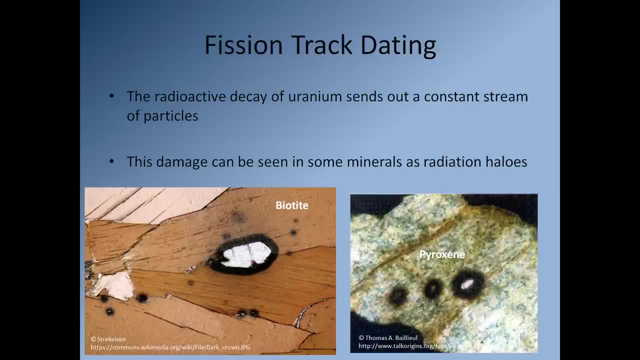 OK, so here we go. We're on the last few slides, so let's just keep going, and hopefully we'll make it to the end of the presentation relatively soon. So today's code word, today's code word, is going to be: 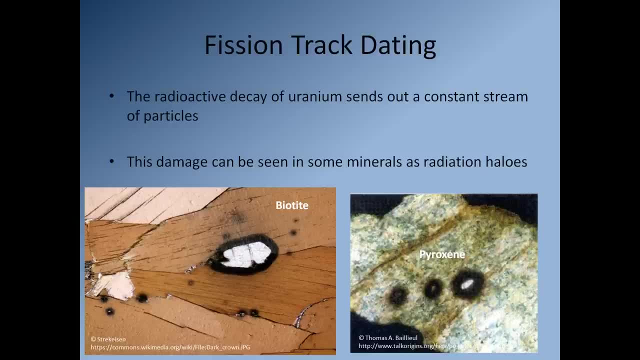 let me see, I'm looking around my games room now. Today's code word is going to be minion, as in the yellow thing from Despicable Me. OK, so that's minion M-I-N-I-O-N. So fish and track dating uses essentially. 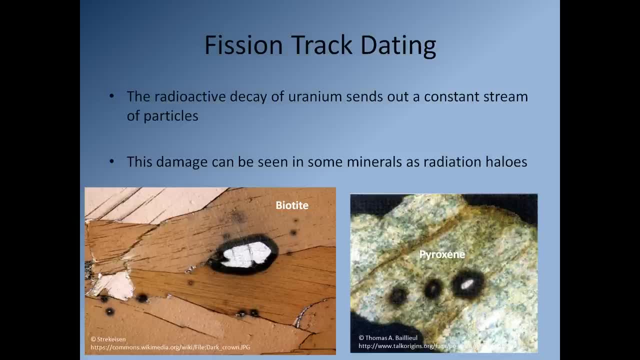 the damage caused by radioactive decay. So I'm sure at some point you guys have either used or you've seen a Geiger counter. So a Geiger counter makes that clicking sound. So it's clicking every time a radioactive particle hits the detector. 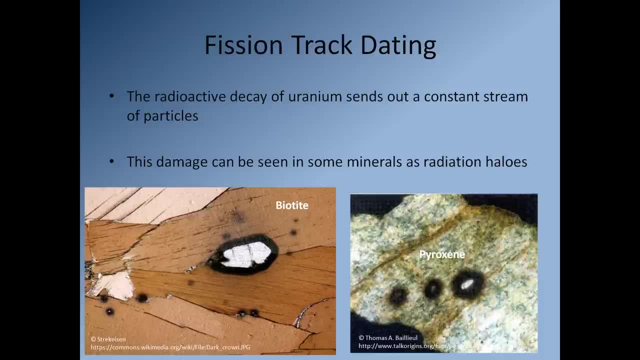 Obviously, the closer you come to a radioactive source, the more particles hit the detector and the faster the particles hit the detector and the faster that clicking noise becomes. So these particles that are being thrown out during radioactive decay go flying everywhere. So in some cases, as these particles fly out of the mineral, 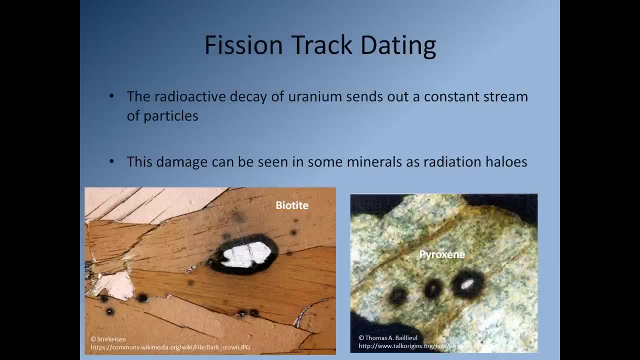 they will hit other minerals that surround them and they'll damage those minerals And we can use that damage to help date a rock. So here's a couple of examples. So here's a crystal of biotite, this brown crystal here, And this is a crystal of pyroxene. 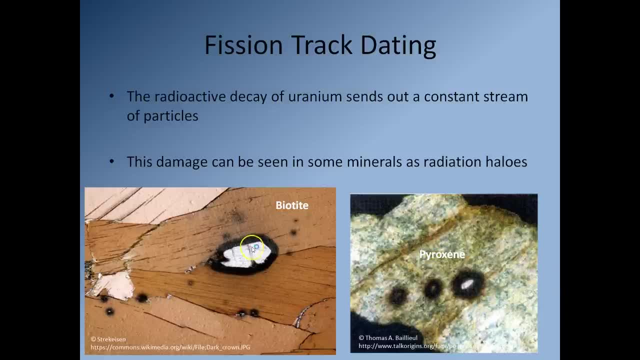 this kind of mottled-looking crystal here. Now you can see, within these two crystals, we have this crystal here, this very, very colourless crystal, and there's a very colourless crystal here. So these are crystals of zircon. 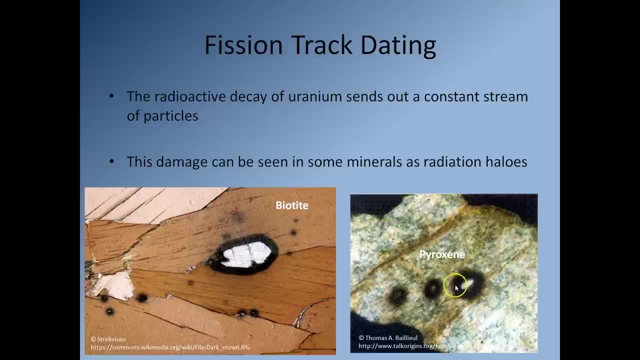 And you can see around these crystals of zircon we have these black lines. These are referred to as halos, And you can see there's another crystal of zircon here, another halo. All these black dots here essentially represent little crystals of zircon. 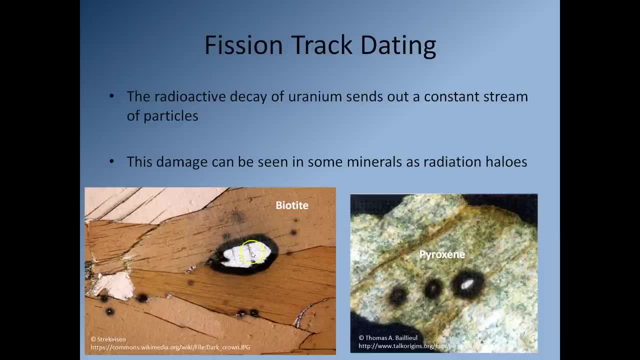 and the black areas represent the halos around them. So what's causing the halos? Well, the halos are being produced by the decay of uranium within the zircon crystal. So, as the uranium decays inside the zircon crystal, alpha particles, that's you know. 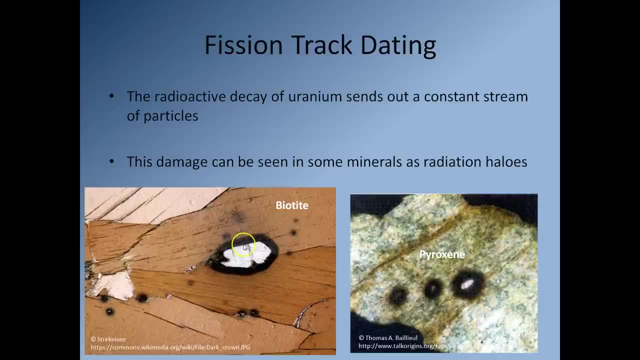 these two-proton, two-neutron particles and electrons from beta decay are being thrown out and they're hitting the surrounding biotite crystal. And as they hit the surrounding biotite crystal, they damage the crystal lattice and so they make the mineral turn black. 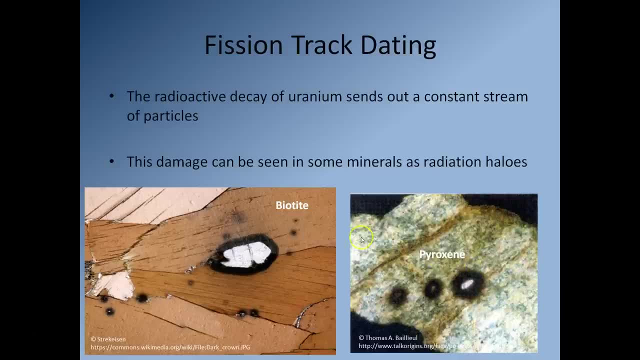 Same thing's happening in the pyroxene right here. So these radiation halos reflect damage caused by the particles coming out of the zircon hitting the surrounding crystals. Now damage will not only be occurring to the surrounding minerals, but it will also be occurring within the crystal. 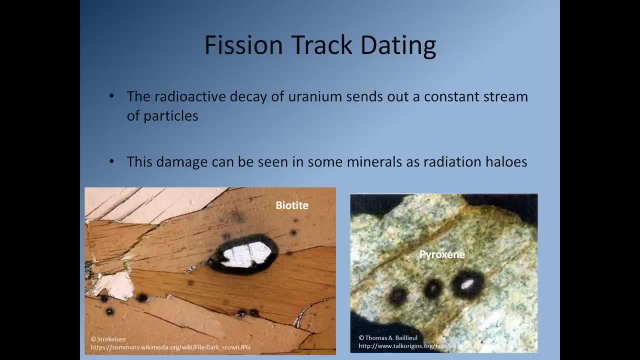 that has the radioactive isotope in it. So we can look for the damage within these crystals and we can count the amount of damage, and that will help us to date the crystal. So how does it work? Well, the preferred mineral for this method. 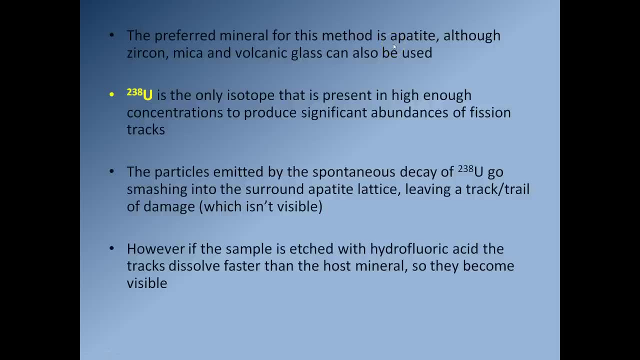 is the mineral apatite, so that's calcium phosphate. It's the stuff your bones are made up from. So, although we can also use zircon microcrystals like biotite or muscovite or volcanic glass like obsidian, 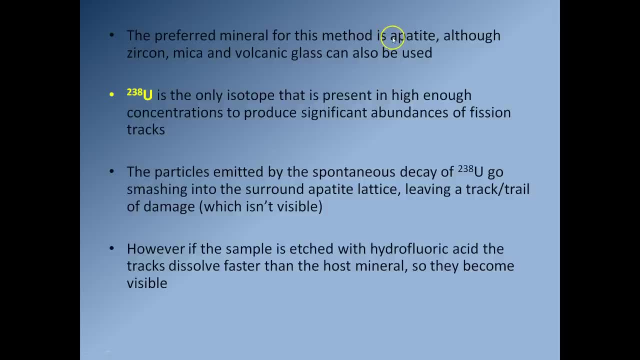 but most of the time we use apatite. So the isotope we use is uranium-238, because it's the only radioactive isotope that's present in apatite in very, very large quantities. So what happens is as uranium-238 decays, 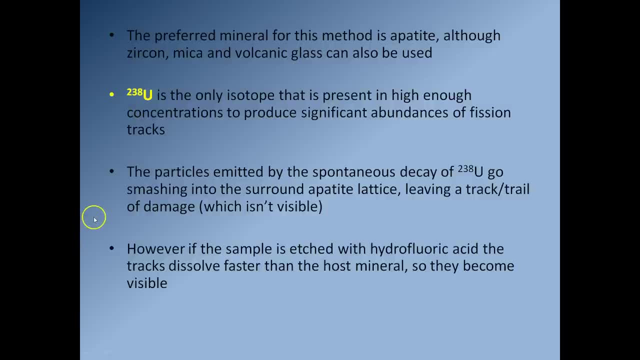 it kicks out particles and those particles go flying through the apatite crystal and sometimes they will hit other atoms in the apatite crystal and they'll damage the crystal lattice. And we can come along later and we can look at that damage in the crystal lattice. 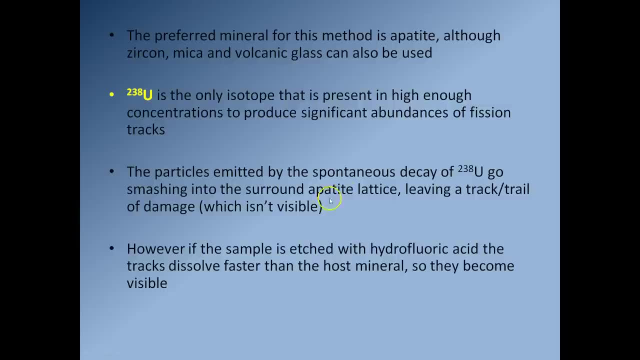 and we can use it to date the mineral. Now the damage itself isn't visible. We can't see it when we look at the crystal down the microscope. We have to do what's called etching. So what we'll do is we'll take the crystal of apatite. 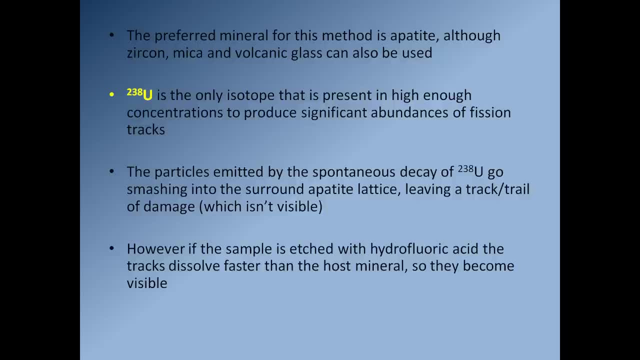 and we'll dunk it in very, very strong acid for a very, very short period of time. Typically, we use an acid called hydrofluoric acid, And hydrofluoric acid will dissolve the areas of damage faster than it will dissolve the areas of the crystal. 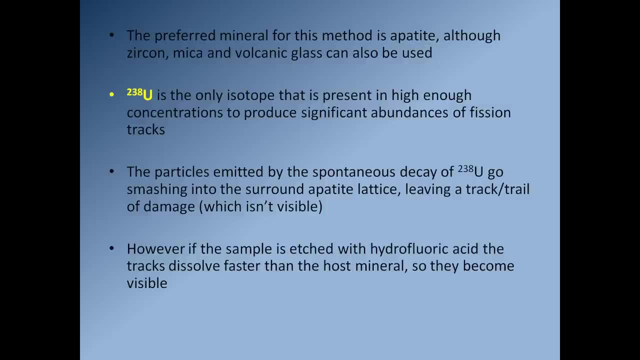 that are not damaged, And so we dunk it in very, very quickly. It will essentially dissolve the damaged areas faster than the damaged areas and the undamaged areas, And so when we look at the crystal down the microscope, we can count the damaged areas. 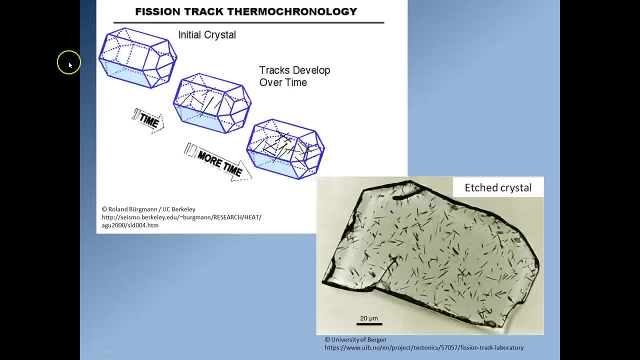 So how does it work? So this is the basic idea. So here's our crystal of apatite, And when it starts off, obviously there's no damage, And over time the amount of uranium decaying is increasing, And so that means there's more uranium decays. 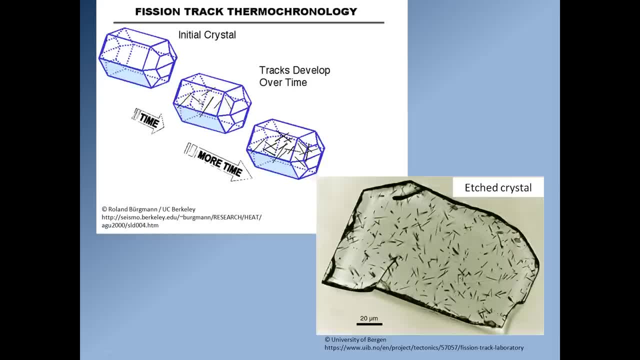 more alpha particles and beta particles have been produced. They've been flying through the crystal, hitting the crystal lattice, And so they've been causing more and more damage. So over time we get more and more uranium decay. We get more and more fission tracks forming. 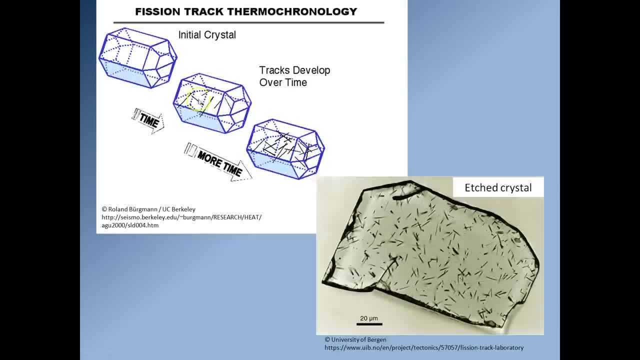 Okay, So that's the general idea. So as time goes by, as time increases, the amount of fission tracks increases. Now, the rate at which these fission tracks form is constant. So once again, it's like the second hand in your watch. 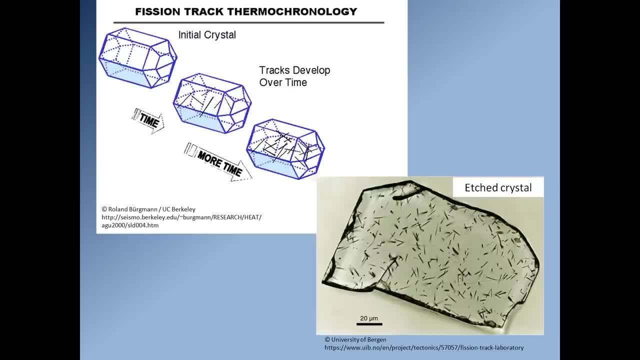 It happens. you know, click, click, click, click, click. It's exactly the same thing with the fission tracks. So let's say you know one fission track forms every day, If you have seven fission tracks when you analyze your crystal. 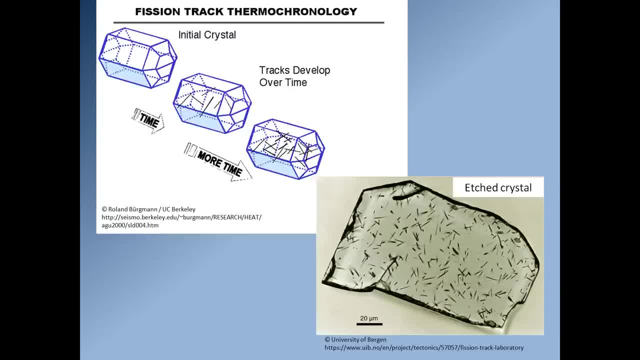 that means your crystal is seven days old. If you have 2,000 fission tracks, that means your crystal is 2,000 days old, And so we can see it in this crystal here. So this is actually an etched crystal. 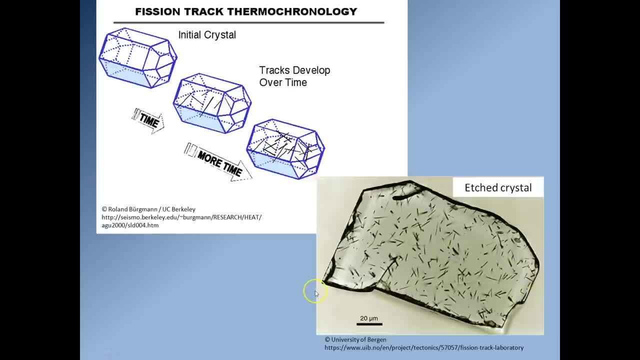 Okay, So this is a crystal of apatite that's been dunked in acid for a few seconds to etch it, And each one of these black lines represents a fission track, And so all you have to do is you look at your crystal. 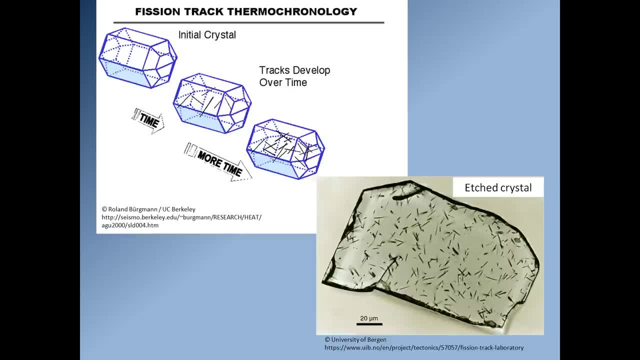 down the microscope and you count all the fission tracks And that's it. And because you know the fission tracks are forming at a constant rate, once you have the total number of fission tracks for the crystal, you can simply multiply the rate of formation. 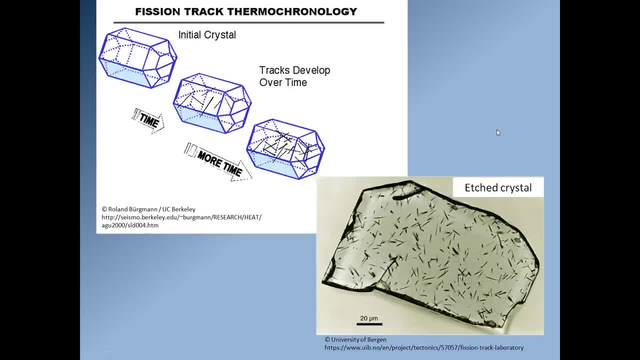 by the number of fission tracks, and it will give you an age for that crystal. Done Very, very simple. It's a very straightforward method. The one thing is, of course, is that you have to count all the fission tracks. 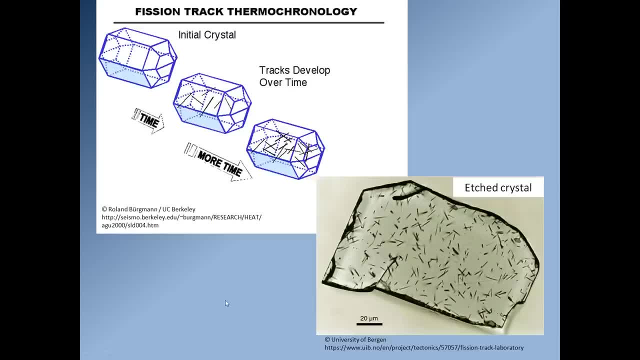 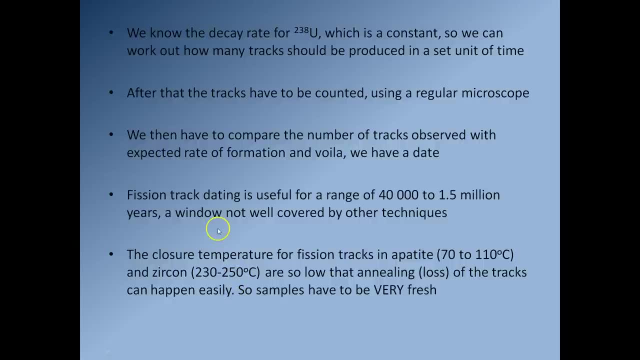 And that means you have to sit in a dark room for hours. So that's the one thing, So that's the one drawback for this particular method. So the great thing about fission track dating is that it covers an age range between 40,000 and 1.5 million years. 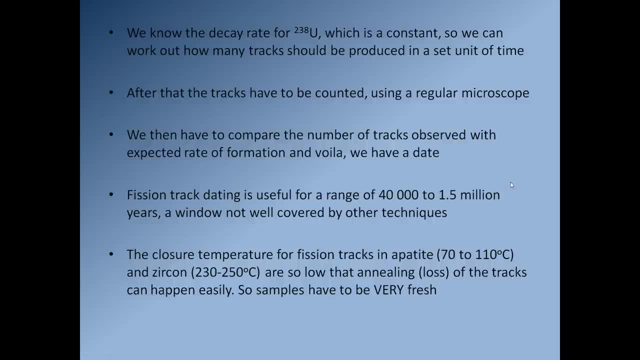 And that's an age range for rocks that's not particularly well covered by other dating techniques. The one problem, though, is this: The closure temperature for apatite for fission tracks is 70 to 110 Celsius, So it's very, very easy to take the crystal back up above that temperature. 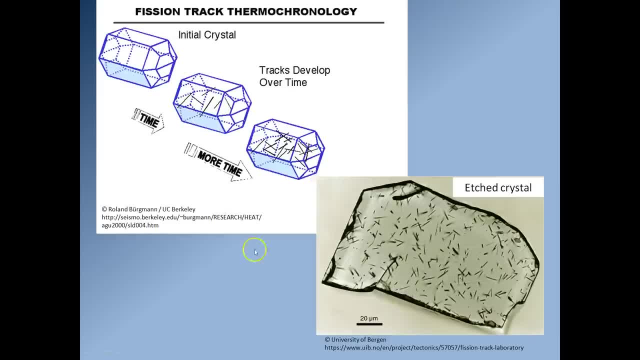 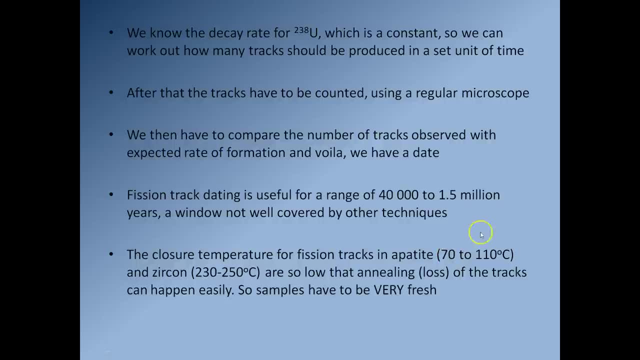 at which point you will lose all or most of your fission tracks. So, to be clear, in terms of geology, taking something to 70 to 110 Celsius is easy. You can sneeze in geology and create those kind of temperatures. 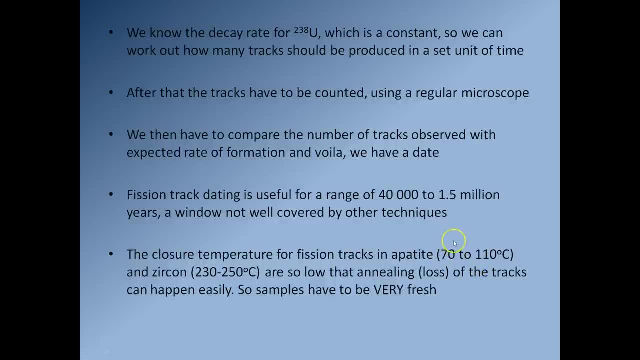 Hell. it's easy to do in your kitchen. You can easily take a crystal of apatite to 70 Celsius by putting it in a pan and heating it up to 70 Celsius, you know, without any effort. So you have to be very, very careful. 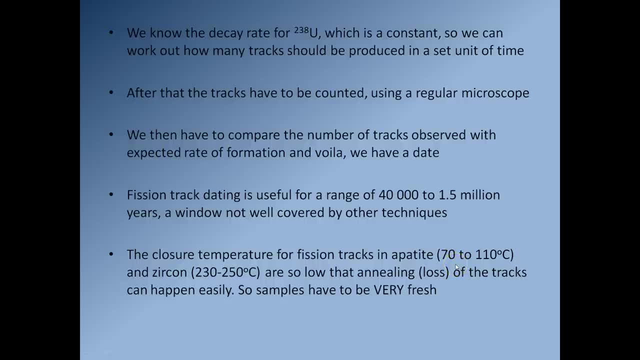 that the material you're using is very, very fresh and hasn't been altered. In the case of zircon, once again, the closure temperature is very, very low. for fission tracks, It's between 230 and 250 Celsius. Once again, in terms of geology, 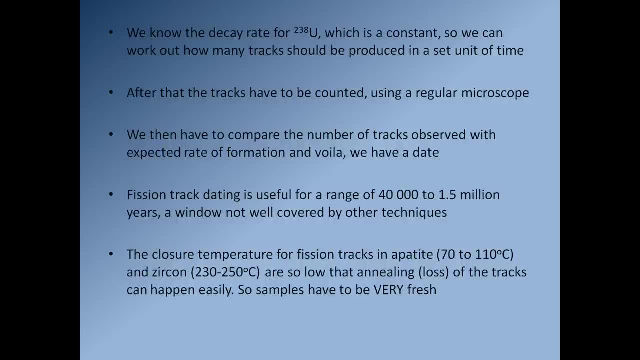 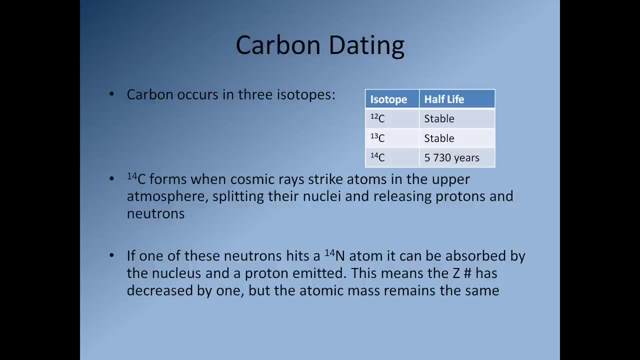 it's super easy to reach those temperatures. So the final method of dating we're going to think about is carbon dating. So carbon dating uses Well. carbon, should I say, occurs in one of three possible isotopes: There's carbon-12, carbon-13, and carbon-14.. 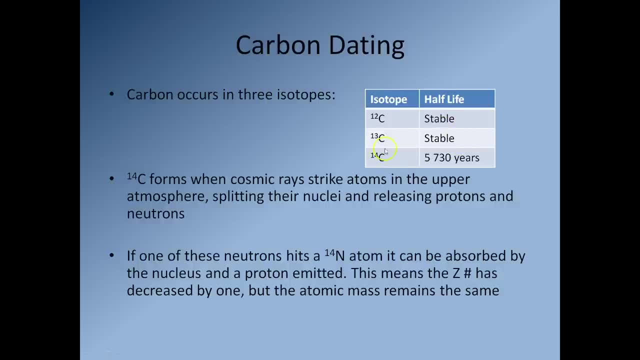 Now, carbon-12 and carbon-13 are stable. Carbon-14,, on the other hand, is unstable and has a half-life of 5,730 years. So how does carbon-14 form? Well, carbon-14 forms when a cosmic ray. 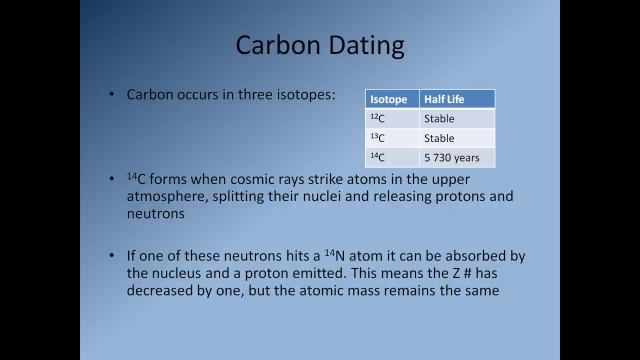 that comes from the sun hits an atom in the upper atmosphere. So when it hits one of these atoms in the upper atmosphere, it can be an atom of anything, Let's say oxygen. So this cosmic ray comes flying in, hits the Earth's atmosphere. 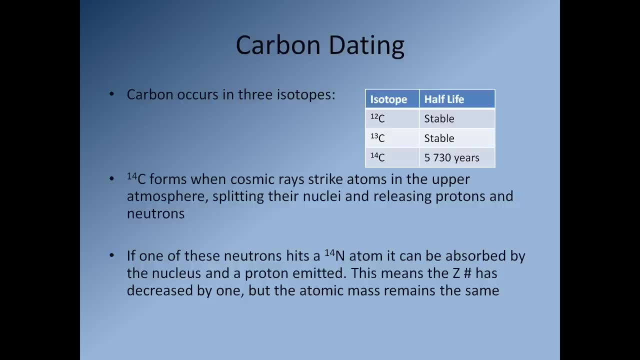 it hits an atom of oxygen in the Earth's atmosphere and it obliterates that atom of oxygen. It sends protons and neutrons flying in all directions, So it's blown up the atom of oxygen. So if one of these neutrons 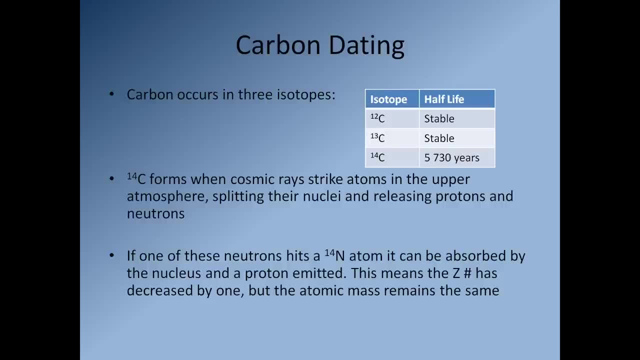 that's produced by this explosion hits a nitrogen-14 isotope, it will be absorbed by the nucleus And once it's absorbed by the nucleus, it will have to get rid of a proton to achieve balance. OK, So what happens is that means you've changed the proton number. 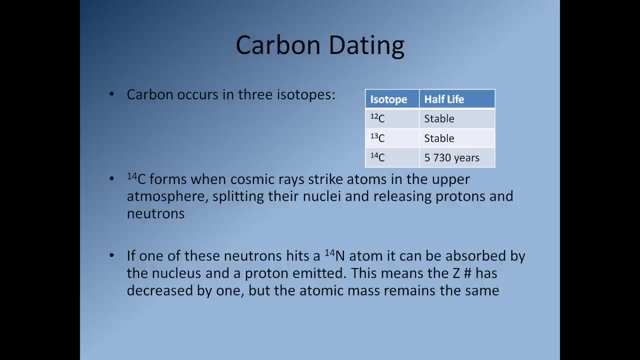 by decreasing it by one. so your atom is, your isotope is no longer, is no longer nitrogen, It's now turned into carbon. Now the atomic mass has remained the same, because you've gained a proton and you've kicked out a neutron. 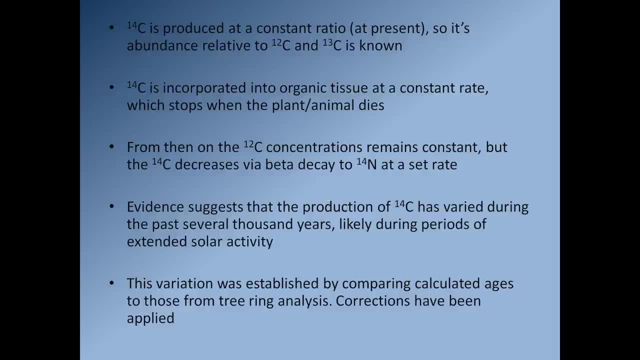 So carbon-14 is produced at a constant rate, and we know what that rate is. So Well, we know what the rate of production is relative to carbon-12 and carbon-13.. So carbon-14 gets incorporated into organic tissue. 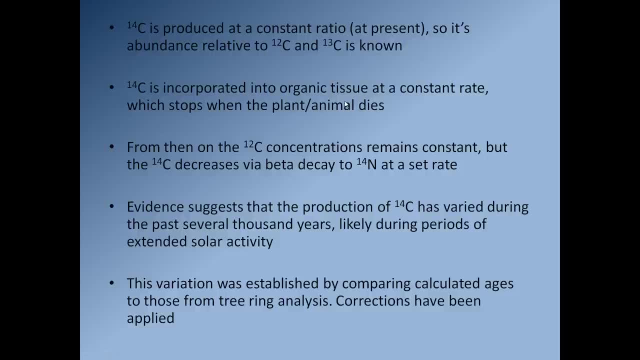 at a constant rate. So plants, when they photosynthesize, will use some carbon-14 as they take in carbon dioxide from the atmosphere. That carbon-14 then gets incorporated into the organic tissue of the plant as the plant's growing. A cow comes along, eats the plant. 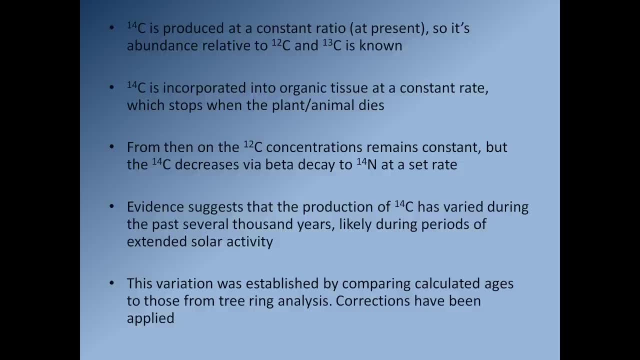 That carbon-14 then gets included into the organic tissue of the cow. We come along, eat that cow. We then get the carbon-14 from the cow and that gets incorporated into our organic tissue, And so carbon-14 is constantly being incorporated. 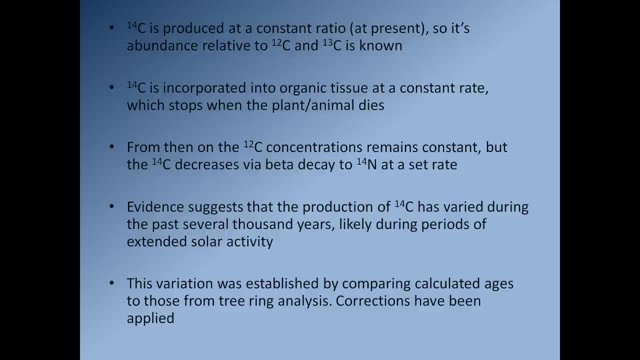 into your organic tissue as long as you're eating. So what we can then do is So, from then on, the carbon-12 concentration in your body remains constant, But the amount of carbon-14 will decrease the second you stop eating. Okay. 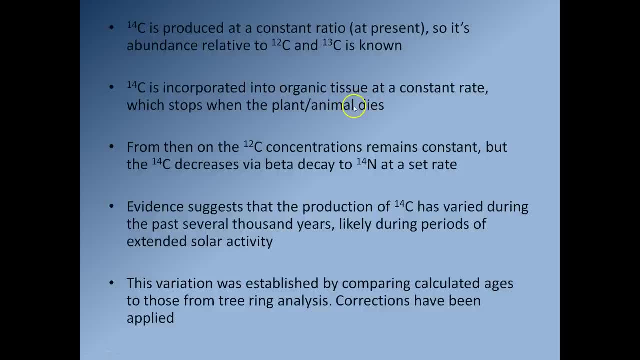 So obviously, you stop eating, unfortunately, when you die. So the amount of carbon-12 in your body doesn't change because it's stable. The amount of carbon-14,, on the other hand, will begin to drop, will begin to decrease. 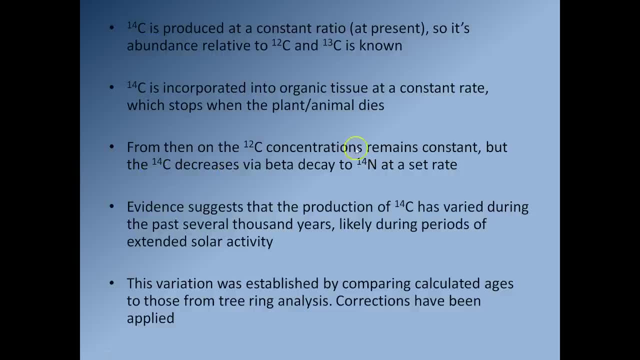 because the carbon-14 is naturally unstable and it will break down to form nitrogen-14 instead, And it does that at a set rate. So we know the amount of carbon-14 that will have been in your body when you died, And so all we have to do is measure. 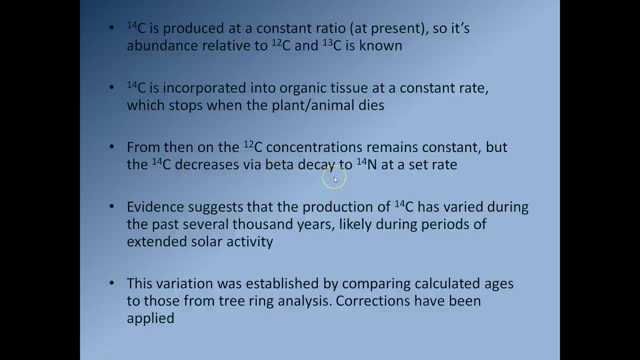 the amount of carbon-14 in your body later on, And so we can look at the change in the amount of carbon-14, and we can use that to calculate an age from that value. So evidence suggests that the production of carbon-14 has varied a bit. 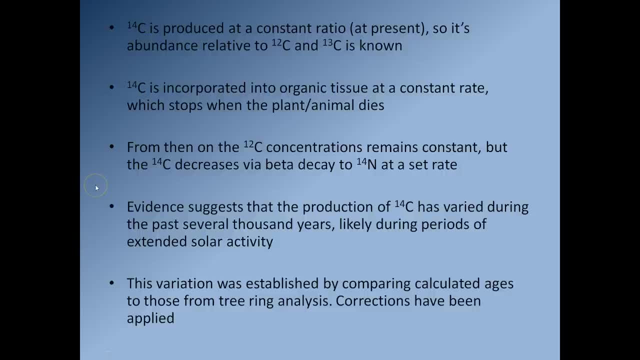 during the past several thousand years, likely during periods of extended solar activity, when the sun was very, very active. So that does have to be taken into account, because the more active the sun is, the more carbon-14 would be produced in the atmosphere and therefore 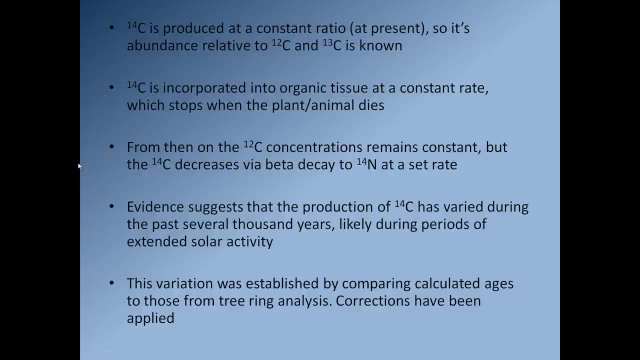 the more carbon-14 there would be in organic tissue from that time period. So we can take that into account and we can correct for it in our calculations. So this variation, this indication that carbon-14 rates varied somewhat, was established by comparing calculated ages. 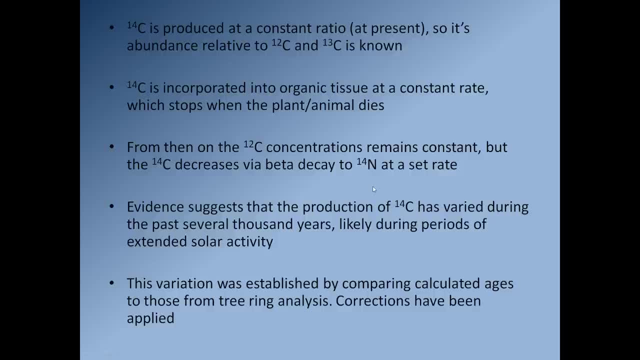 to those from tree rings. So we analyzed organic material from tree rings and we compared it to the tree ring date and we managed to work out that in some cases the tree ring date and the carbon-14 date did not agree, And that would typically mean that 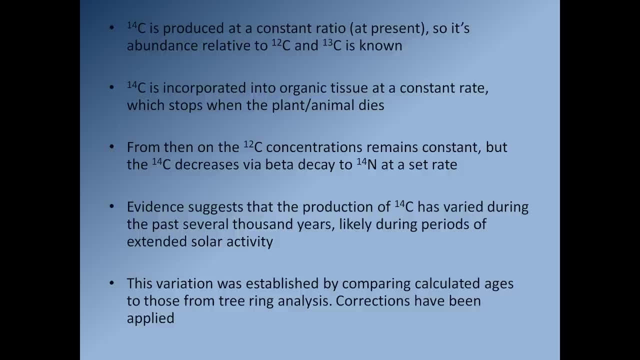 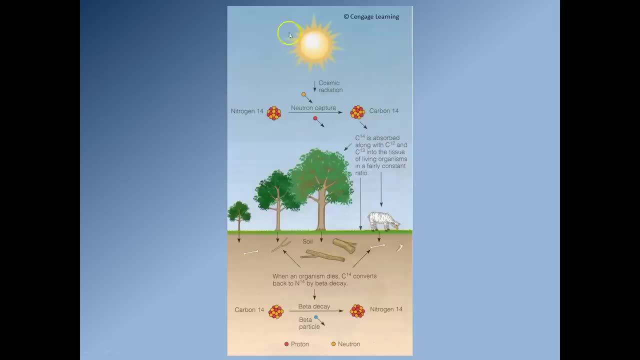 more carbon-14 was being produced at that time, and so once we know that we can correct for it in our calculations. So this diagram here kind of summarizes the basic idea. The sun produces cosmic rays. Cosmic rays strike some unknown atom in the atmosphere, destroying it. 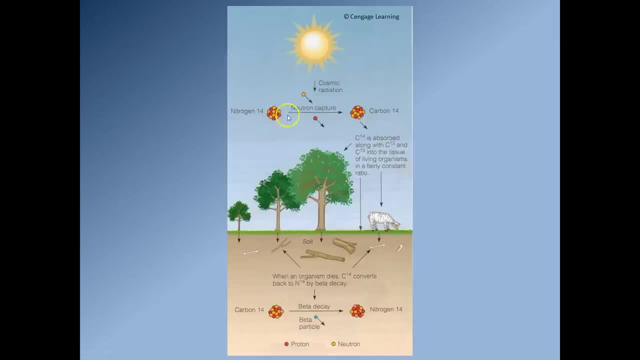 sending out a neutron that flies and hits a nitrogen-14 atom. When that neutron hits a nitrogen-14 atom, to make itself stable it has to kick out a proton. That means your nitrogen-14 has now lost a proton, so now it's carbon-14. 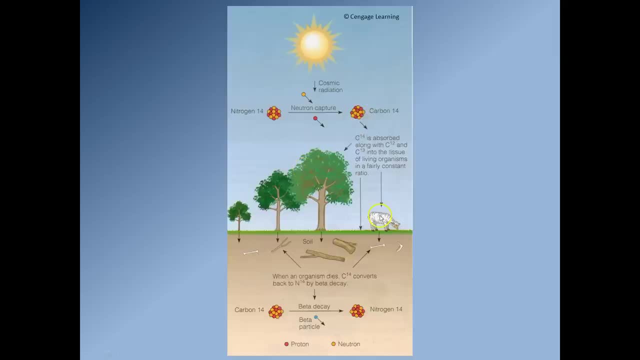 The carbon-14 gets incorporated into plants. Animals eat the plants, We eat the animals And the amount of carbon-14 is being constantly replenished in your body every time you eat. We know the amount of carbon-14 in the organic tissue. 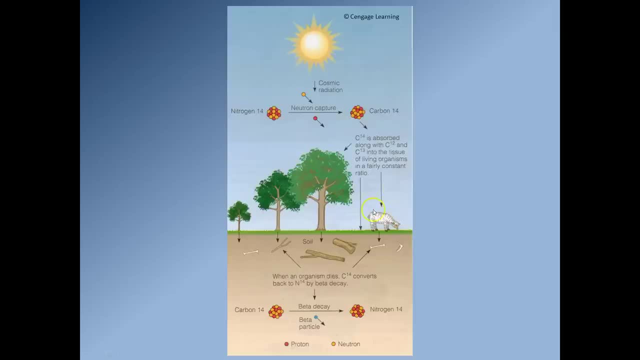 The amount of carbon-14 stops being replenished when the organism dies, And so, after it dies, the amount of carbon-14 steadily drops, And so we can calculate the age of the organic material using the amount of carbon-14 present. And so that's why carbon dating. 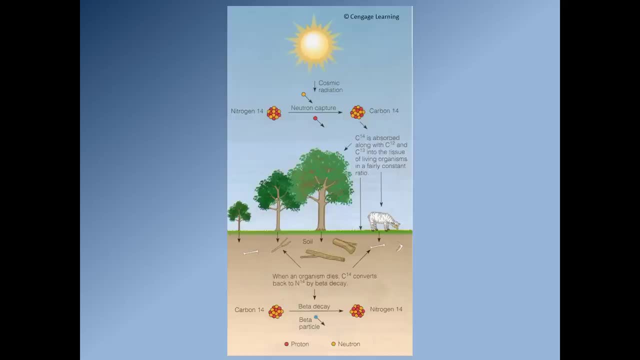 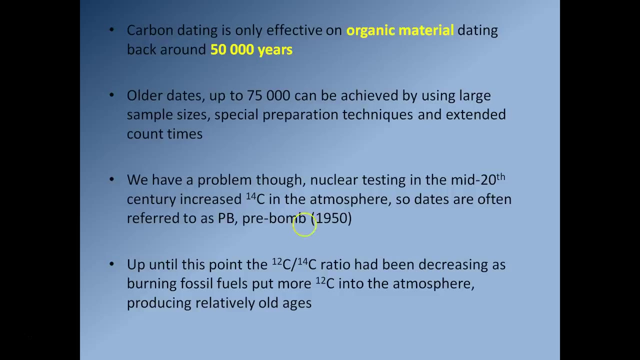 is good for dating stuff like organic remains, be it leather or actual bone or anything like that. Now, the one problem is that carbon dating is only good for material that's up to 50,000 years old, So you can't really use it for rocks. 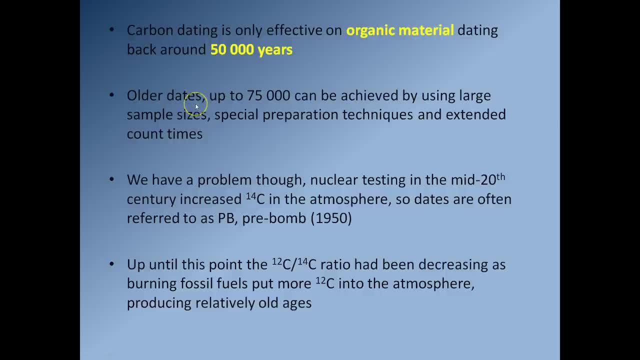 and you can't use it for very, very old stuff. You can date older material up to 75,000 years, but you need a very, very large sample size and you need to use very, very special techniques and extended count times, so it's more expensive. 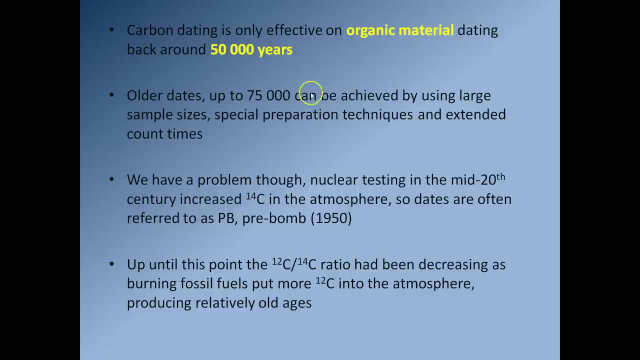 So carbon dating can only date stuff that's up to 75,000 years old at the extreme maximum. Typically it can only date stuff that's 50,000 years old. So another problem is that nuclear testing in the mid to early 20th century 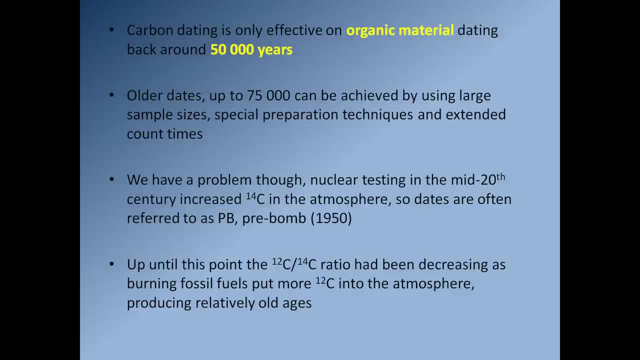 has affected the amount of carbon-14 in the atmosphere. So when we blew up all these nuclear bombs, well, that increased the amount of carbon-14 in the atmosphere and so that went and affected the amount of carbon-14 that was going into. 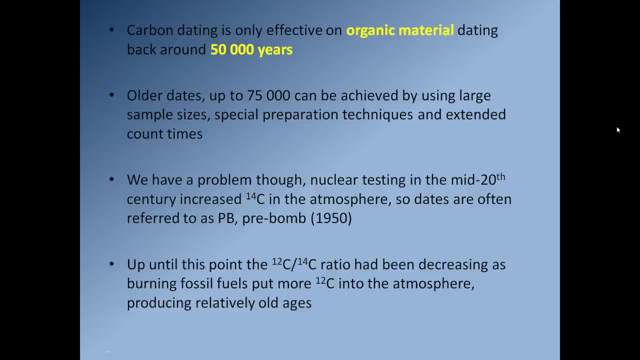 organic tissue And so that's obviously had an effect on carbon-14 dating. So we can correct for that. So if we are dating something that happened before we started exploding nuclear weapons, it's given a date that's called PB or pre-bomb, and that's essentially 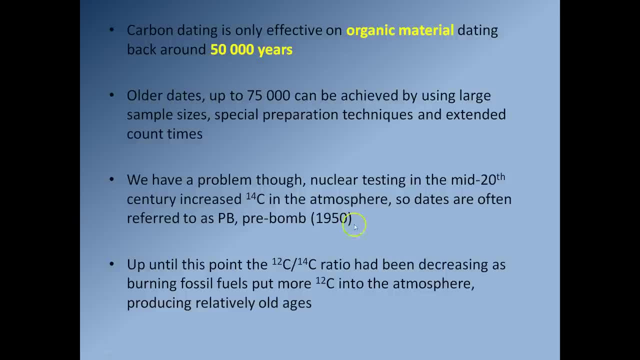 anything before 1950. Anything that's dated from after 1950, essentially, if we try to use carbon dating to date, it essentially we have to take into account the amount of carbon, the extra carbon-14 that was produced by these nuclear. 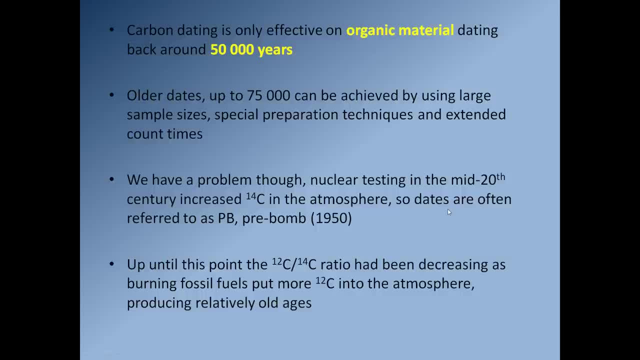 explosions, And so we'll have to apply a correction for that. I should also point out that the burning of fossil fuels is also affecting the amount of carbon-12 and carbon-14 in the atmosphere, because we are burning organic material in the form of coal. 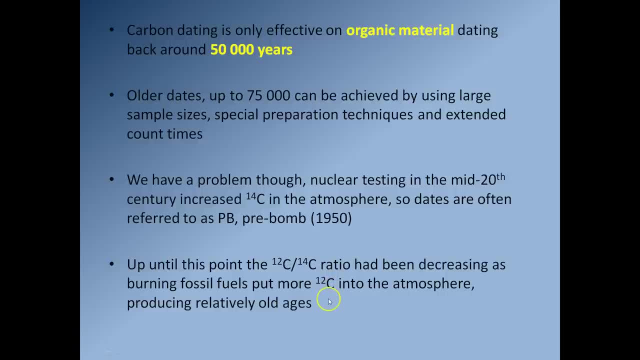 and oil and gas, and that's releasing carbon-12 back into the atmosphere and so that's affecting the carbon-12 carbon-14 ratio And so that also has a very small effect on our dating. so once again, we have to apply a correction for that. 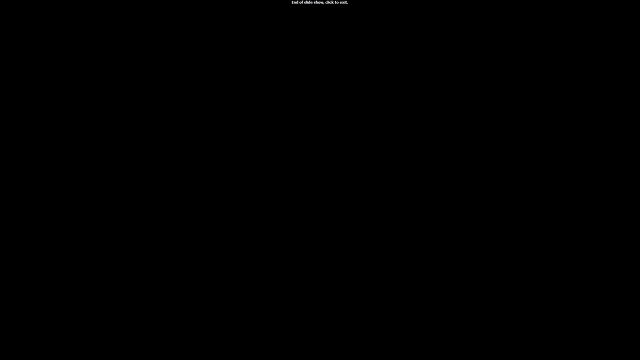 Okay, so that was the end of the geologic timescale presentation. Obviously, please make sure you write down the code word. the code word was, of course, MINION M-I-N-I-O-N. so think of these small yellow guys from the Despicable Me movies.